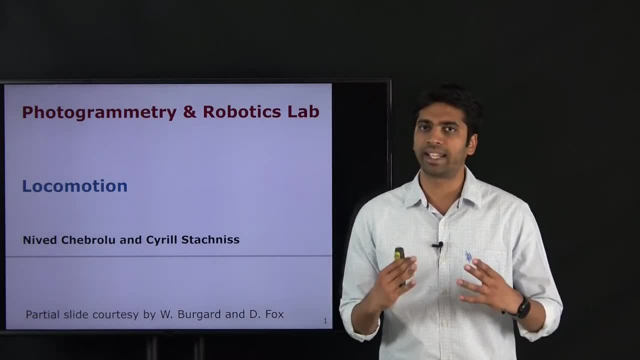 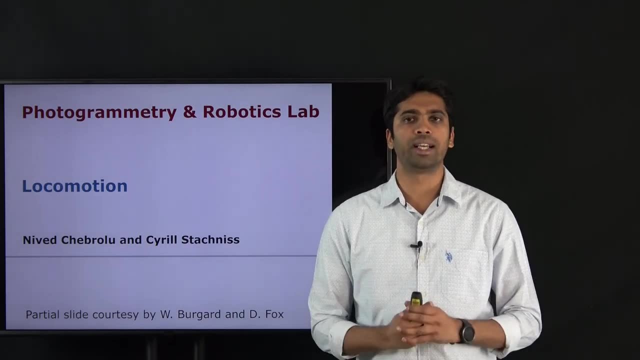 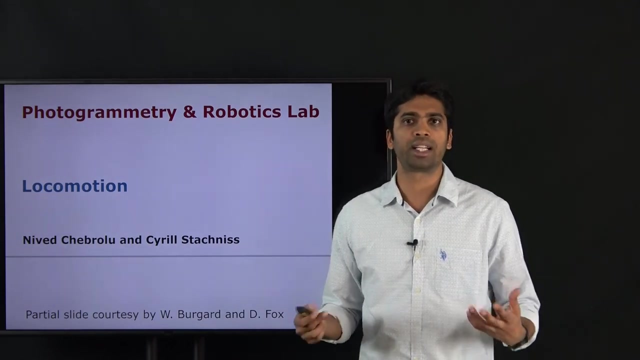 So in this lecture, we will primarily focus our attention to mobile systems that are wheeled. So they are equipped with wheels, which let them move around in their environment. A couple of reasons to do this. One: they're one of the most common kind of platforms that are available around us. 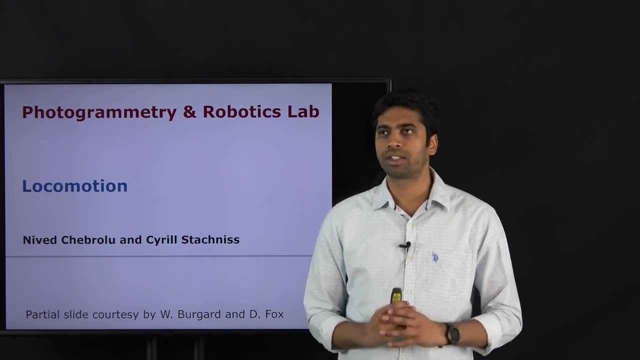 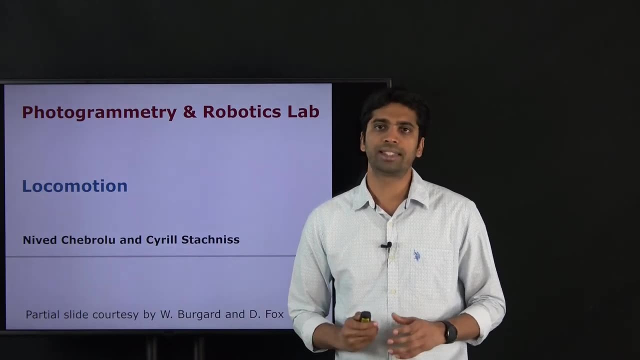 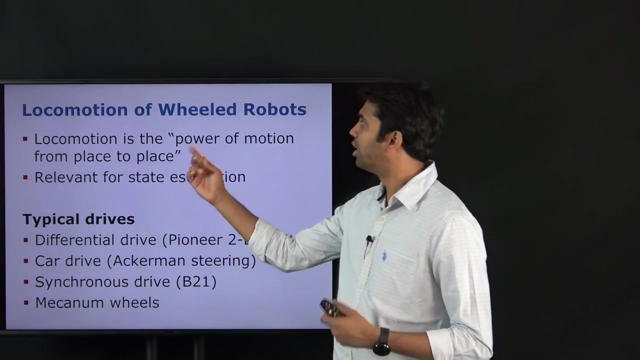 and therefore very useful To know how they work. And two because the analysis is quite straightforward, which lets us understand the principles in a rather simple manner. So let's get started. What does locomotion really mean? So the definition is the power of motion from. 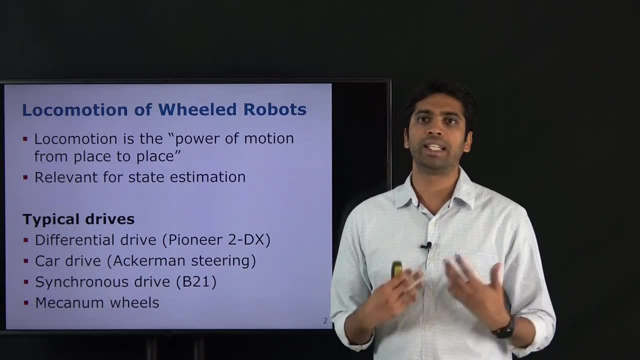 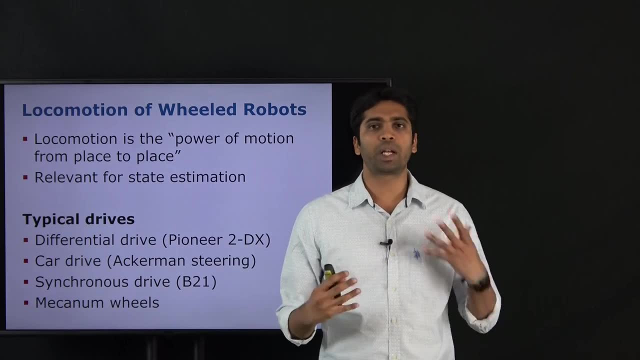 place to place. Essentially, what locomotion deals with is to understand how to move from point A to point B in your environment, And this is done quite at a lower level, in the sense that we don't really understand at this point how our environment. 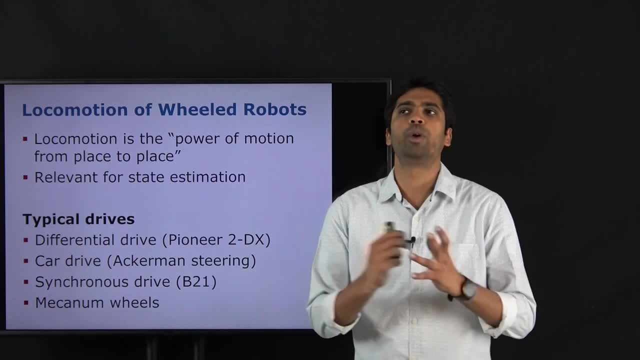 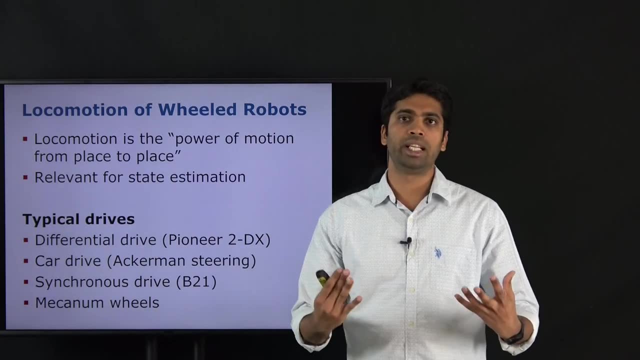 looks like or anything. We don't have a map of the environment or we don't have a plan which we want to particularly follow. It's more at a level as to understand: when we provide certain inputs to our mobile robotic system, how does it respond? How does it actually move in its 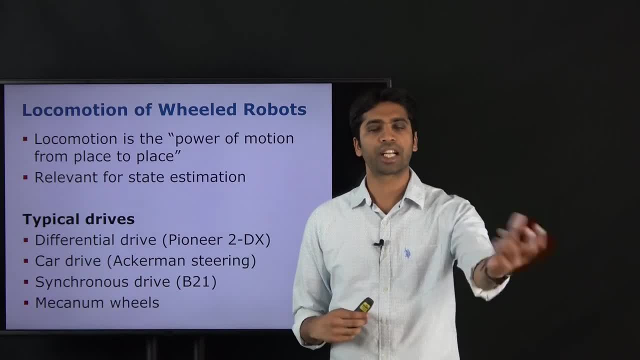 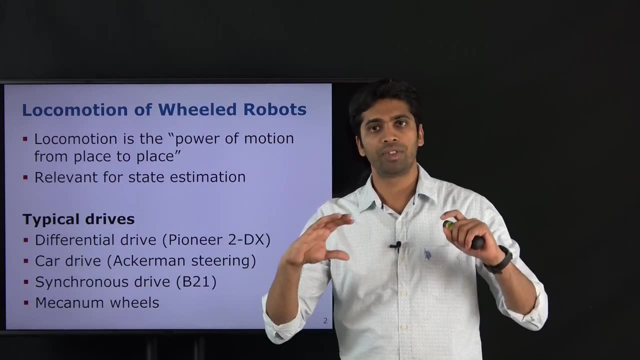 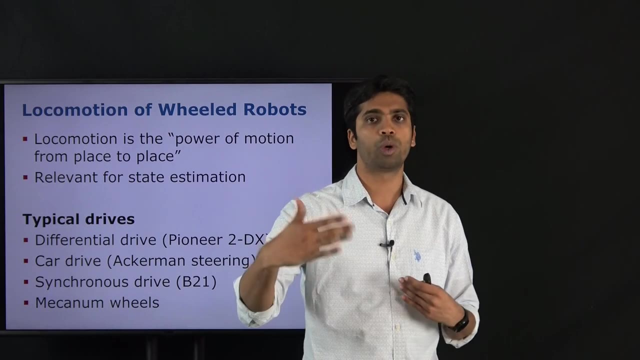 environment, And this information is actually relevant for state estimation problems. So if we understand how the robot reacts to certain input commands, then we kind of have an estimate of where the robot is over a period of time. This information, so this locomotion information, 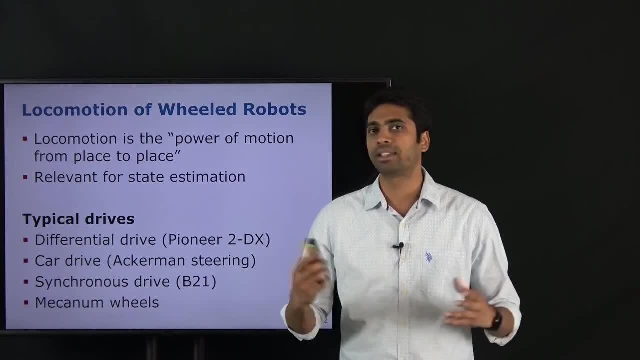 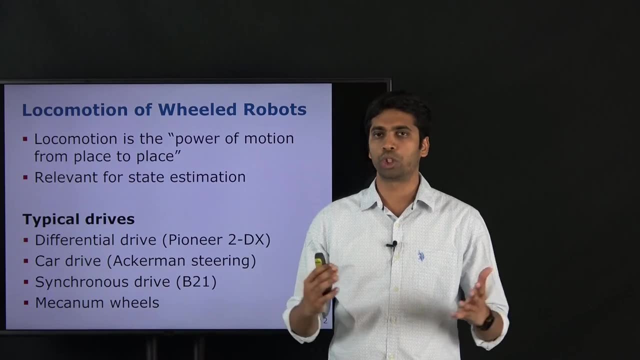 can then be fused with information coming from other sensors, some other external sensors. This could be, say, a GPS sensor if you're outside, Or these could be a laser scanner which gives us some motion of how we move. And so these are. 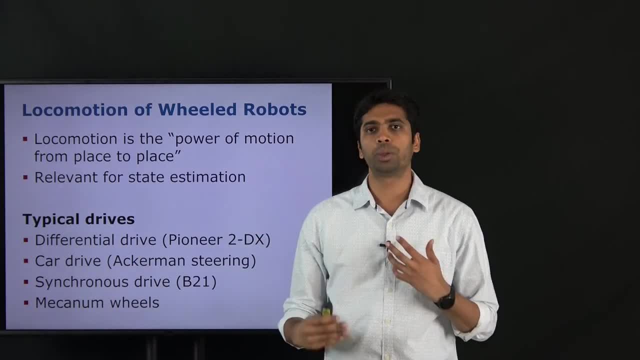 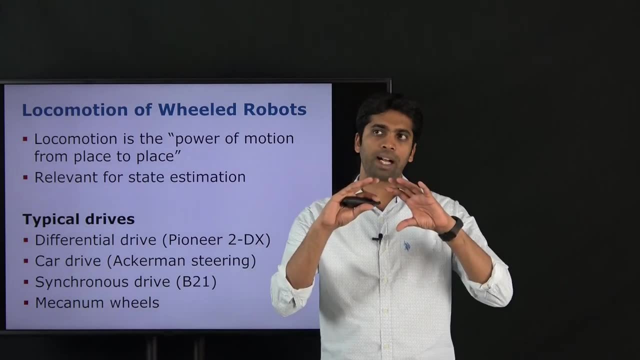 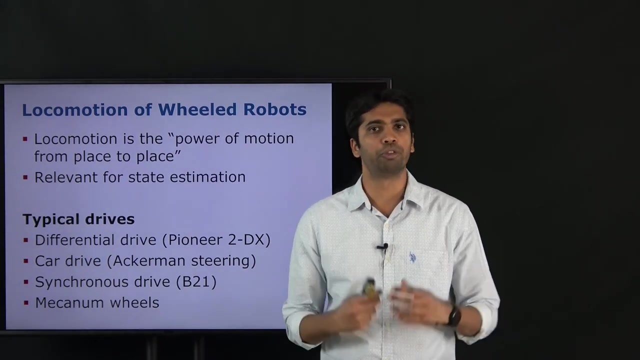 these information can then be fused together in order to estimate the pose of our system. So these are some techniques that we'll see in other parts of the course, But basically the idea of locomotion fits in there in order to have an estimate of how the platform has moved. 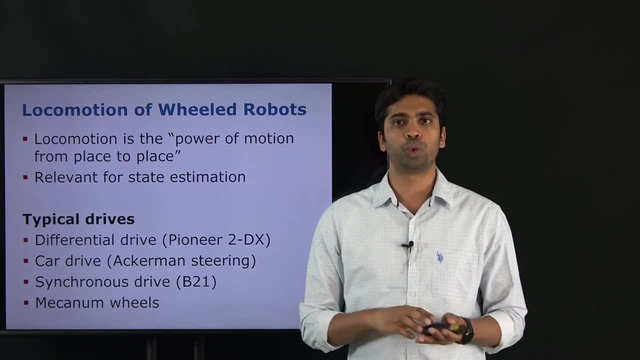 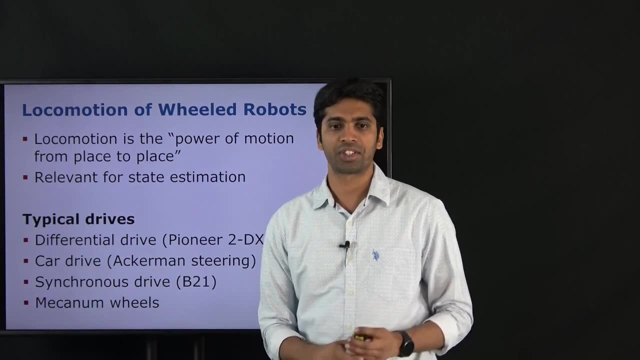 So in this lecture, since we limit ourselves to wheeled robots, there are three or four types of wheeled robots which are quite common and they are listed here. They're also called as drives, So we'll spend quite a bit of time understanding what is called as the differential. 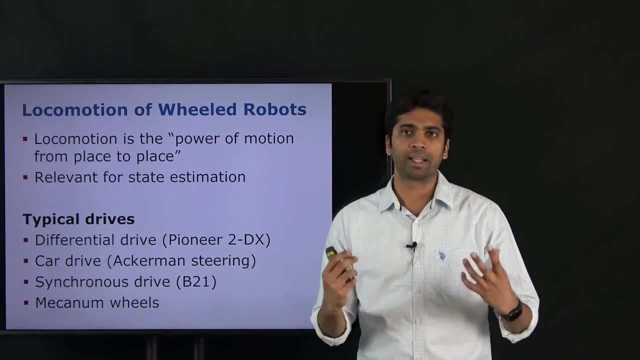 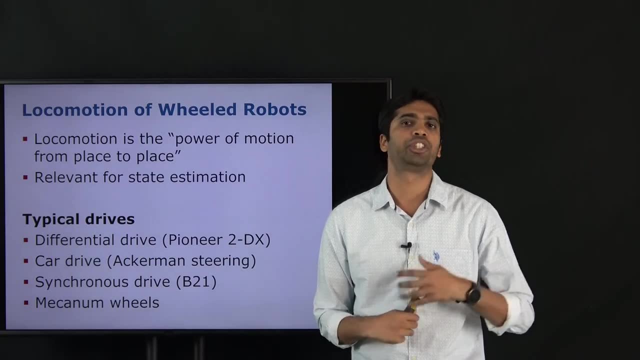 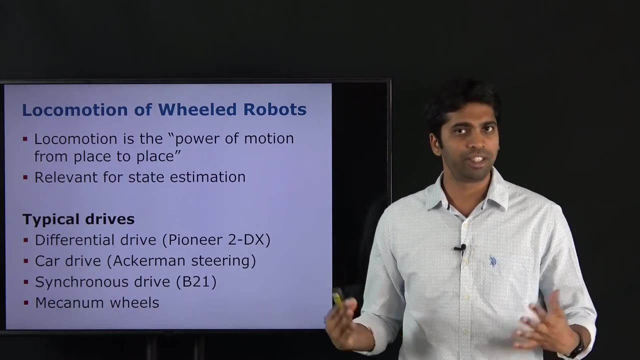 drive. Essentially, these are robots- typically indoor robots- which have a couple of wheels on them, And each of these wheels has a motor attached to them which rotates these motors and lets them move around in their environment. We'll see in detail how the motion is evolved and 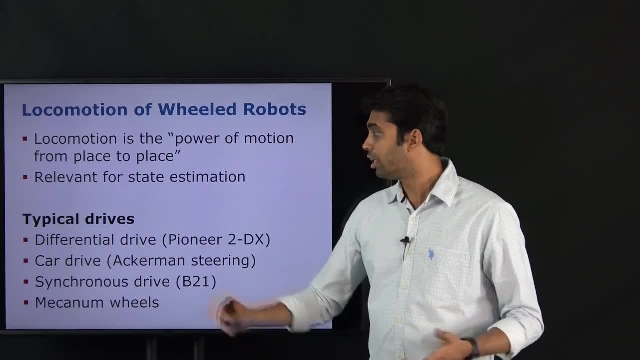 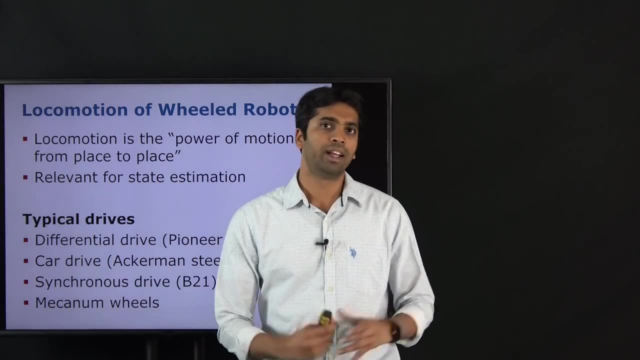 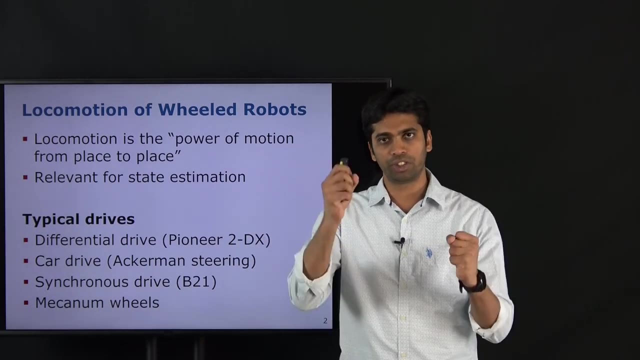 how we can control such Such robots. The other common kind of robot or drive that we have all seen is the Ackermann drive or the car drive. Essentially, in these vehicles you have the back wheels, which are fixed, and we have front wheels, which can be then steered, And in this way, 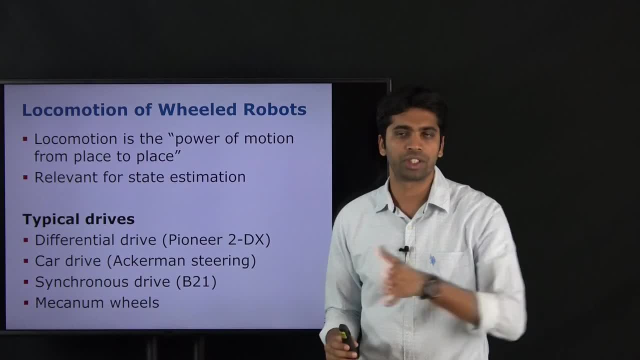 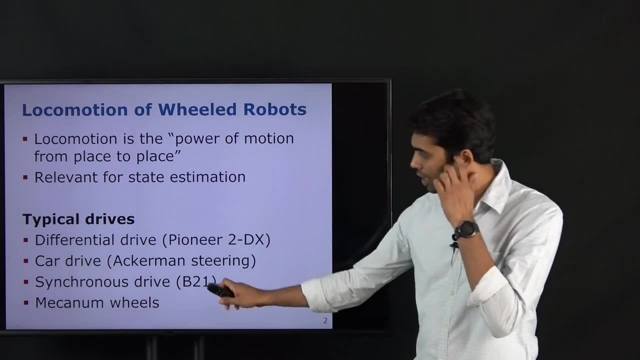 we are able to track a certain path or a certain circular arc, for example. And there are these two other drives which are quite interesting. One is called as the kernel drive and another which is based on these Mecanum wheels. 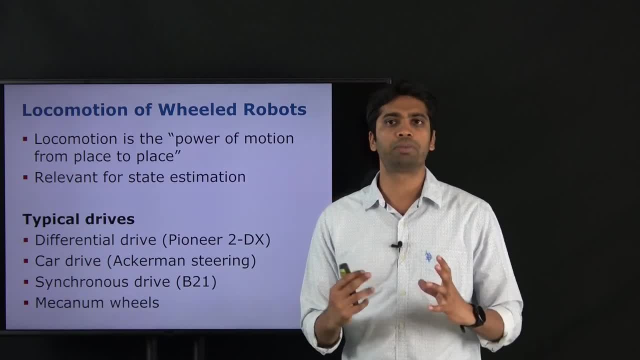 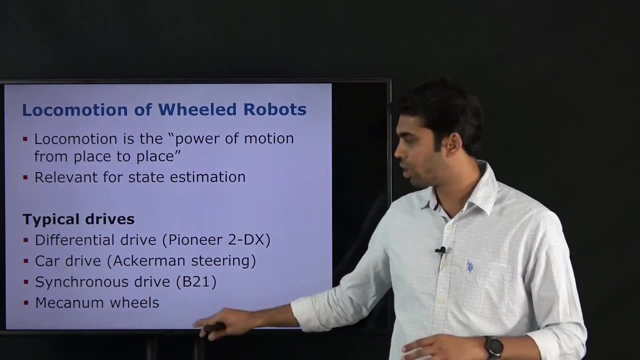 which have, which become quite interesting in confined spaces. If you have really limited space to make a maneuver, these kinds of drives really help us out there. So we'll also look a little bit about how and where these drives can be useful. 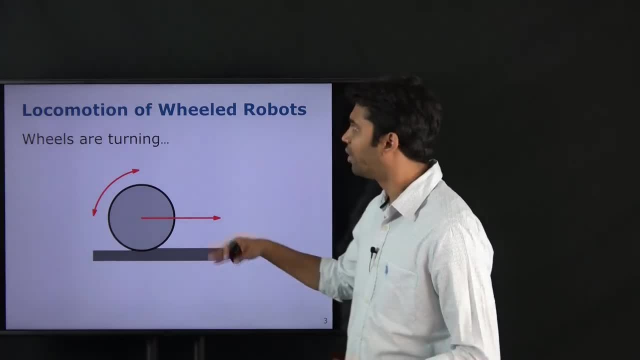 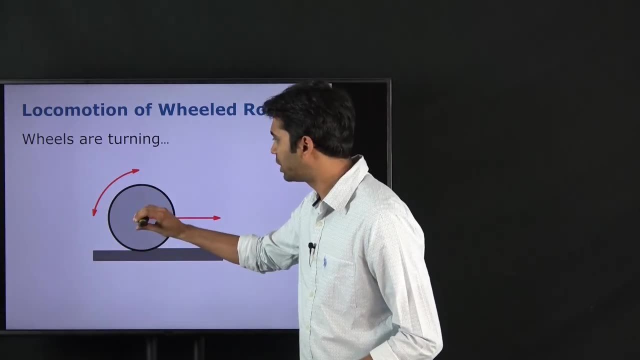 So the basis of a wheeled robot is a wheel. So we start at the wheel and the concept is something we're all familiar with. So we have a wheel and there is an axis going through the wheel. Typically, this axis or this axle is then connected to a motor, which 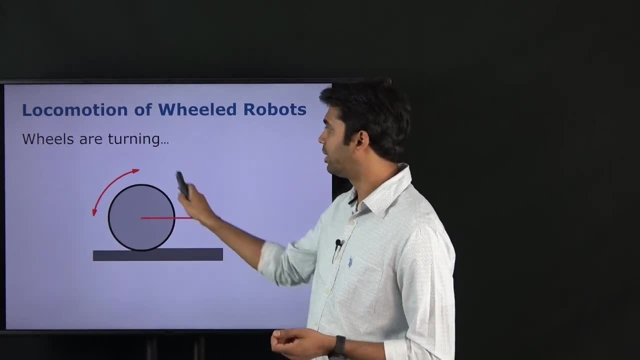 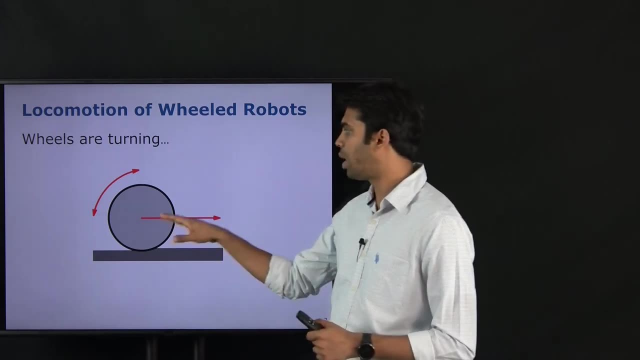 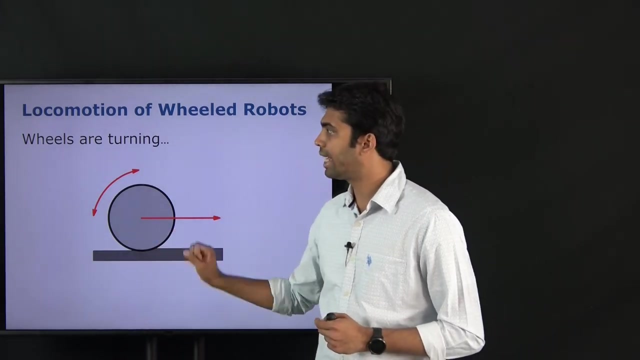 rotates, And for example here, if the motor rotates in the clockwise direction, we end up with a motion which is in the forward direction. So this is a very simple case in 1D. nothing surprising there. However, if we have multiple wheels, the analysis is not so straightforward. 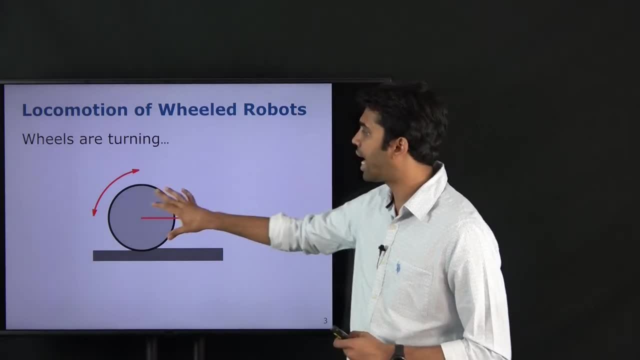 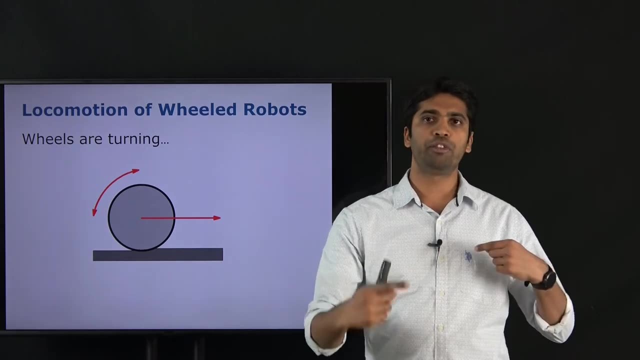 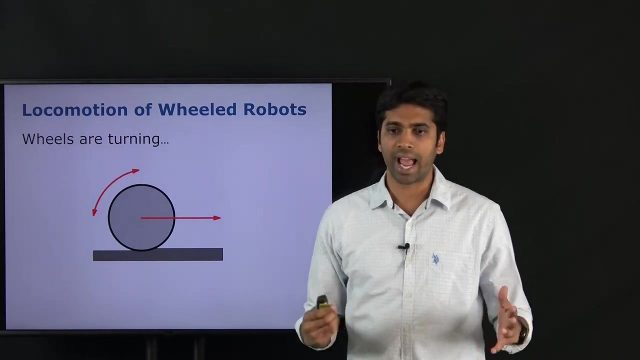 So we want to understand what happens when we stack several of those wheels on a mobile platform, and we want to understand what's the resulting motion when we apply different, for example inputs, different velocities on each of these wheels. how do they then react? right? So let's? 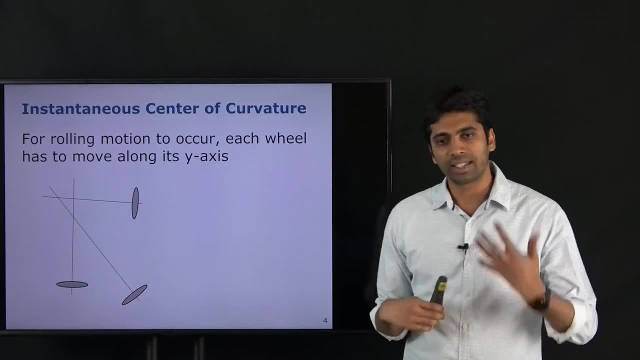 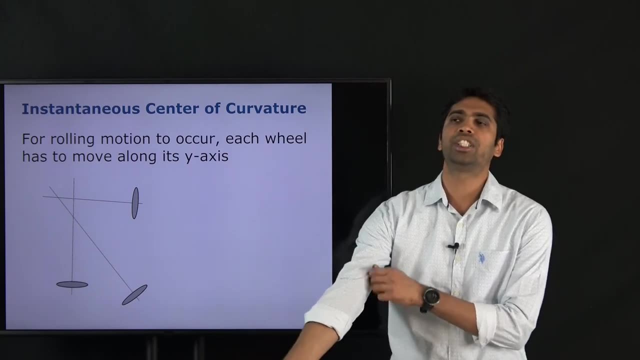 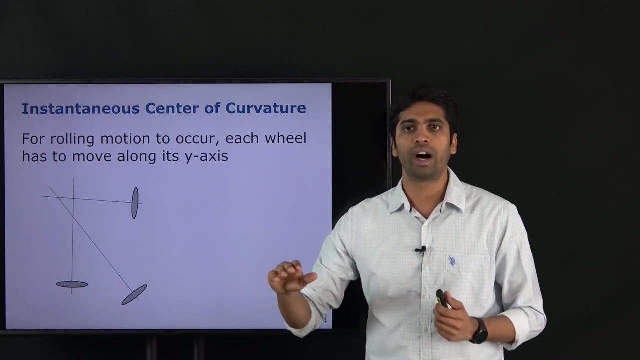 see. So let's see how this works And to understand basically this motion, there's this concept of instantaneous center of curvature. Essentially, what this means is that if we make our whole robotic system move around a certain center of curvature, then we can ensure that the wheels 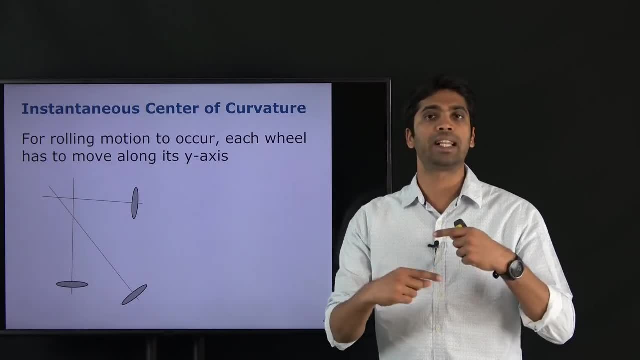 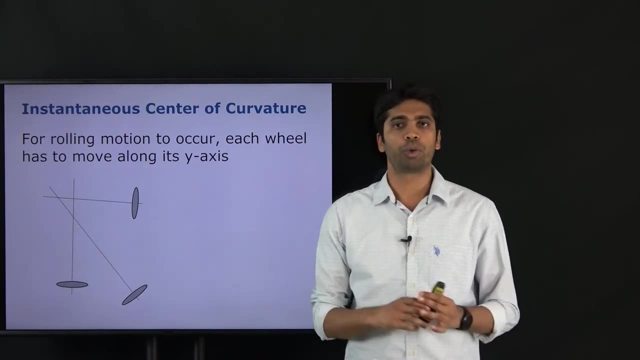 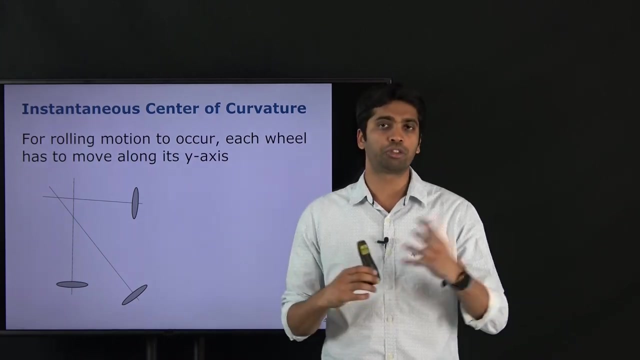 that are attached to this system move smoothly, So basically they roll When they roll. they move smoothly, So they roll, They start teardowning on the surface instead of skidding around. So what we really want to avoid is that the platforms skid around in the environment, as then there'll be large forces both on 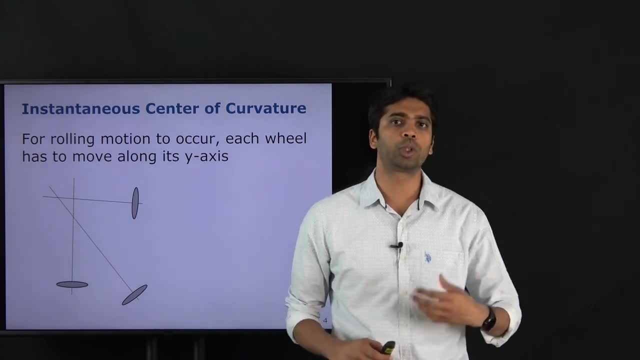 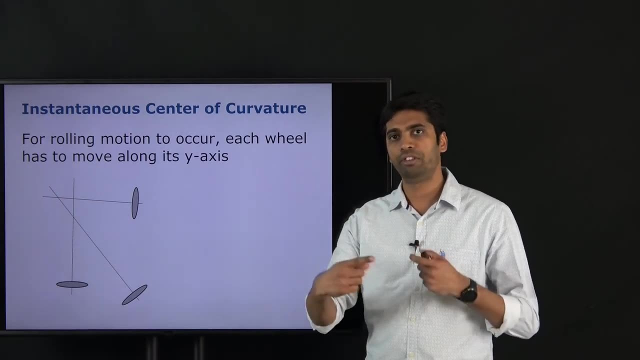 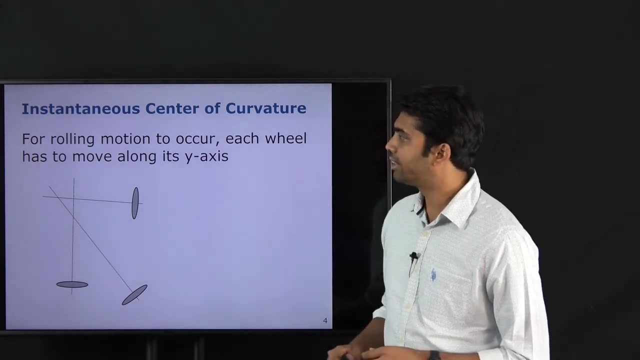 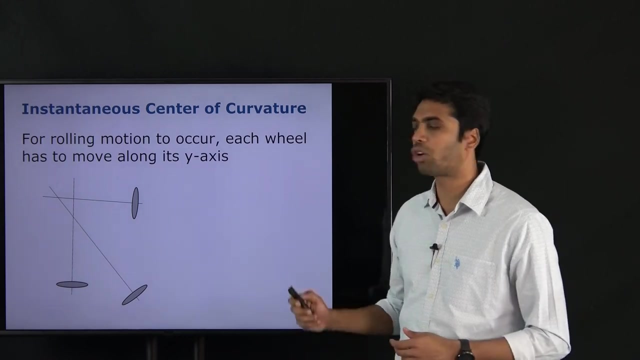 the on the floor itself where the robot is moving, but also large forces that are acting on the platform itself. So the idea is to have the wheels always rolling, And one of the ways to actually ensure this rolling is is to make sure that all the axes of the wheels are intersecting at a common point. So this is not. 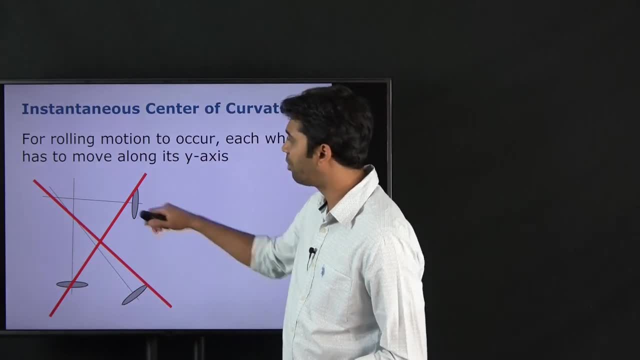 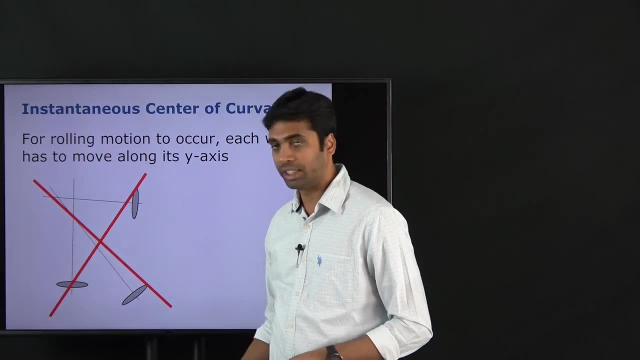 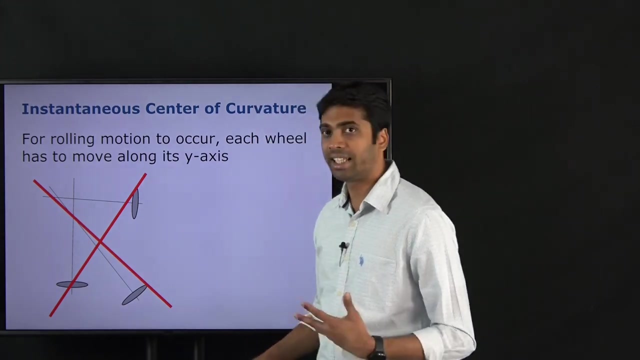 good Why? Because, for example, if say, these are three wheels that are on our platform and there is this axis which passes through each of these wheels, and since each one of these wheels is rotating, they do not have a common center and therefore what will happen is one or more of these. 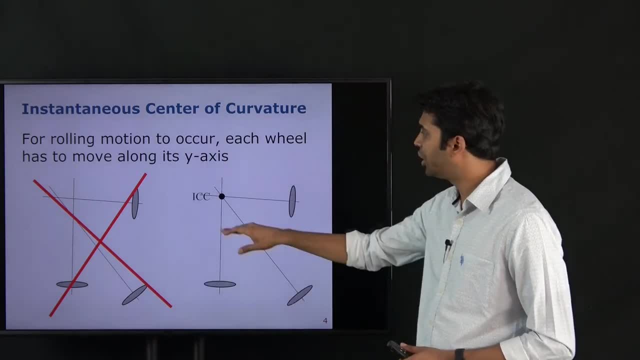 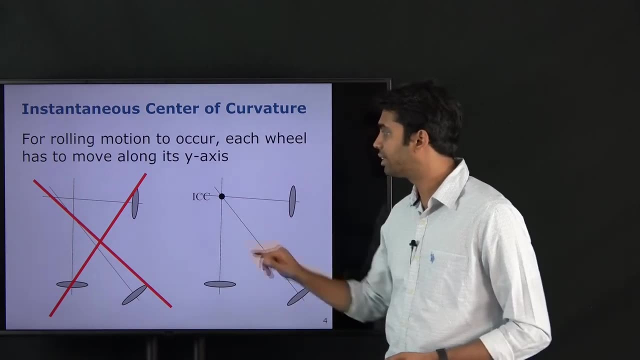 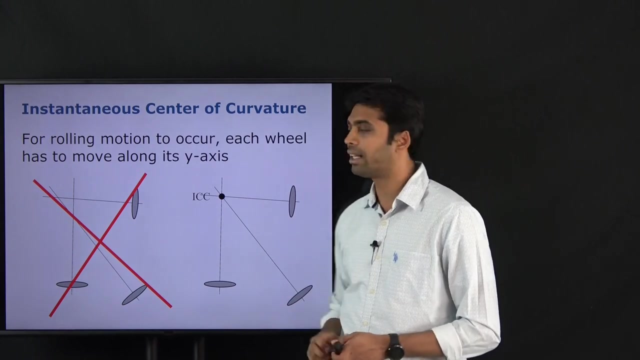 wheels will be skidding. Instead, if we arrange them in the following manner, such that the axes which pass through each of these wheels pass through an instantaneous center of curvature, then they can all move smoothly as one object around that ICC. So there are two ways to look. 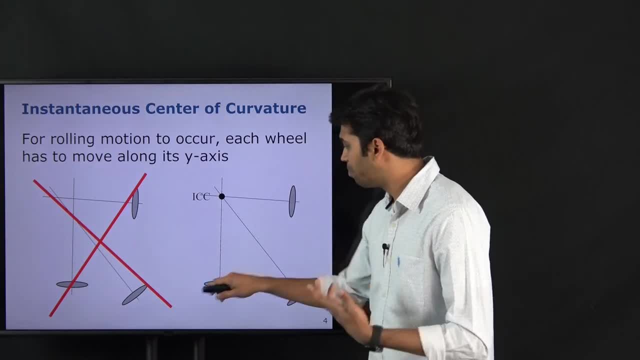 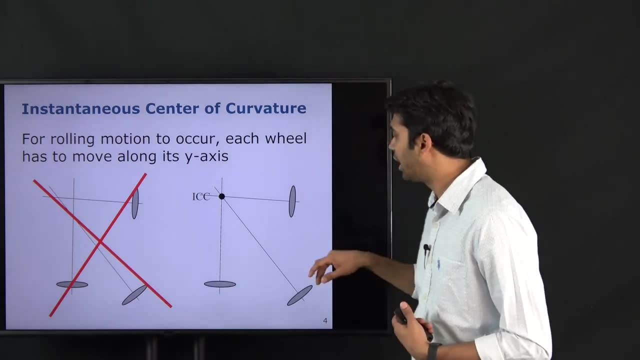 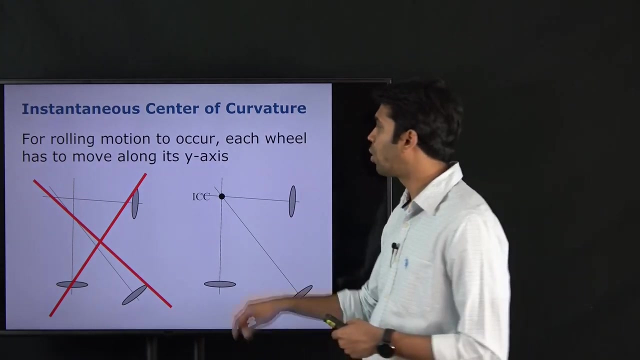 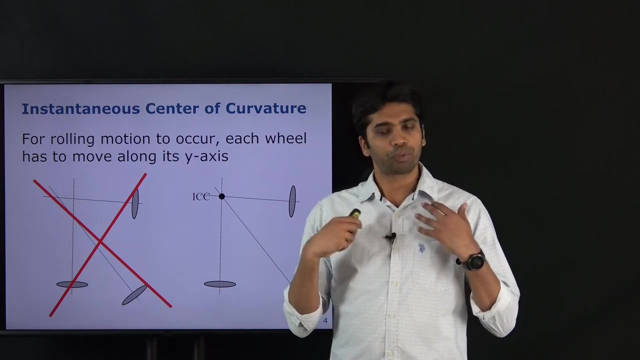 at it. Either we can see them as multiple wheels on the same platform, or we could see it as the platform at different points of time, And in either case, we would want them to move in such a manner that there is always one point around which it's moving along a curve, And what we want to do is what we. 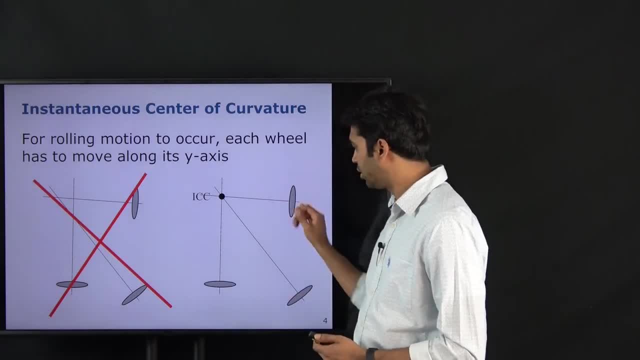 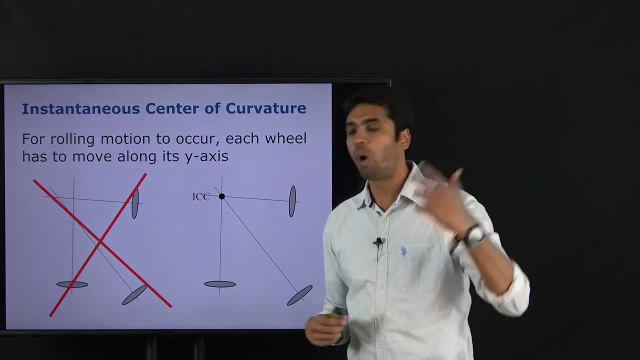 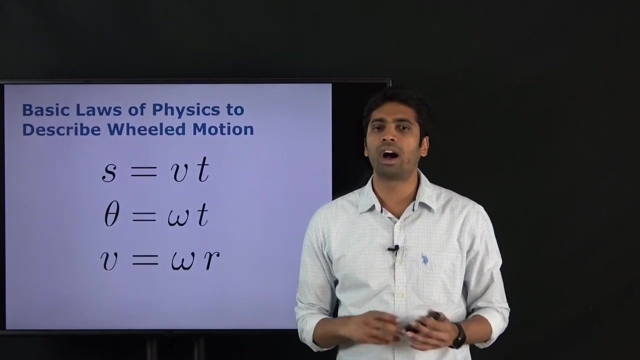 want to essentially set is: we want to control these different wheels, so by spinning them at different rates or by steering them in a particular manner, such that we always maintain this one point of the wheel rotation. So, in order to do this, let's start off with the basic laws of physics, which we will use. 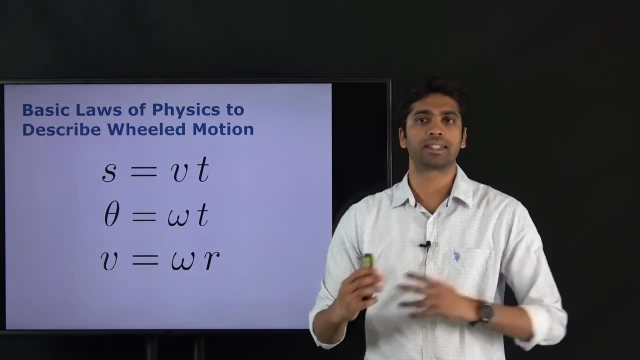 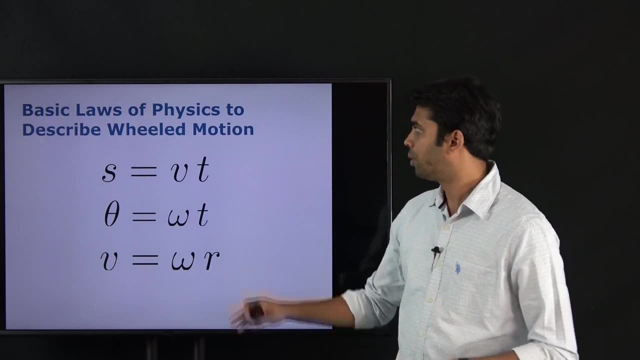 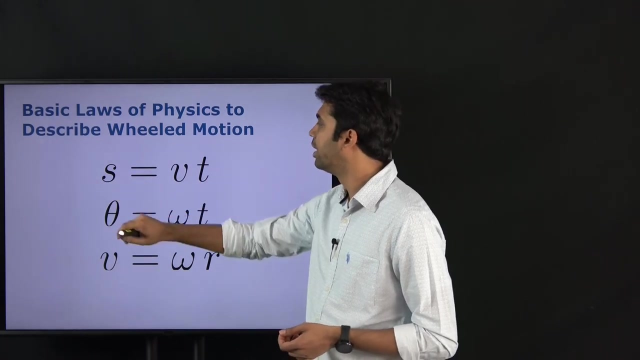 to derive these equations and to understand how the platform moves while following a particular arc, for example. So, for example, the first law here is a very basic one which says the amount of distance moved s is nothing but the linear velocity of the platform multiplied by the amount. 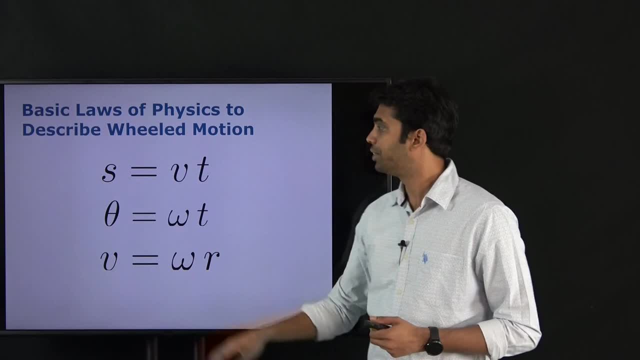 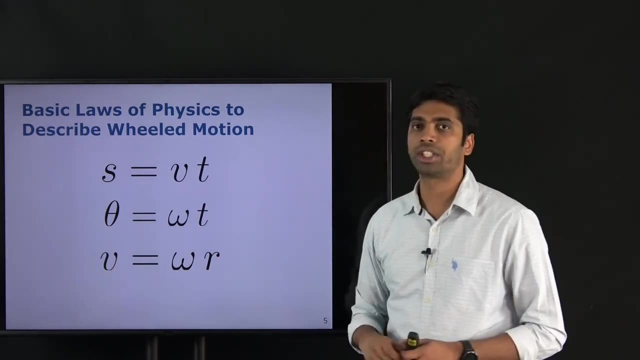 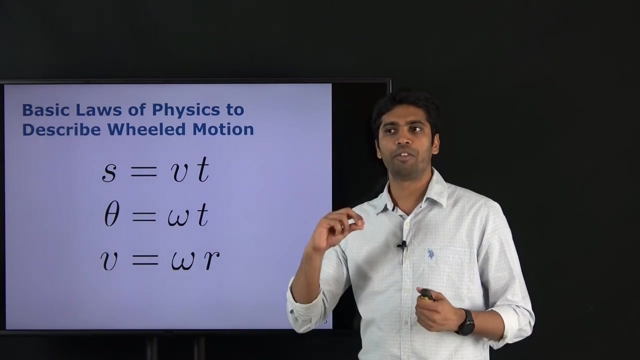 of time for which that particular command has been given. So this is a really simple model in the sense that we are also neglecting any accelerations here. So there are no acceleration terms. Essentially, this means that we are making the assumption that we can supply a particular 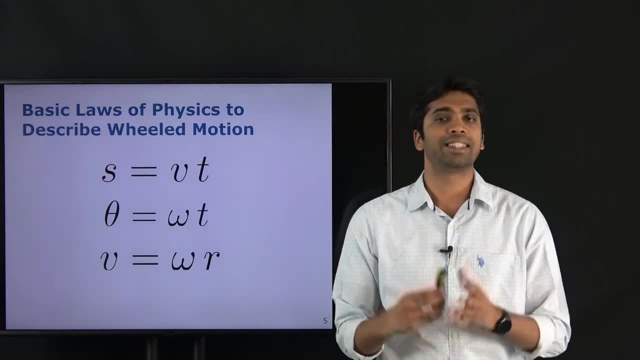 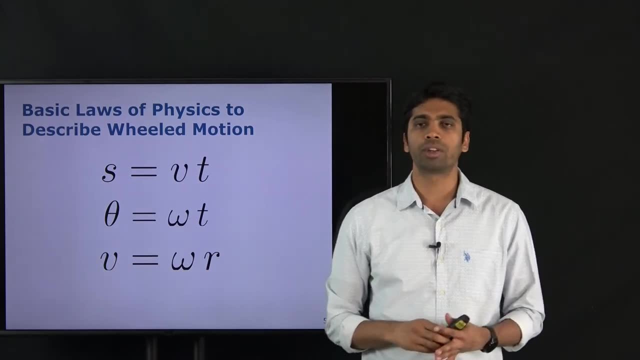 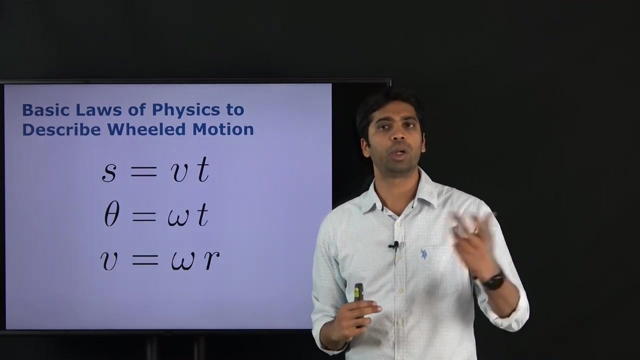 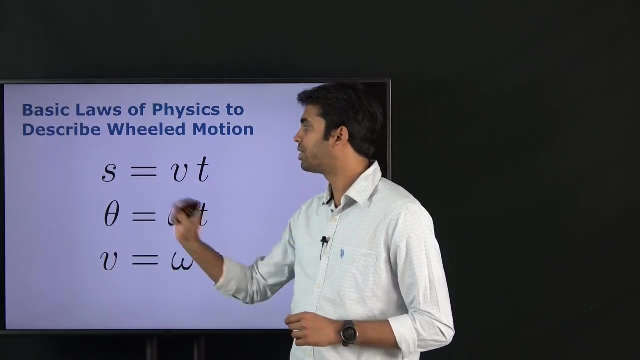 velocity to the platform instantaneously. This is typically not the case in real robots. You often require a certain time in order to reach a desired velocity. But it so happens that for controlling robots or for understanding the motion of robots at lower speeds, this is a fair enough assumption, And the next equation that we see here is the: 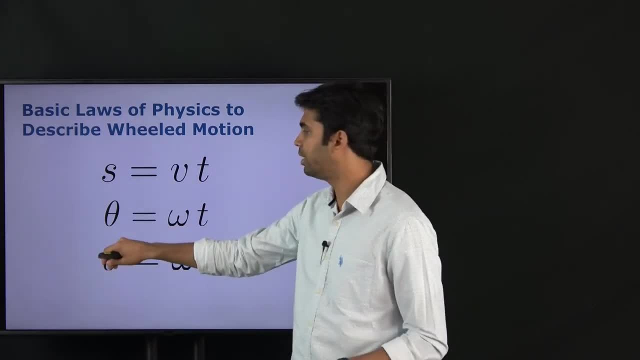 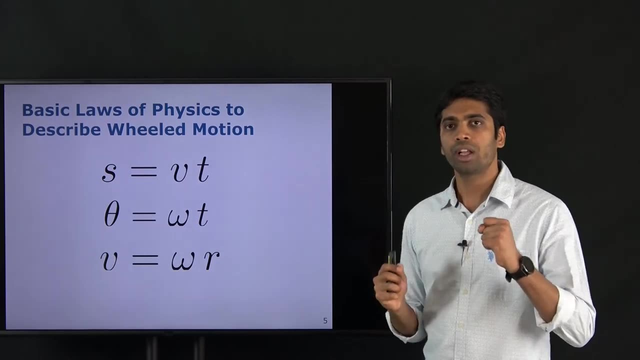 angular orientation of our platform. So the yaw angle, in this case represented by theta, is nothing but the angular velocity of the platform multiplied by the amount of time it takes for the robot to move. So the angular velocity of the robot omega multiplied by the time for which that particular 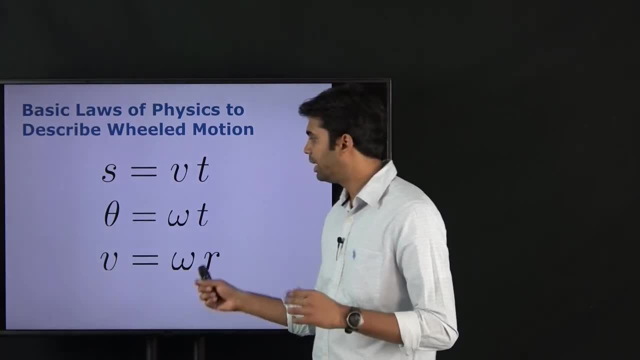 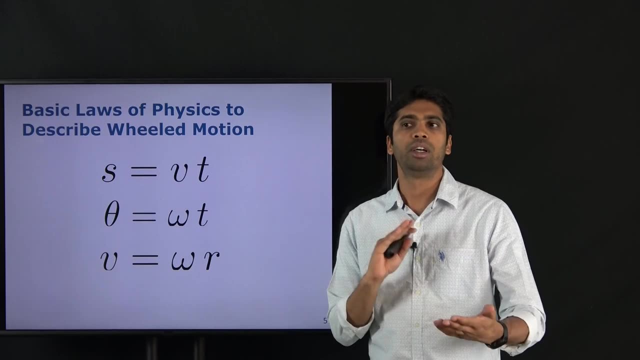 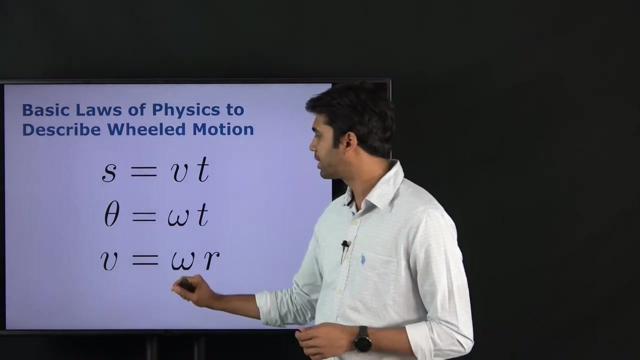 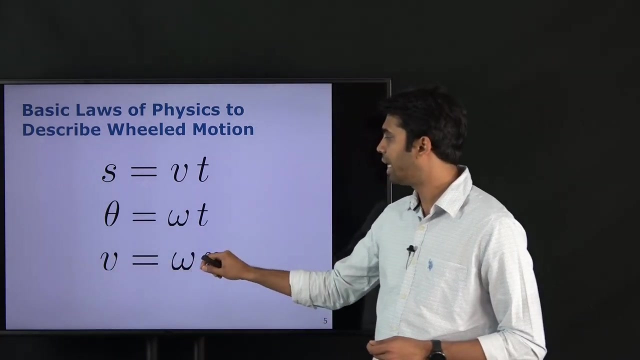 angular velocity has been applied. And similarly we also have a relationship between the linear velocity and the angular velocity when a particular platform, or any point mass for that matter, is following a circular arc. So in this case the relationship between the linear velocity is nothing but the angular velocity times the radius of curvature of the arc which that particular 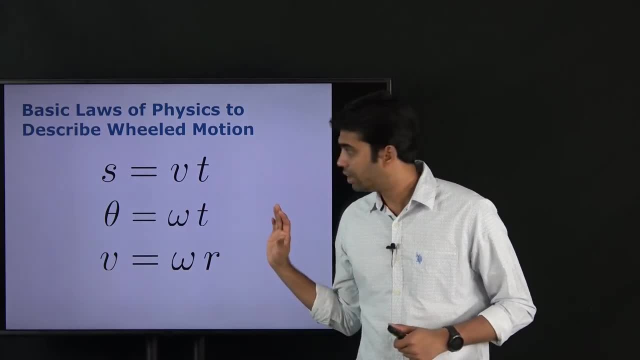 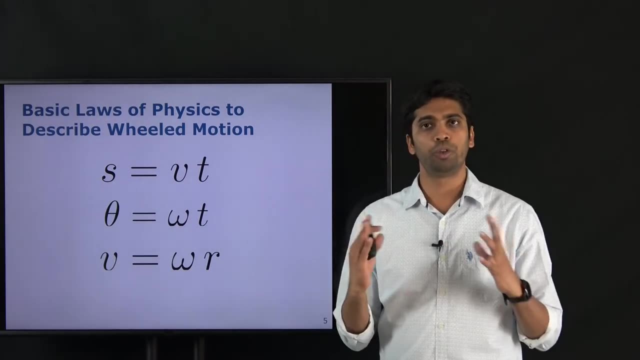 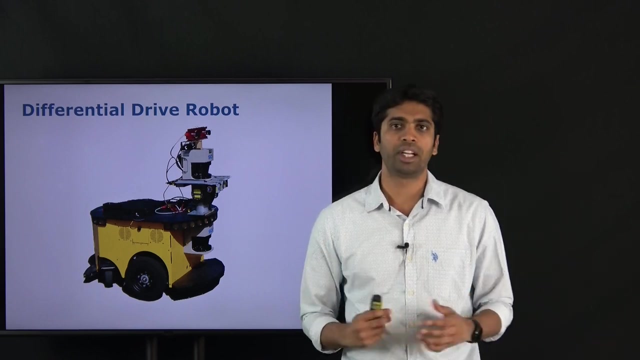 platform is following. So these equations will be used in order to understand how different drives or different robots actually move in their environments. We start off with the most basic or the most common drive- what is also called as differential drive- that you see here. 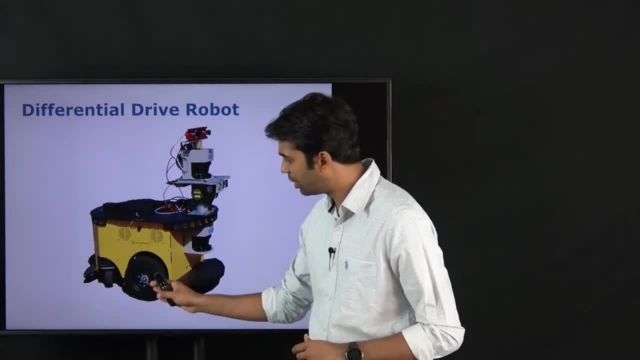 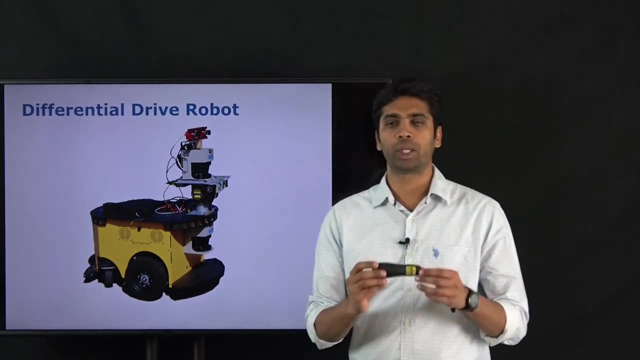 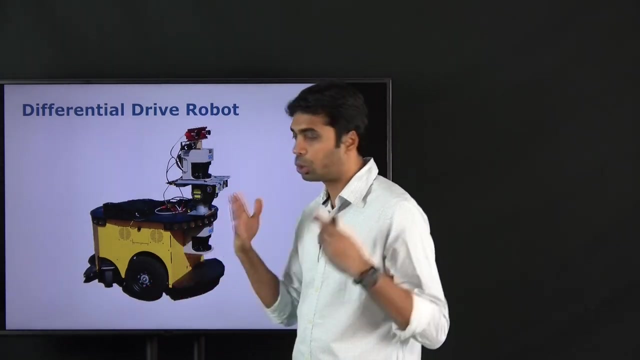 So, basically, a differential drive robot has two wheels, So one we see on this side and one on the back side, which we don't see here. But and basically, each of these wheels is connected to an axle, connected then to a motor which rotates, So what we can do is to move each of these two. 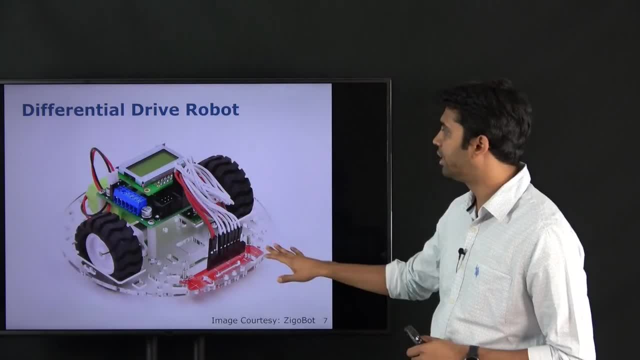 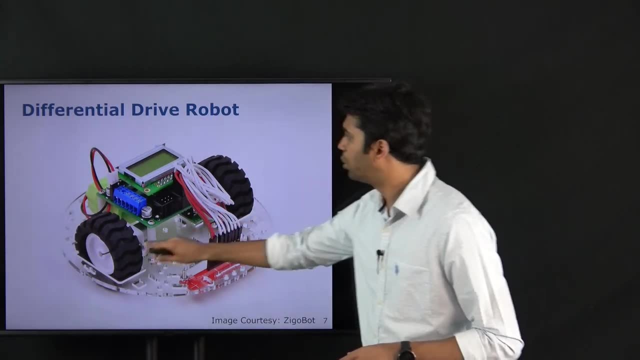 fields independently. We can see this a little bit better in this picture. here It's a smaller robot, but the idea is the same. It's also a differential drive robot- Again, two wheels connected to two individual robots which can spin at different velocities, if you wanted. 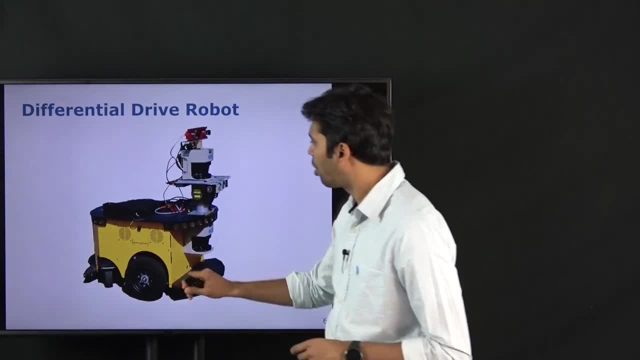 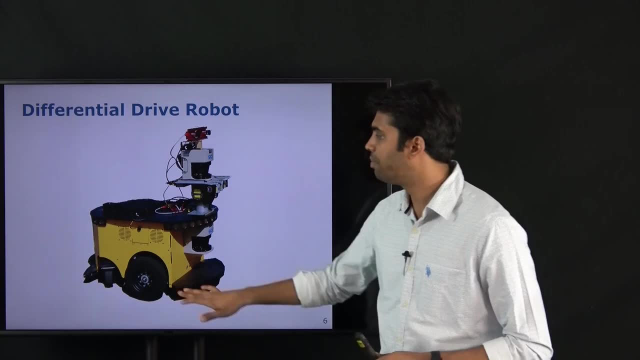 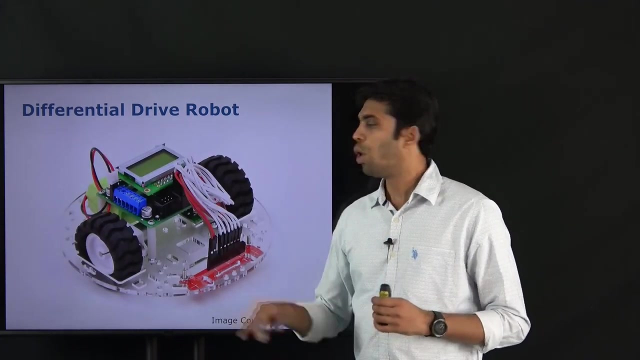 to, and often times, what is often kept is also a third wheel, which is a free moving wheel, also called as a caster wheel. So it's mainly to maintain a balance and is not an active wheel, so to say. So what we can do here is to set the velocities of each of these tires. 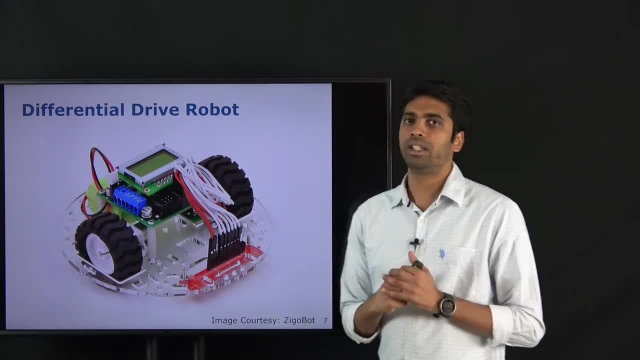 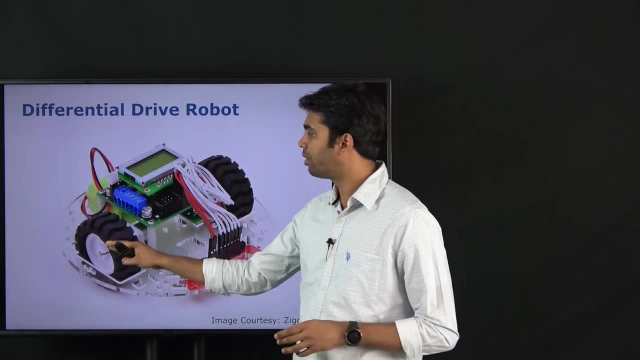 or the wheels independently and, for example, let's say we want to go straight with this particular robot. The answer is quite simple. We set the same velocities both on, let's say, the left wheel and the right wheel, and this would result in the platform moving in a straight. 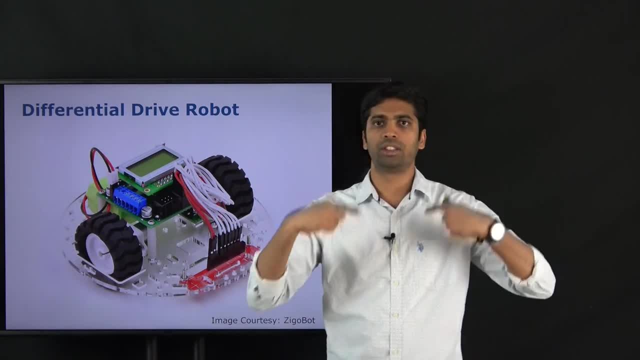 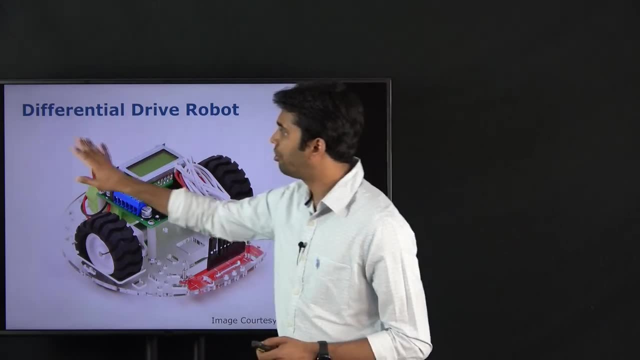 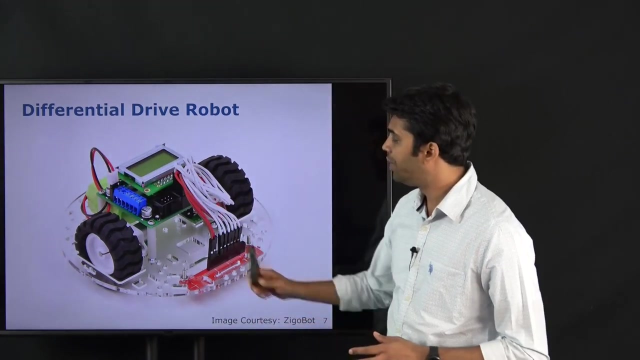 forward manner The same. if we want to move back, just the velocities are reversed and in this way we can move back. However, if we want to move along a curve, this changes slightly. So, if you think of it, if you want to make a curve like this, the wheel which is on the 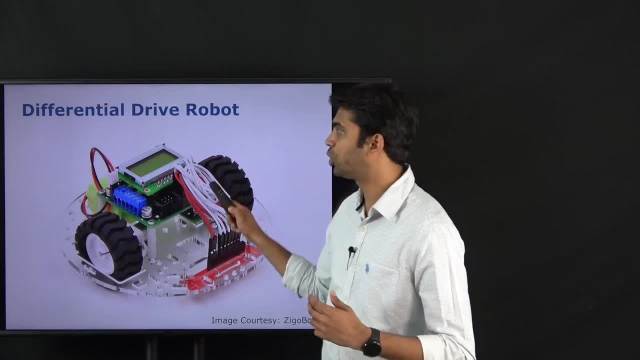 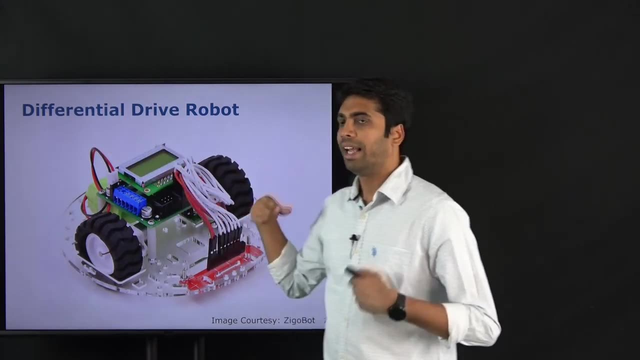 left, which is actually also, in this case, an inner wheel- it's towards the curve- has to travel a distance which is less than the distance that the outer wheel has to travel. And so, since the outer wheel has to travel a larger distance when it's following this particular 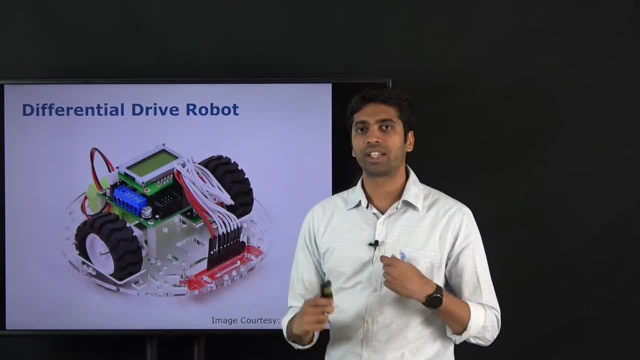 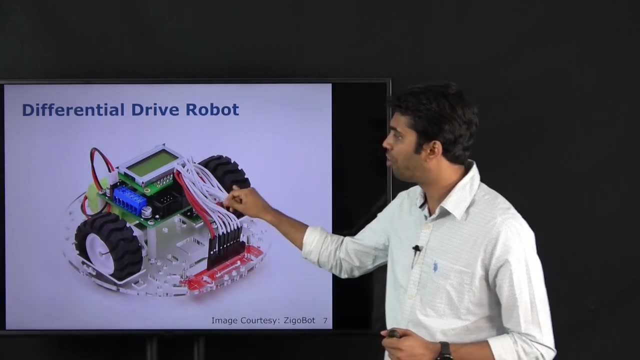 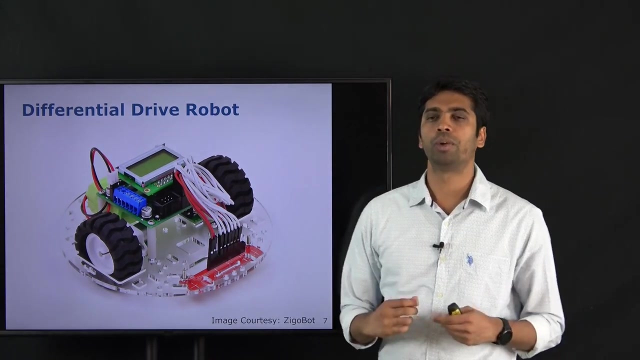 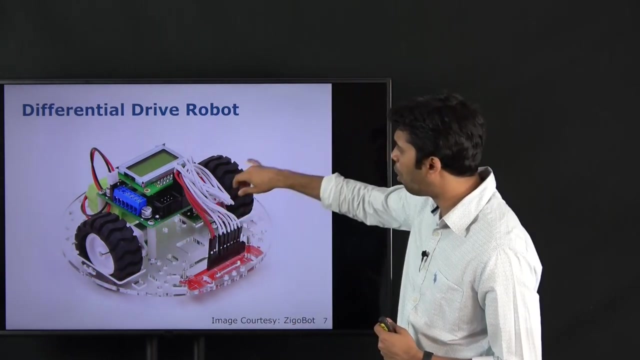 arc. it needs to spin faster such that, overall, they don't skid. Okay, And also, if you think, in terms of the instantaneous center of curvature that we just introduced, by construction these differential drive robots always have an instantaneous center of curvature. For example, since these accesses pass through both these wheels, essentially the instantaneous. 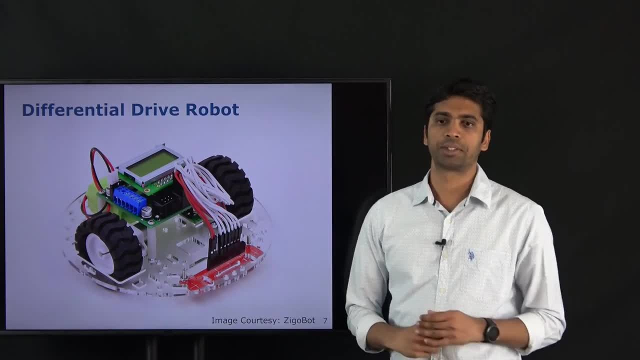 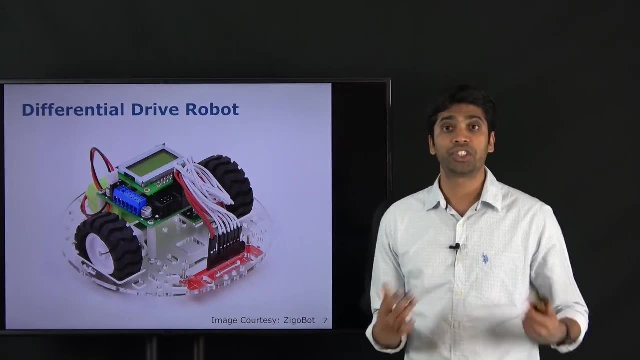 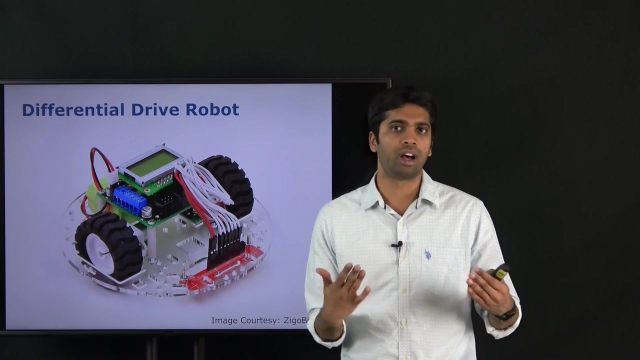 center of curvature will lie on that axis. What's also interesting is that these kind of robots can also spin- Okay, They can spin on spot, which is really interesting to have if we have confined spaces. You can imagine that this is not possible for a car or a car like robot, which also we saw called. 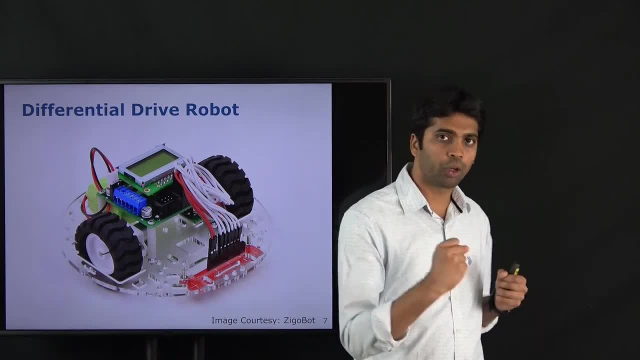 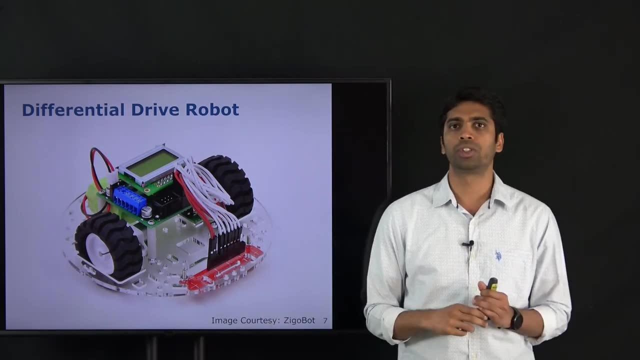 an Ackermann robot, because there you can't really rotate on spot. There's a minimum turning circle that's there, which restricts us from making arbitrarily sharp turns, so to say. However, for differential robots, this is quite a nice property. So how this is done is that. 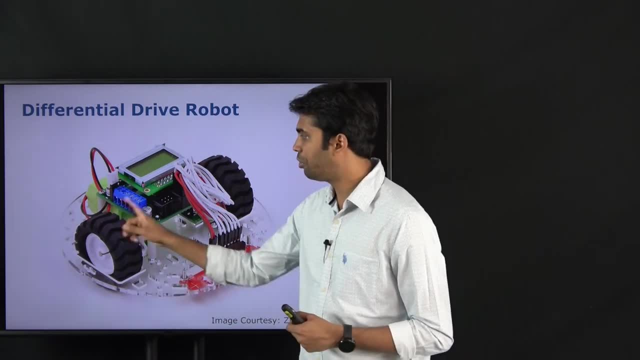 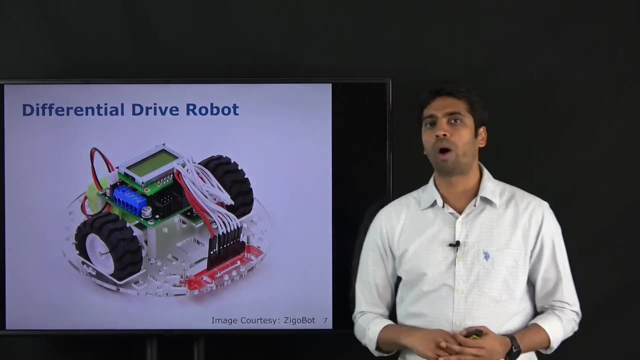 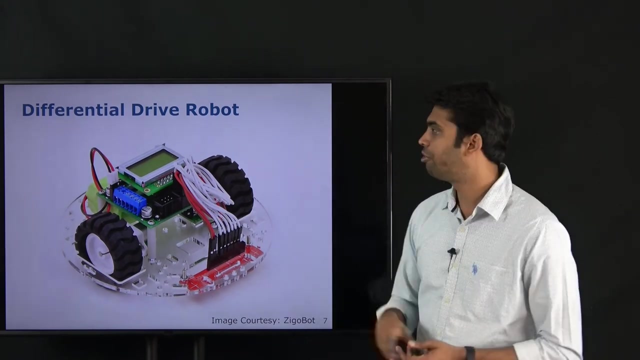 by rotating the one of the wheels, so let's say, the left wheel in, say, clockwise direction and the other one in anti-clockwise direction, we are able to spin on spot, and by switching it we can spin on the other way as well, And so these are quite interesting properties for a differential robot. 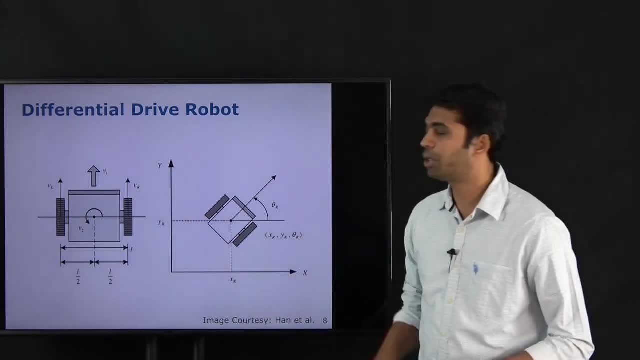 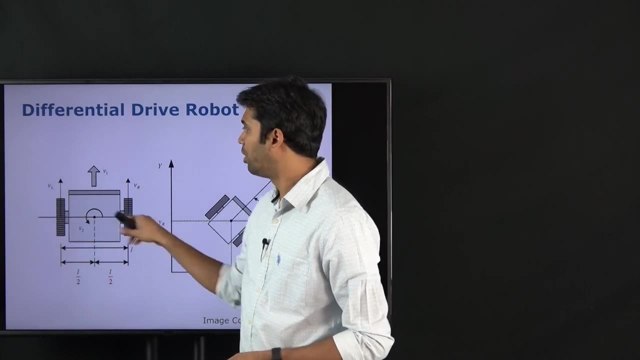 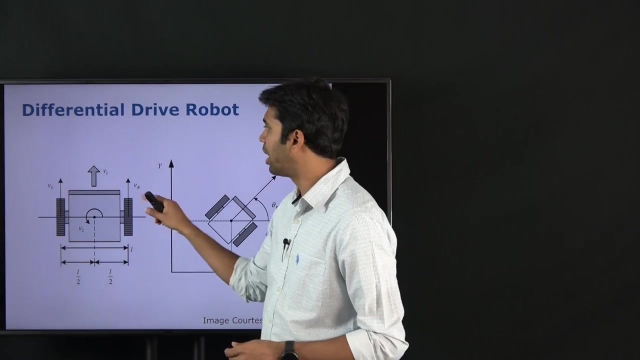 Let's now put some variables on this robot, to understand what are the different terms that we are interested in, and so on. So, like we said, So we have two velocities, the left and the right. So these are the velocities that can be set as an input to the system, So VL and VR here, And then there is angular velocity. 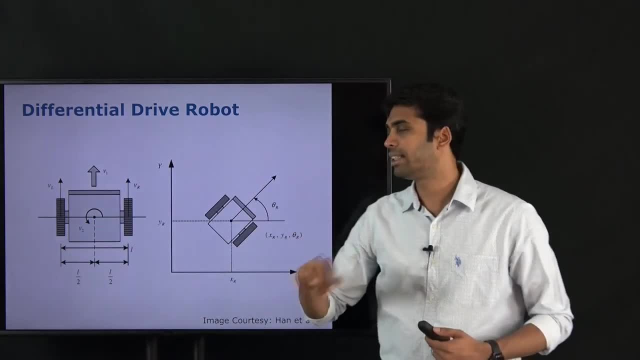 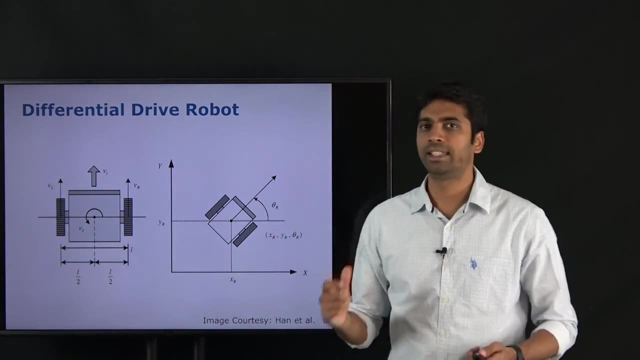 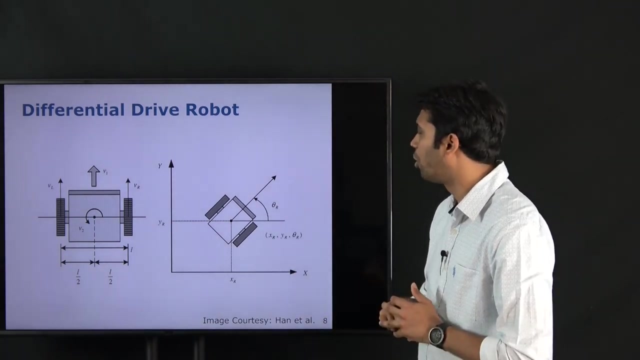 that exists along, let's say, the center of mass of this robot. And then there's also the width of these robot. We will see why these particular terms are important in order to describe the motion that such drives actually follow, In addition to its xy, for example, position, here defined by its center of mass. we are 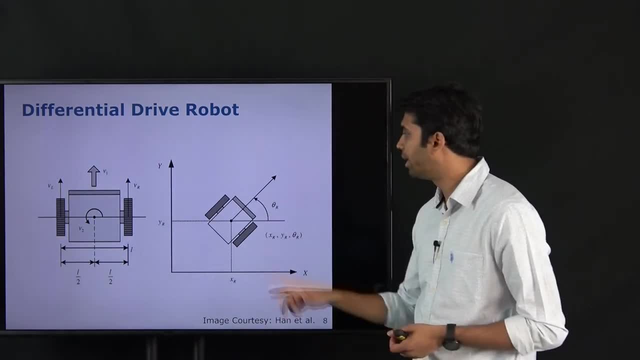 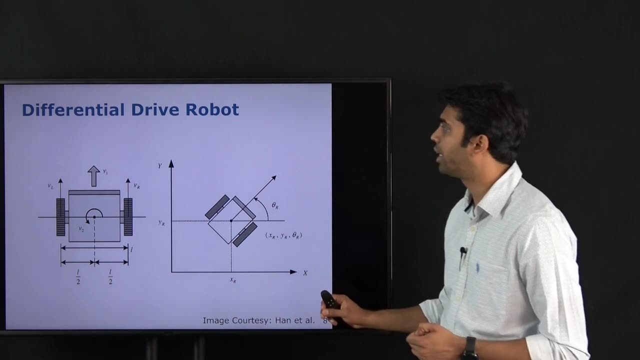 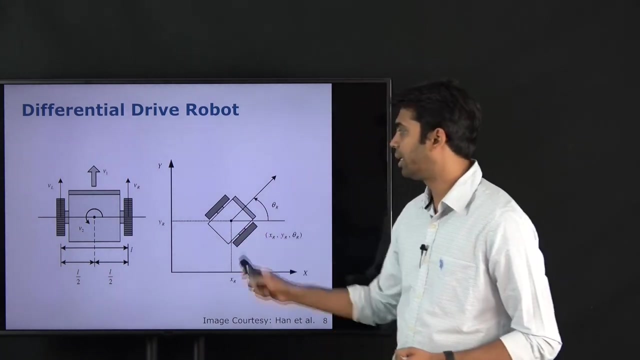 also interested in the orientation of the robot here given by theta. So to describe the position of our robot, of this differential robot, in a global coordinate frame, what we would require essentially is the x and the y positions of the center of mass, and often this is taken on the or at the midpoint of the axis that passes through. 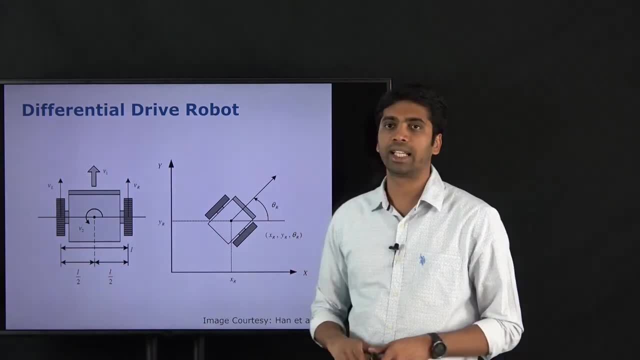 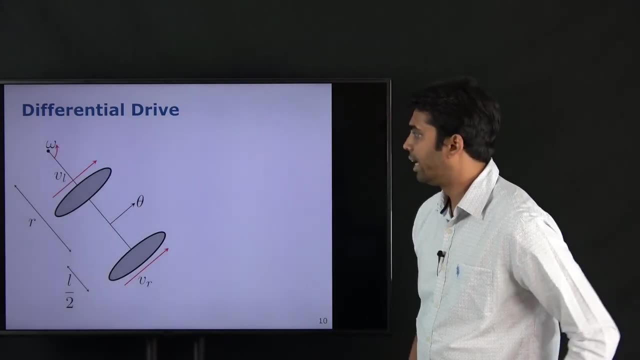 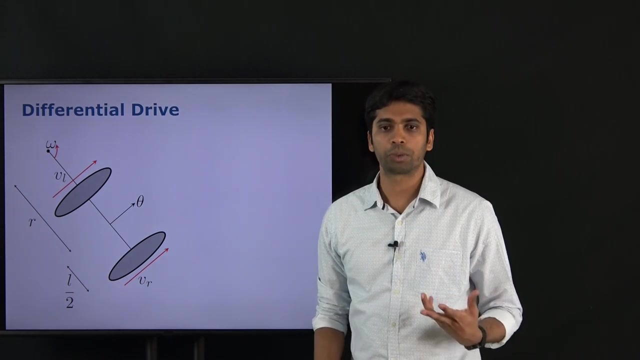 these wheels. So somewhere here, and we are also interested in the orientation of the robot. Okay, so let's see a little bit in more detail. Again, it's the same thing what we saw before. We have a left velocity and the right velocity for the two corresponding wheels We have 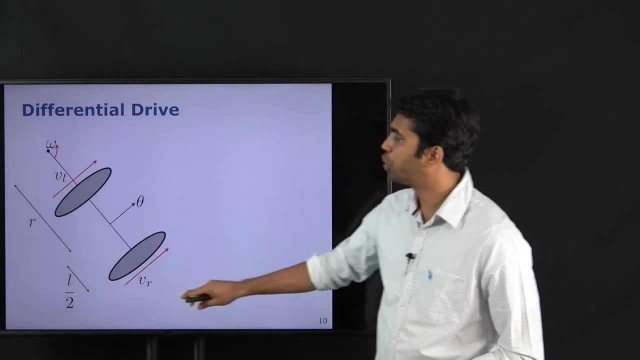 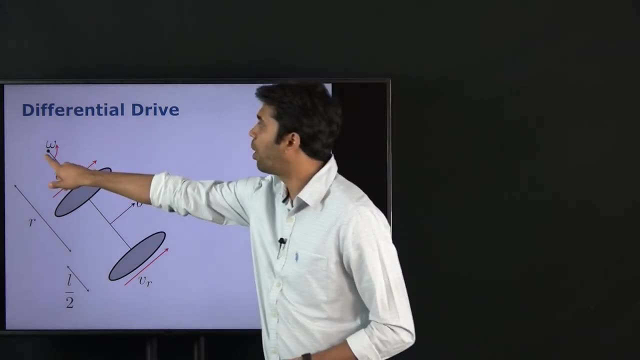 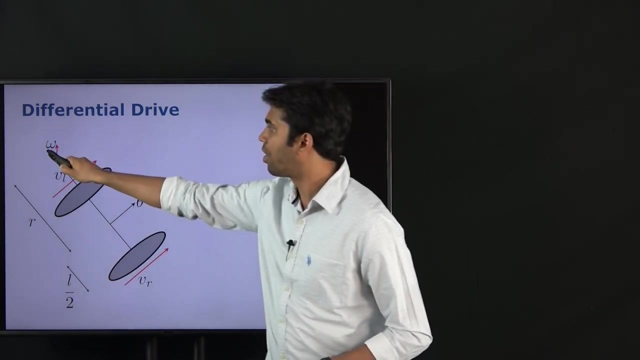 an orientation of the robot, and what we also show here is the radius to the instantaneous center of curvature here. So this point here represents this instantaneous center of curvature. So the robot is making a turn, presumably like this, along this point and of course we have the length of the length. 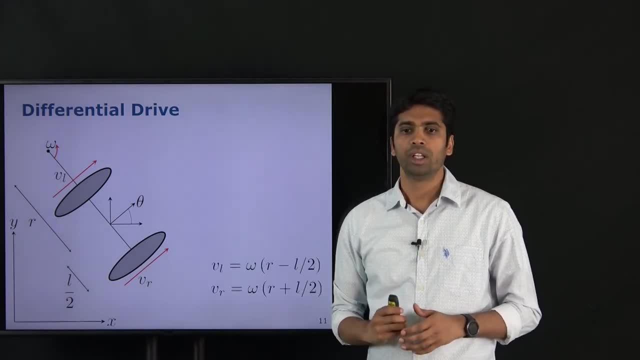 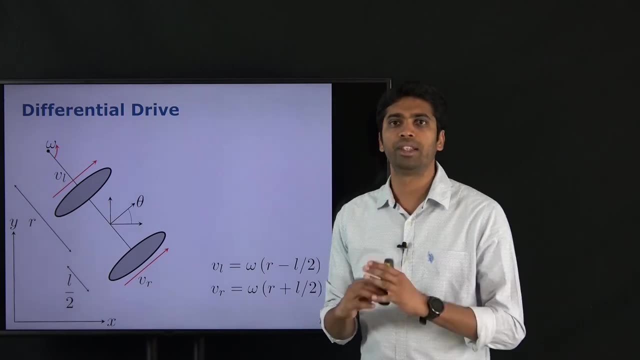 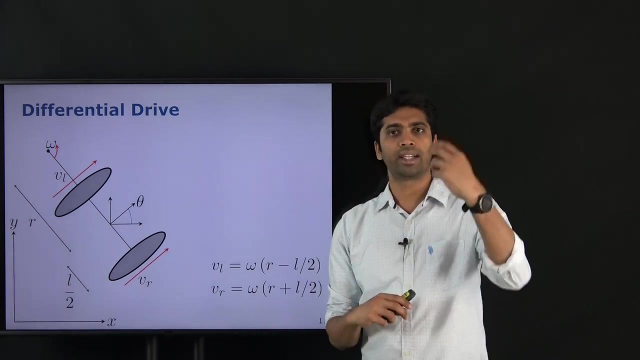 between the two wheels on the robot itself. So now we will use one of the laws that we saw before, which is the relationship between the linear and the angular velocities of the robot. So what we would like to end up with is to understand the motion of the robot in terms. 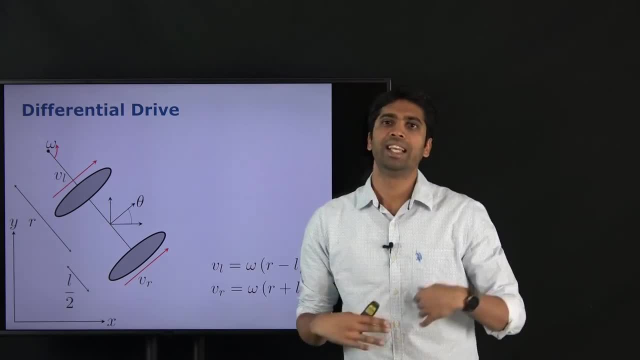 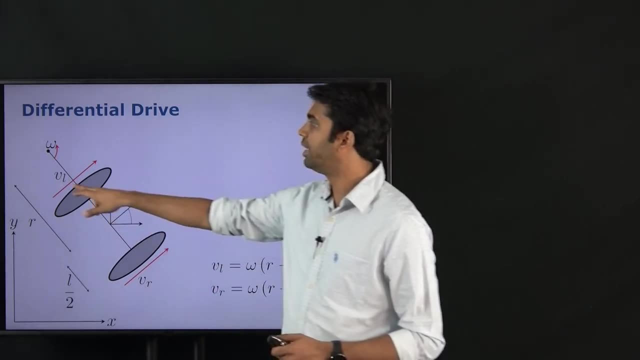 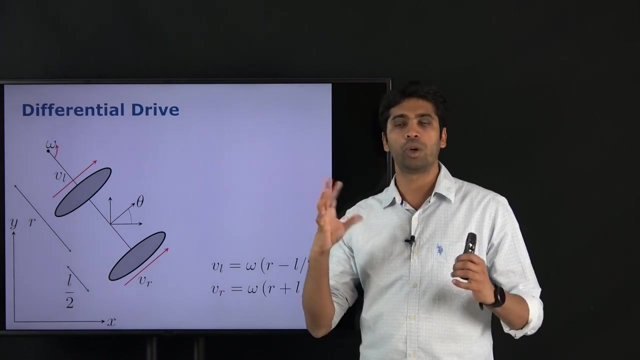 of its linear and angular velocity. so V and ω in terms of the commands or in terms of the velocities that are set to it. So, for example, in this case, vL and vr are the velocities that are set to these two wheels, And what we want to understand is: how does the overall 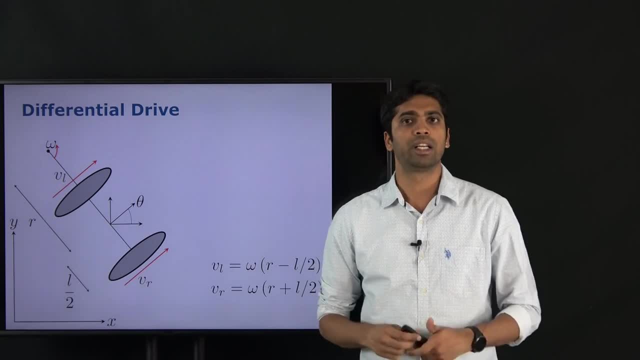 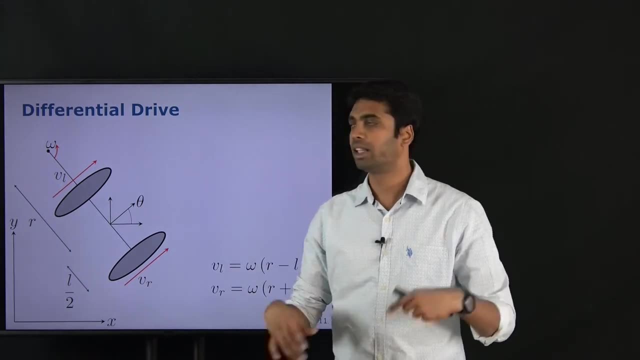 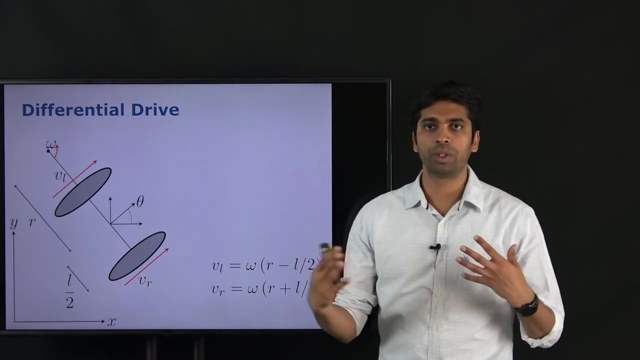 robot, the overall platform, respond to these commands. So we want to understand what the angular velocity is, as well as the linear velocity of the platform as a whole, is given that we set V, L and V R to the two wheels, And so we will develop some equations and come out with these results and see how they 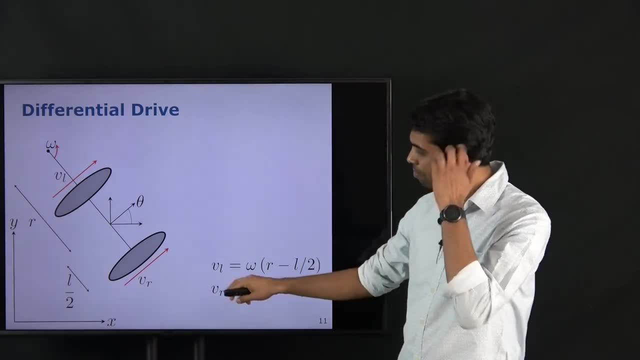 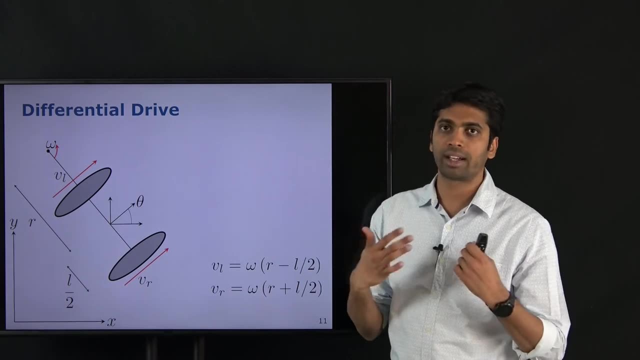 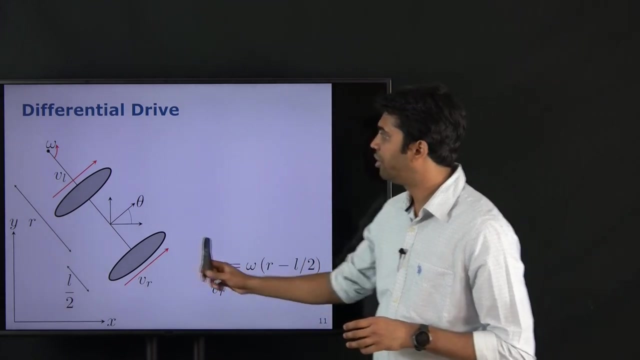 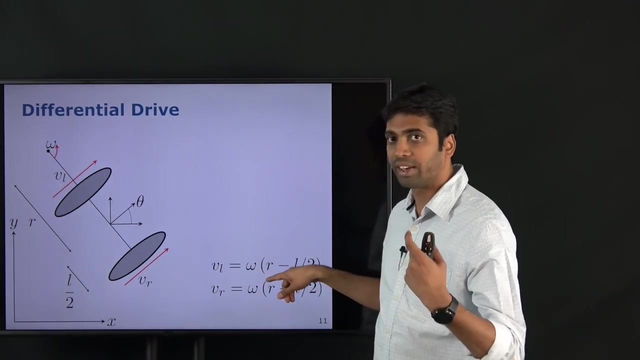 look like and where we start with is the relationship between the linear and angular velocities. So essentially, the formula that we are following is: V is equals to omega times R, where R is the radius of the circle that it is rolling along. So in this case, if we take, at the left wheel here, the radius of the circle that it is following, 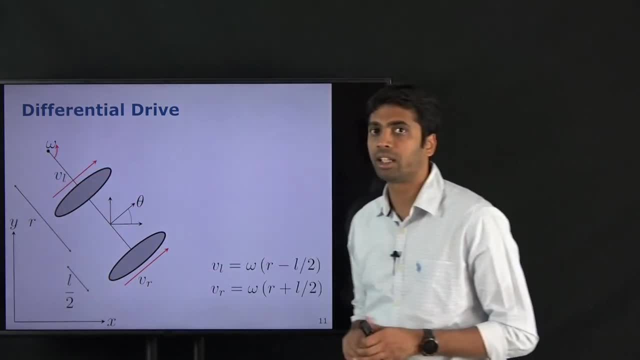 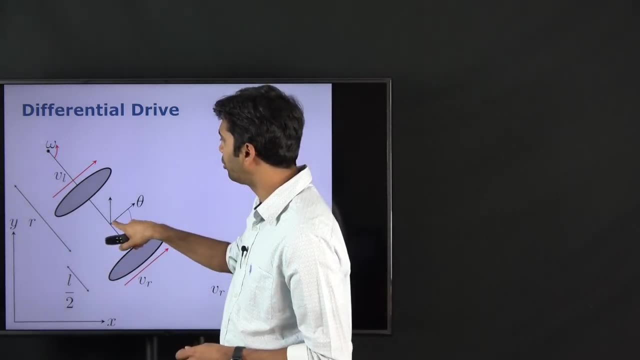 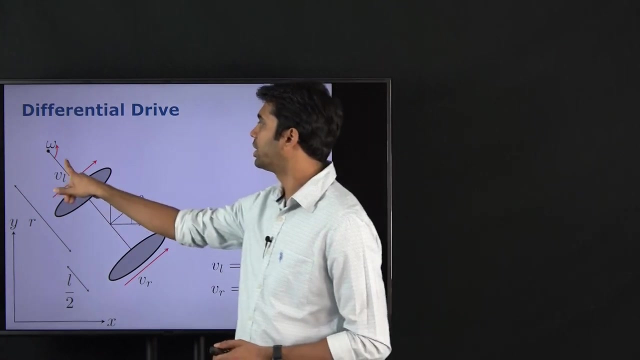 in this case it is the distance to the instantaneous center of curvature- is nothing but R minus L over 2.. So, since R is the distance from the center of the robot to the instantaneous center of curvature and L over 2 is this distance, this particular distance that's left here, is nothing but R minus L over 2, and the same happens. 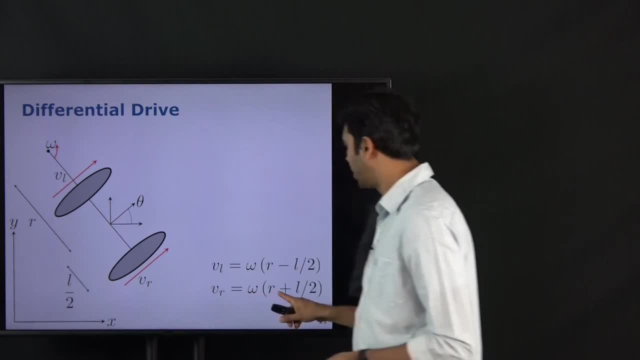 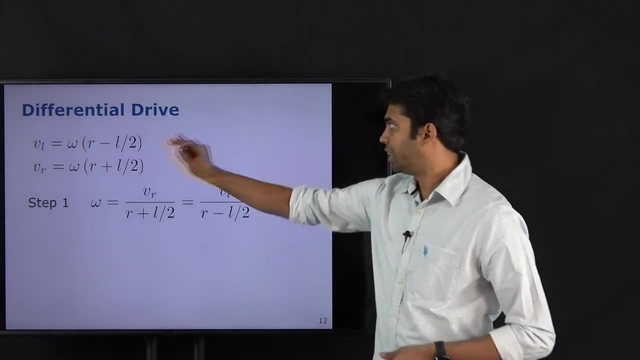 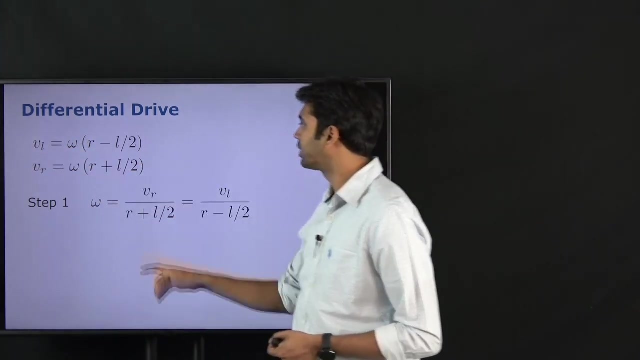 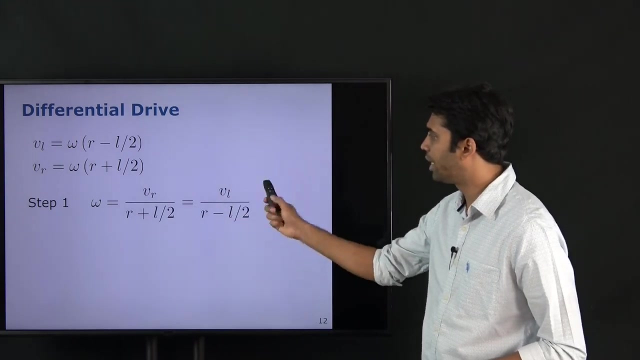 for the right wheel here. So nothing more. but it's R plus L over 2, since it's on the other side. So we just rewrite these two equations here, and the first step is to just take out omega on one side. So what we have is these equations, with Vr over R plus L by 2 being equal to VL over R minus. 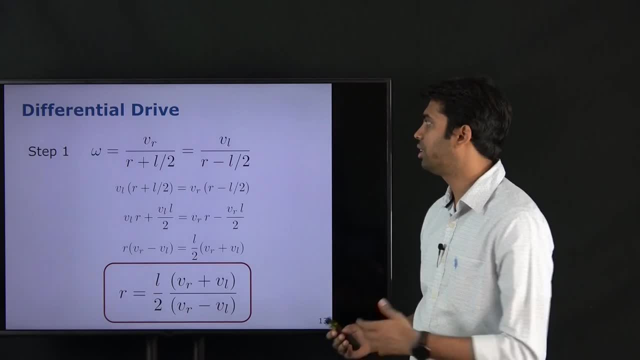 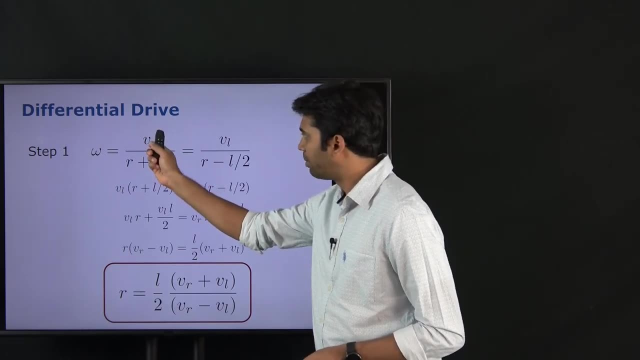 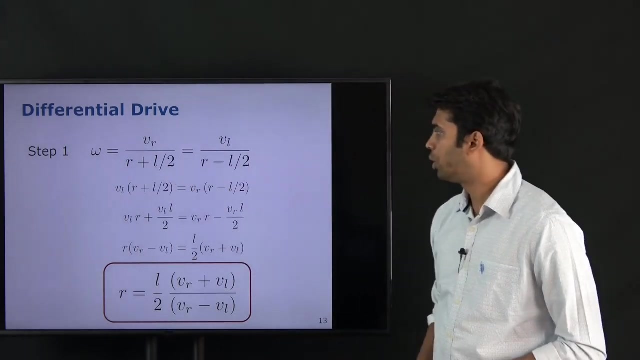 L by 2.. Then we do some algebra, very simple algebra: just multiply and move the terms around. What we would find is: we multiply Vr times R minus L over 2 is nothing but VL times R plus L over 2. Then we can remove some terms and then, if we 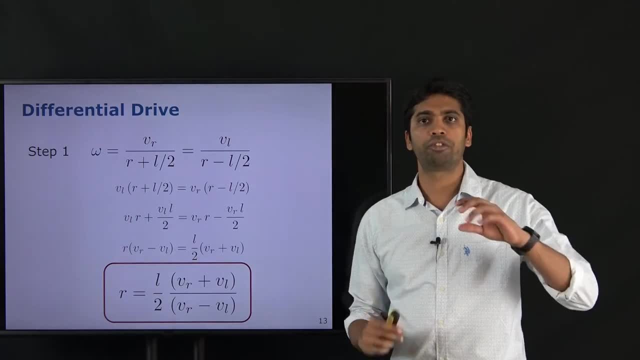 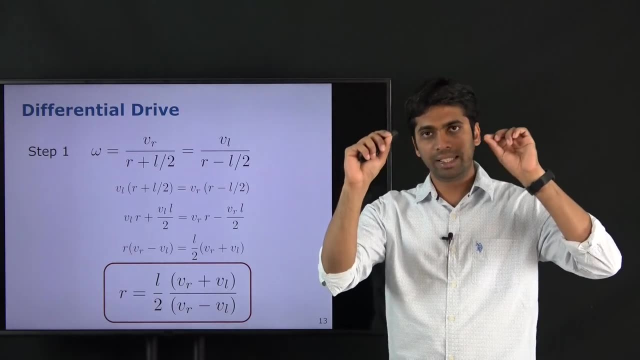 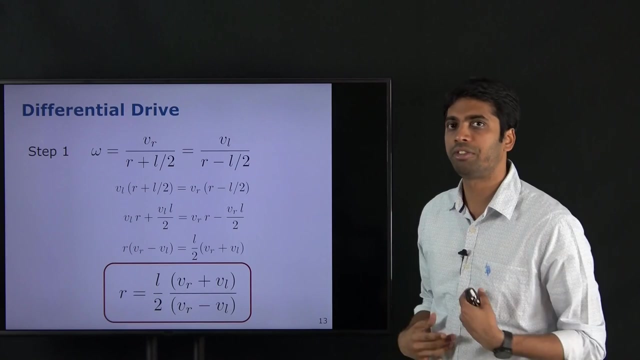 rearrange it. what we would like to find is an expression for the R, So the radius of this distance between the center of the wheels to the instantaneous center of curvature, So this radius of the circle that the platform itself is following around. and if we move these equations, 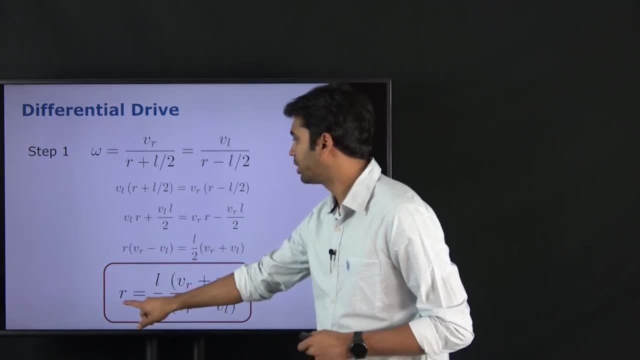 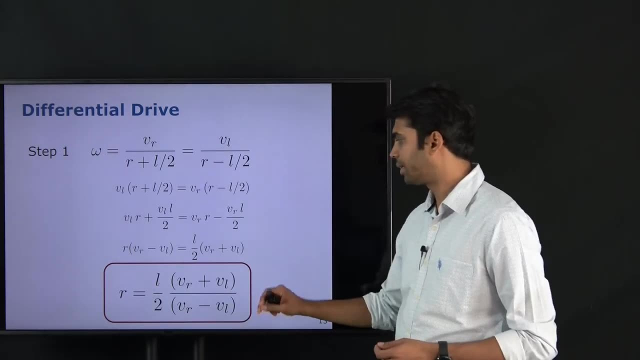 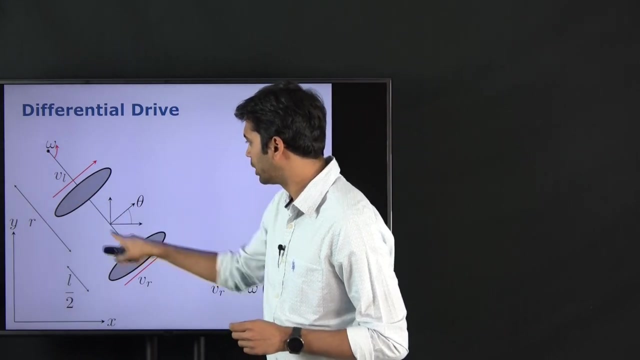 So we take R out and if we move the equations around, what we will end up is an equation for R which depends on two things, or three things, which depends on the L, which is the distance between the two wheels. L is nothing but the distance between these two wheels and it depends on the left and the right. 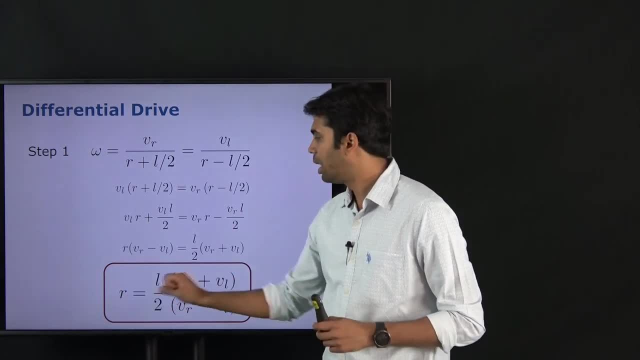 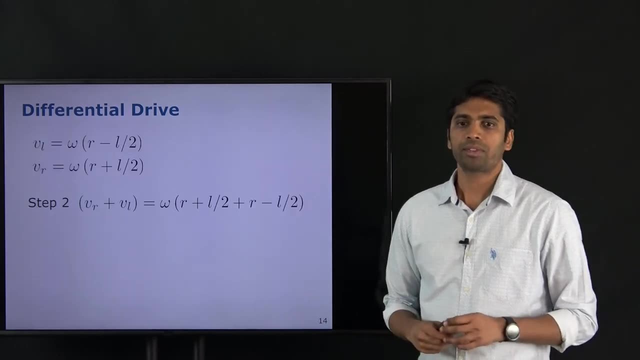 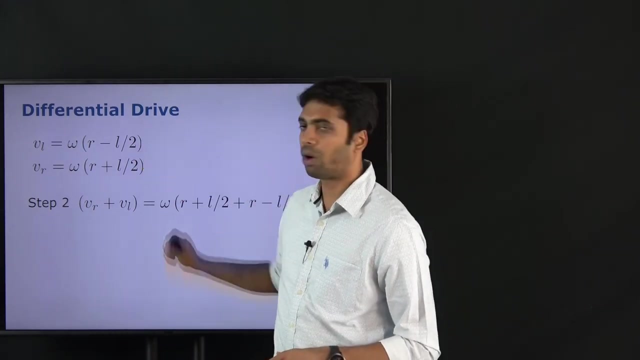 wheel velocity. So now we have an expression for R based on our inputs, as well as some dimensions of the robot itself. right, Let us see what else can be developed from here. So we have these equations which we saw before. We can also add them up, So in this case, we basically add these. 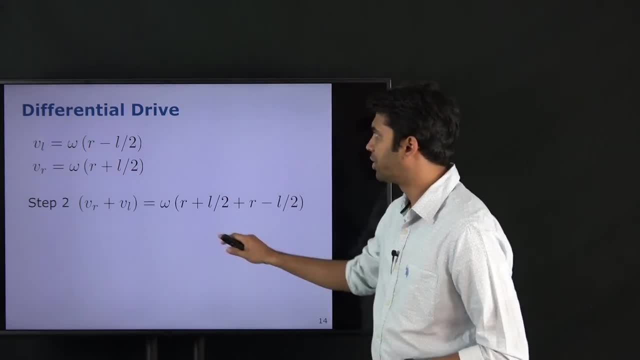 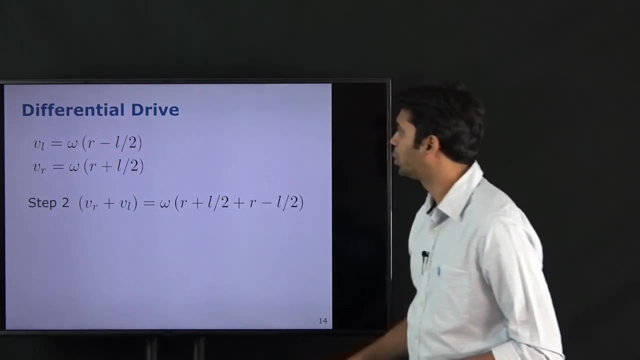 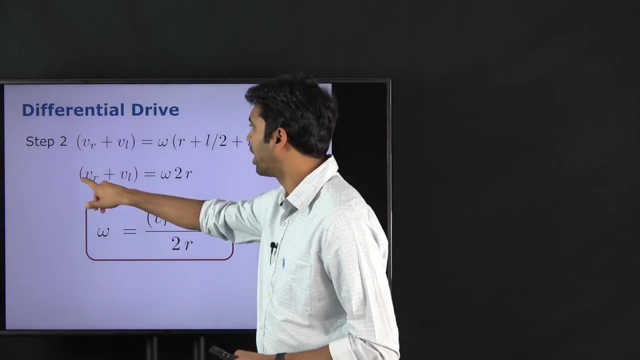 two velocities here and we obtain the equation here. So nothing. VL plus Vr is omega times R minus L over 2, plus R plus L over 2, and these two terms will cancel each other out there. If giving us VL plus Vr or Vr plus VL equals to 2 omega. 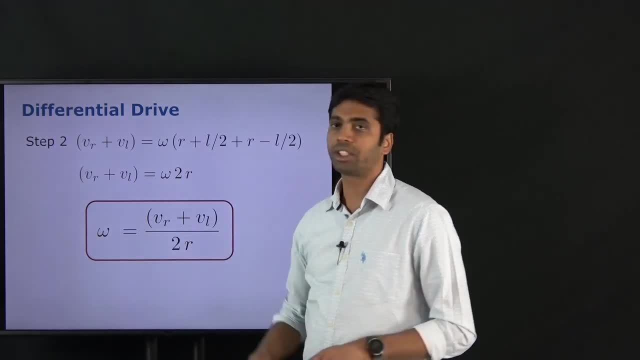 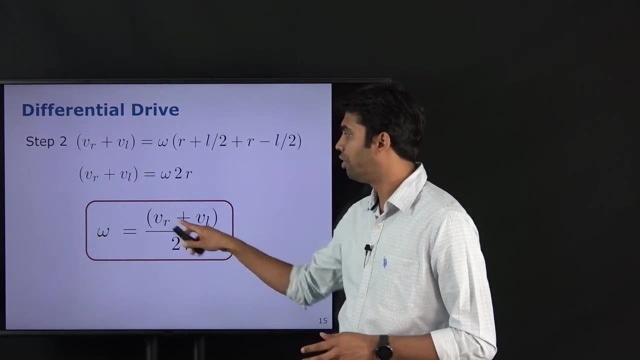 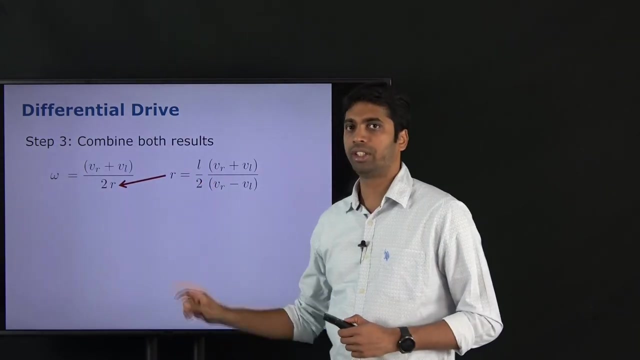 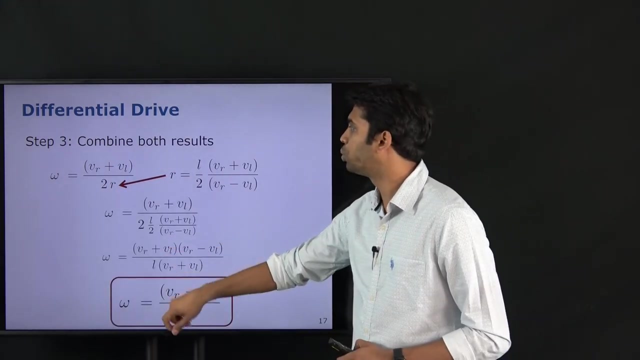 So we have an expression for the angular velocity of the whole platform in terms of the individual velocities of the wheels and the radius of curvature. Since we had just computed the radius of curvature, we replace it into this equation and we will end up with an equation like this, which where we will have basically these terms. 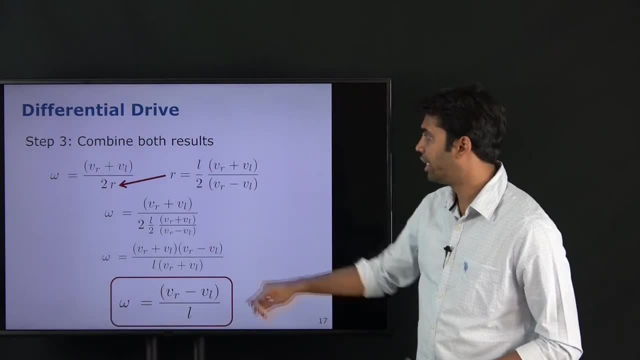 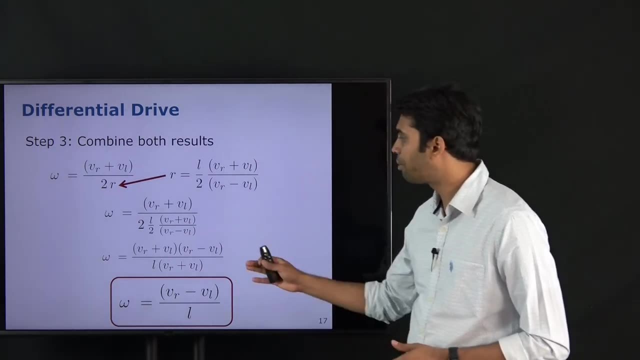 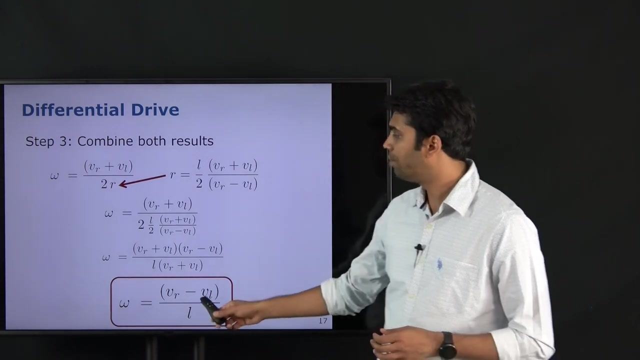 sitting in here And if you look at this equation, we can see that we can cross over some terms and, with a little bit of manipulation, what you end up is now, again equation for the omega. So which is the angular velocity of the platform, in terms of, either, the velocities that have 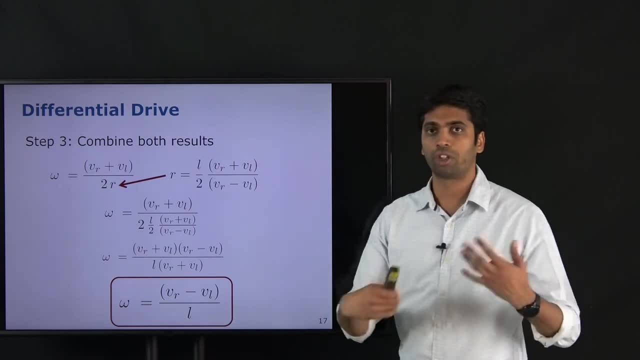 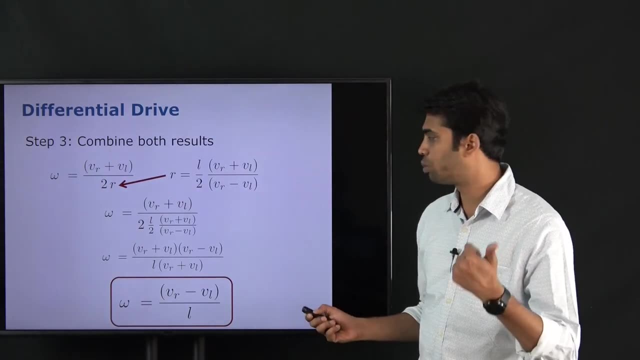 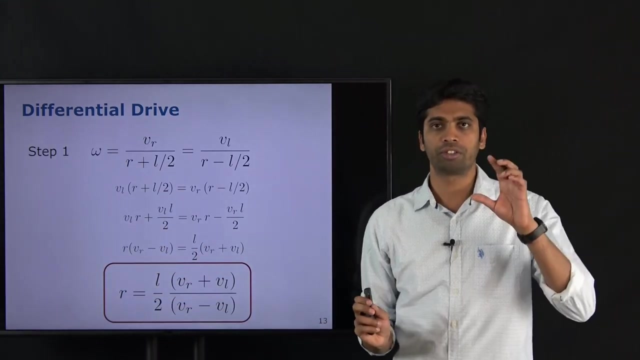 been set to individual wheels or some parameter of the robot itself, So in this case, the length between the two wheels that we have. So we have. we have done two things. One, we have expressed the radius of the curve or the radius of the curvature, for the curvature which the robot is. 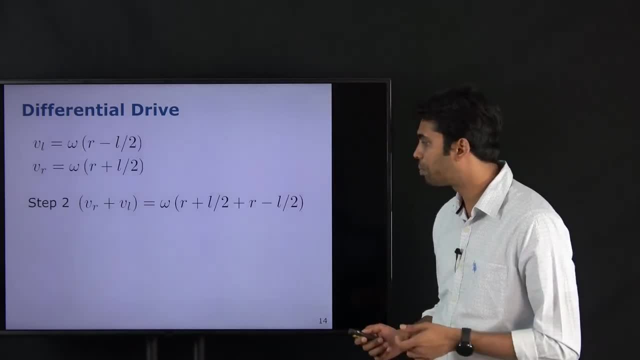 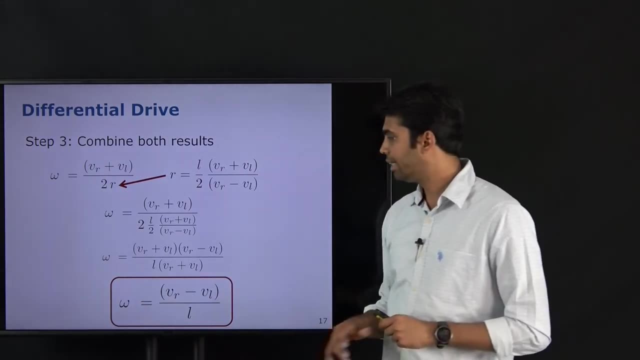 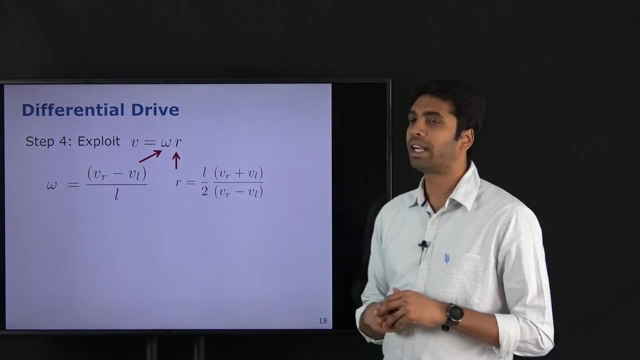 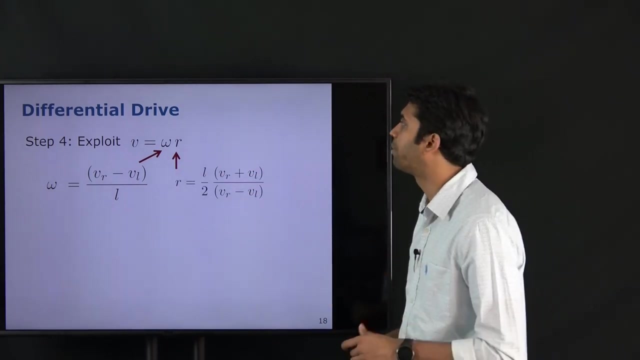 going to follow in terms of these parameters. We have also expressed the angular velocity in terms of the two velocities of left and right wheels, as we see here. What we can then do is also find out an expression for the linear velocity by replacing these two things that we had computed in step 2 and step 3.. So step 2: I. 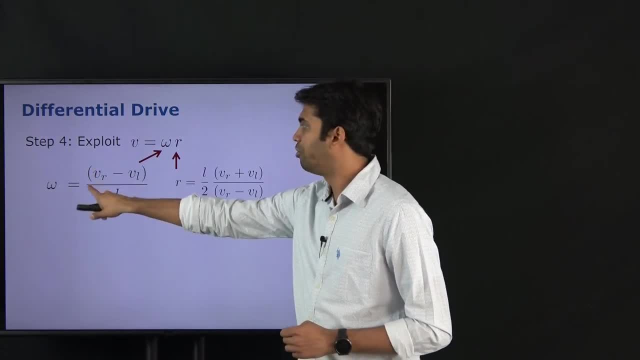 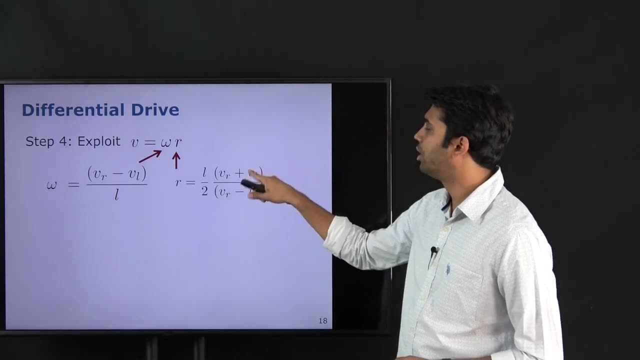 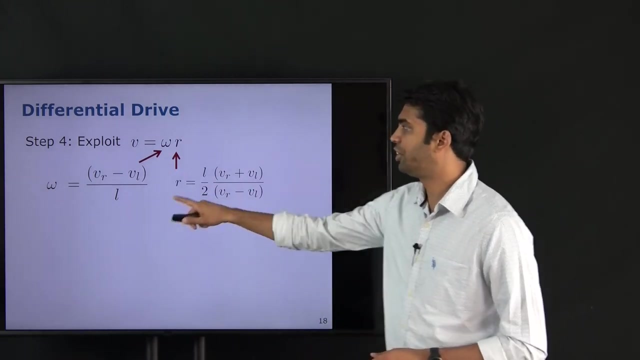 think gave us the angular velocity as vr minus vl by l and r was nothing but l over 2 times the right velocity plus the left, one whole divided by the right velocity minus the left one. And if we just replace these through two equations here, what we would end up is the 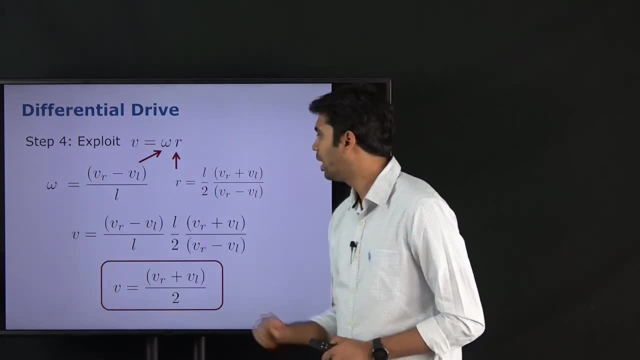 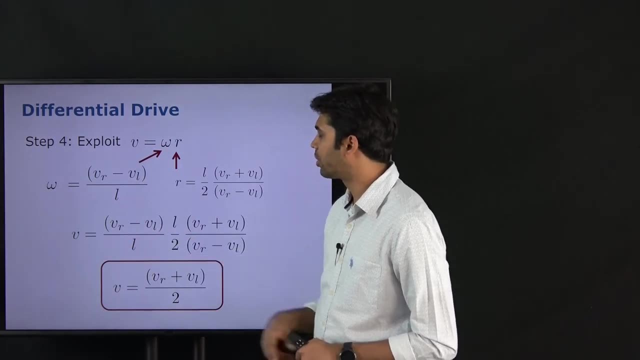 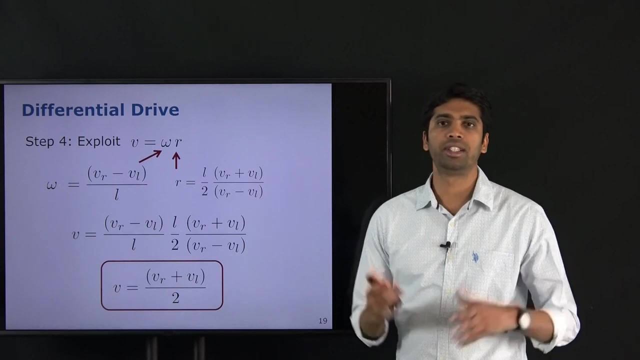 linear velocity is this expression here, and here we see that these two terms are the same, which we can cross out, the else cross out. Essentially, what we end up is that the linear velocity is nothing but the average of the left and the right velocity, and this also makes sense intuitively. 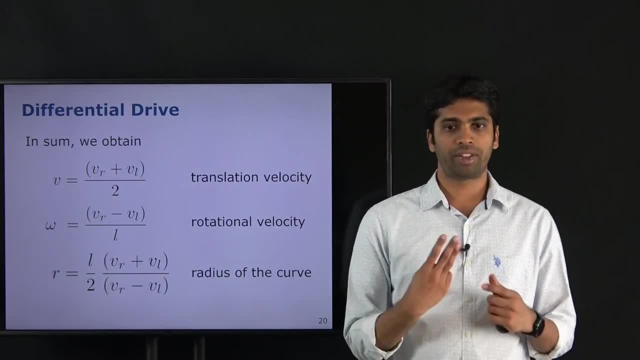 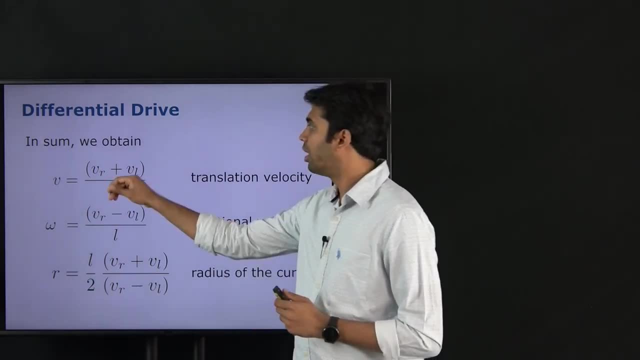 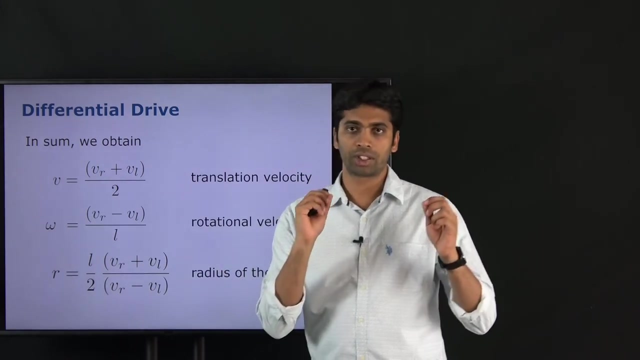 And so what we have now are three things. One, we know what the, how the, the complete platform moves with respect to the left and the right velocities that we put on to these two wheels. We know what's the angular velocity of the robot is. 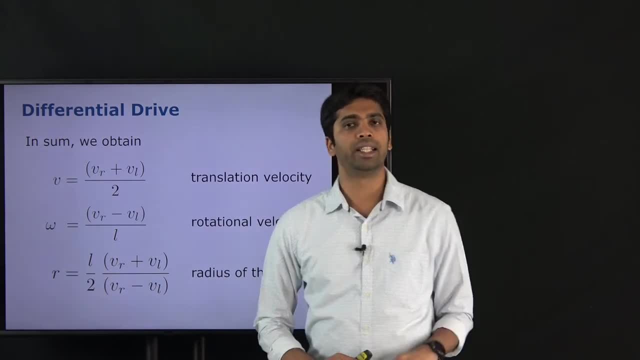 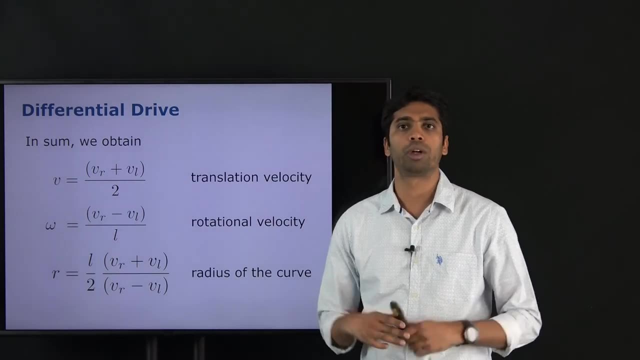 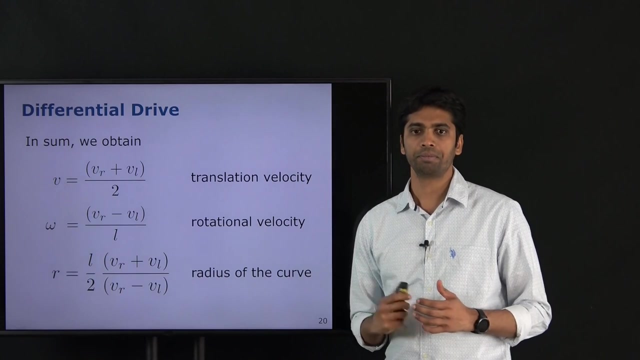 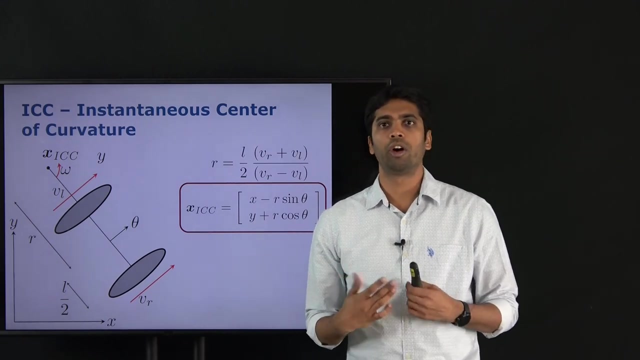 and we also know the radius of the curve that the that this robot travels along. So these are the important terms that we require in order to understand how this differential robot moves when a particular velocity is applied to the left and the right wheels. With this we can also compute the coordinates, for example, of the instantaneous center of curvature. 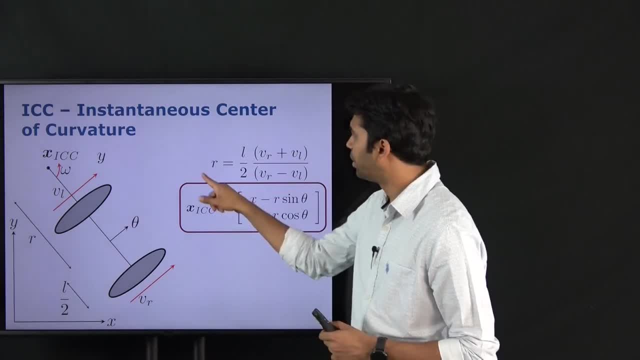 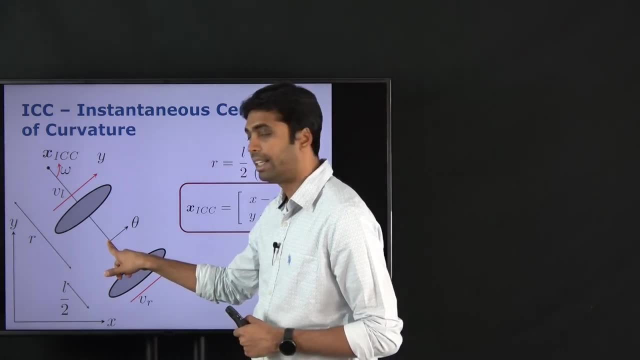 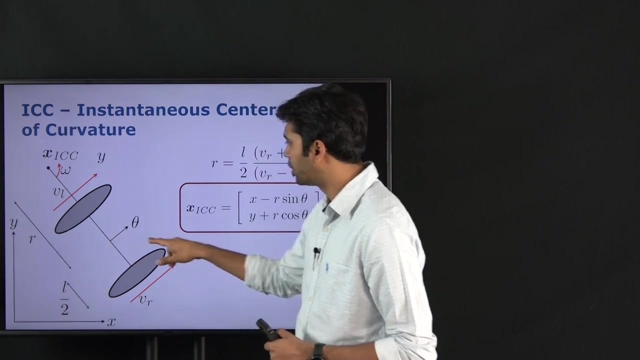 So we've had the, the radius which is given by this particular term here, and then we know that if the position of the robot is set here to x and y and then some amount of trigonometry, So it makes an angle of theta with the positive x-axis. So essentially this particular 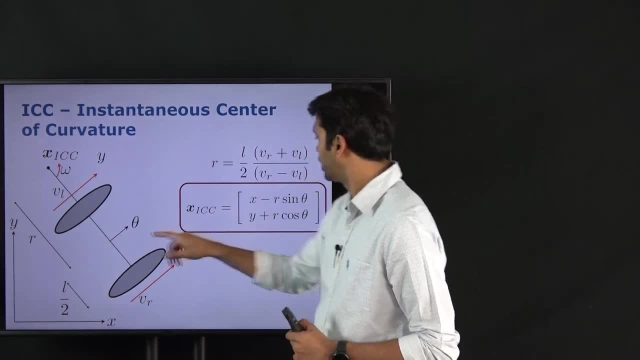 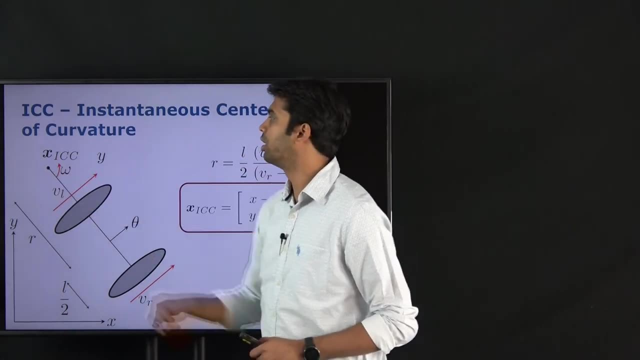 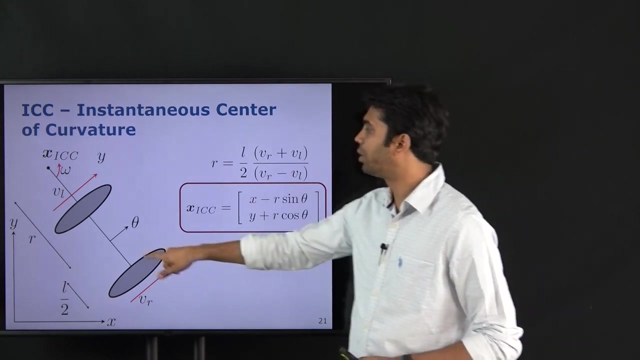 coordinate would be nothing but the position of this, which is x minus the r times of sinus. of that theta would give us this particular coordinate and, similarly, to get the y coordinate, it would be a cosine of theta which needs to be added to the position of that, of that point itself. 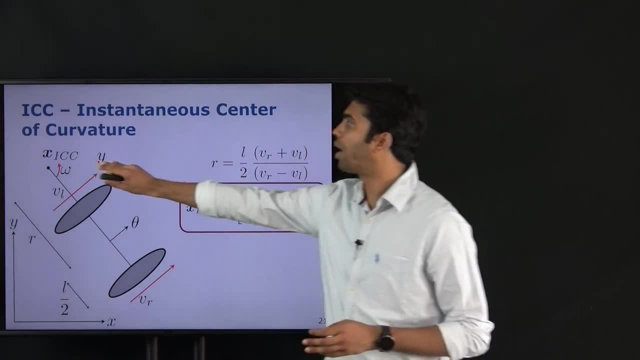 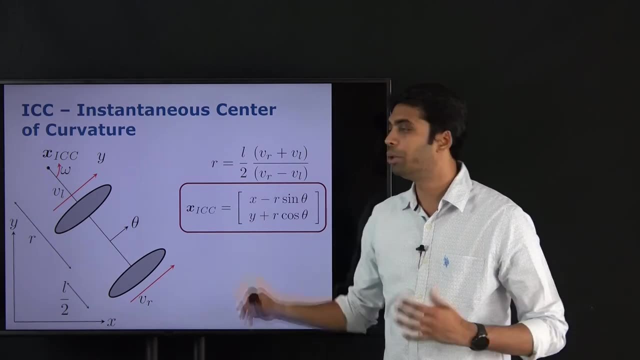 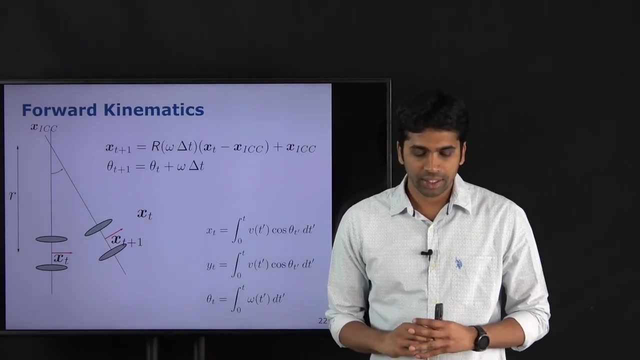 So what we are now able to express is the coordinates of the instantaneous center of curvature in a global coordinate frame using the radius of curvature that we just computed now. Next, what we are really interested is to infer how the platform is going to move. So, for example, 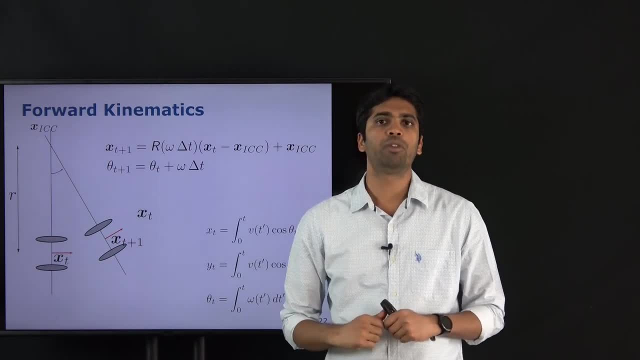 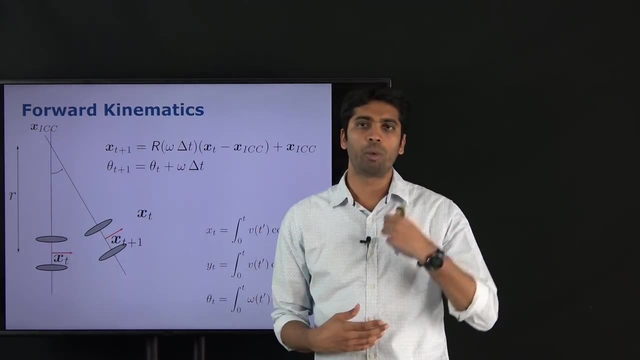 we know where the platform is at time t and we want to understand where the platform would be at time t plus 1, and this is also called as forward kinematics. So, given the velocities, whatever vl and vr to the two, and this is also called as forward kinematics. So, given the velocities, whatever vl and vr to the two, 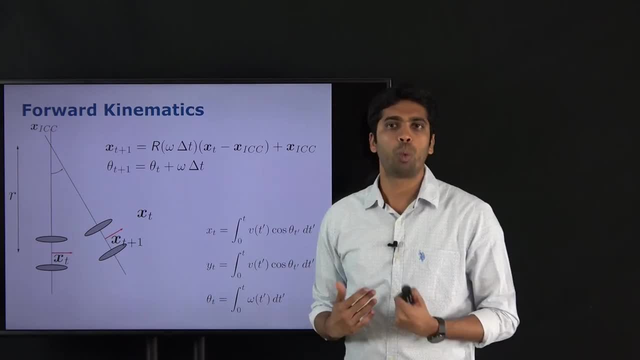 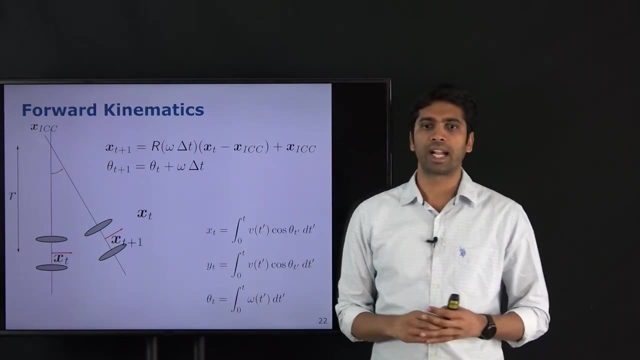 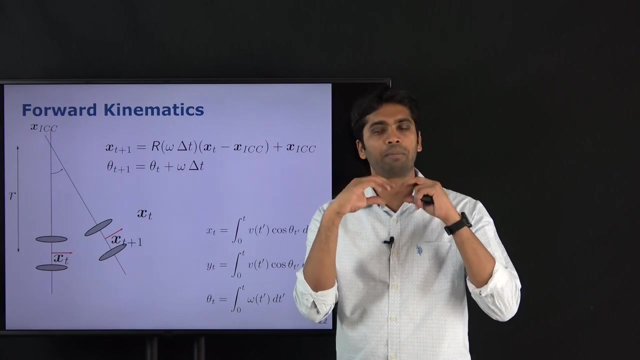 two wheels, where would we end up after one particular time step? So what we see here is a, let us say, a discrete format of understanding this. So, for example, for a time period of delta t, we put our, or we, we apply a constant velocity to our platform, So a constant rotational and. 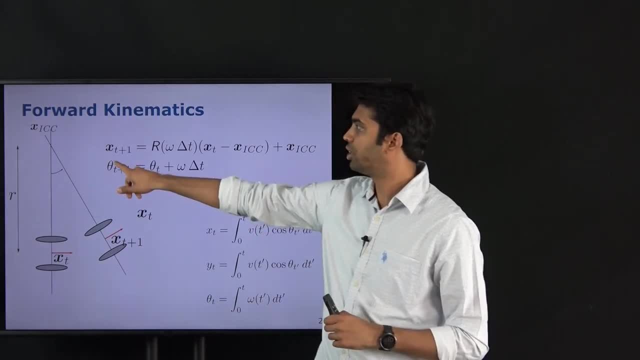 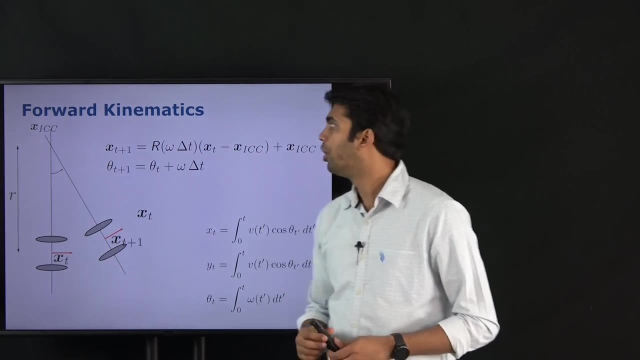 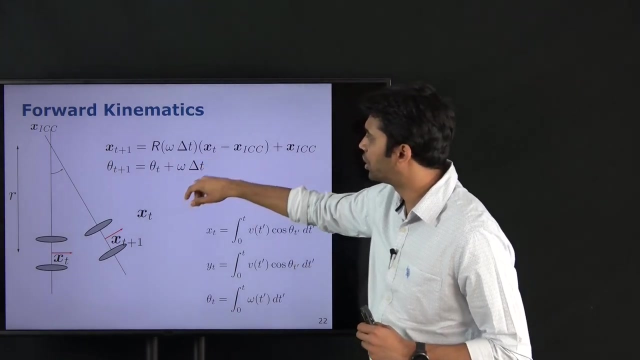 a linear velocity of the platform, the new position, So in this case, x refers to the, the position, So the location, x and y, whereas theta refers to the orientation of the rubber and essentially this depends on the, on on where it is. So what you need to do is to, is to take where you are, so this: 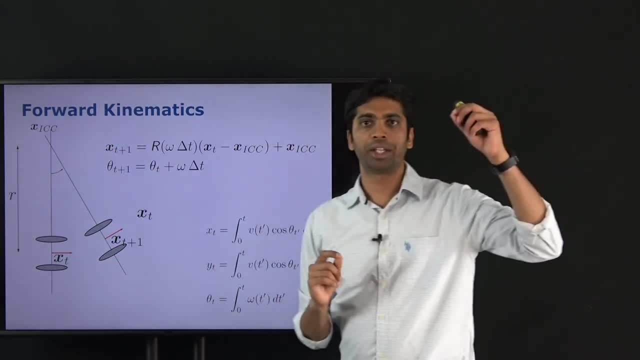 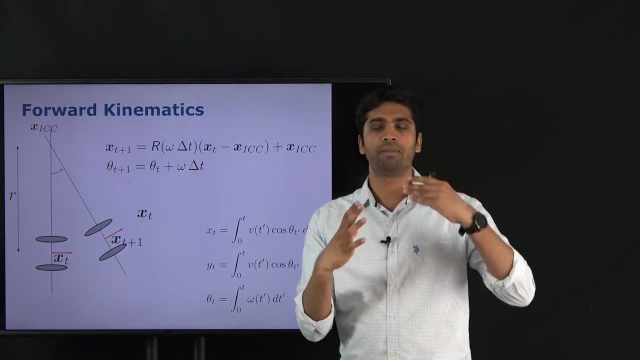 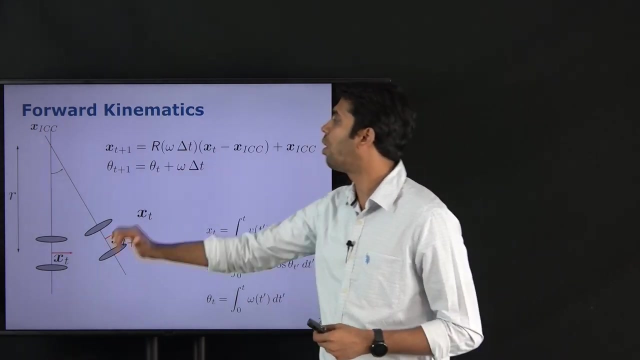 is x, t and subtract the coordinates of where your instantaneous center of rotation is, So this gives us x, t minus x, i, c, c, and then, when we multiply it with the rotation matrix, so this r of omega t corresponds to the rotation matrix, matrix which is defined along an axis which is perpendicular to the plane. here, 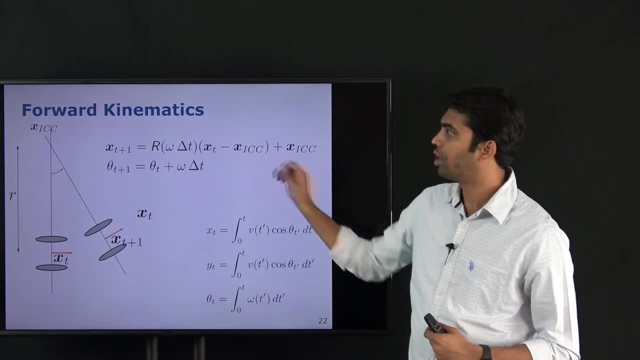 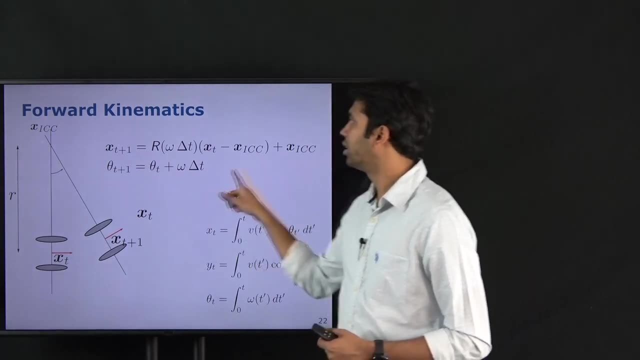 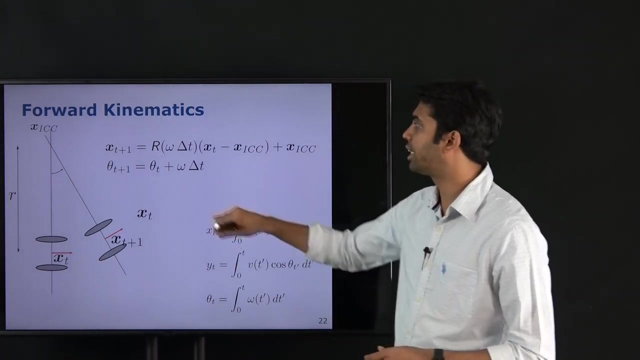 This way we would get the new position of the robot. So we have to take the x, i, c, c and add it to this difference vector that we have just computed. Similarly, we can also compute the new orientation as nothing but the old orientation plus the angular velocity. 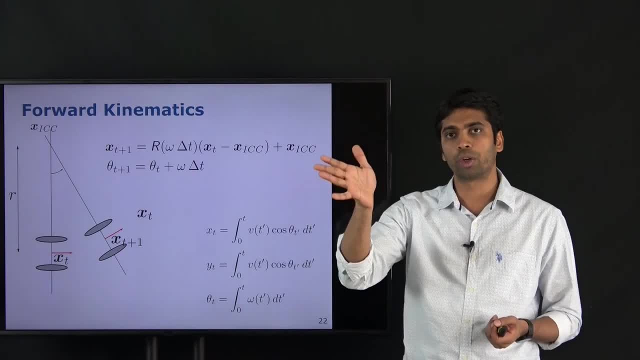 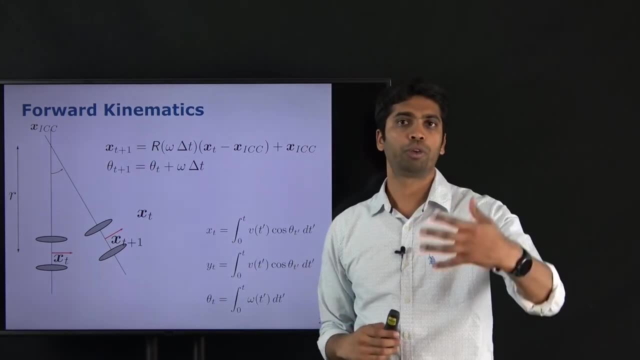 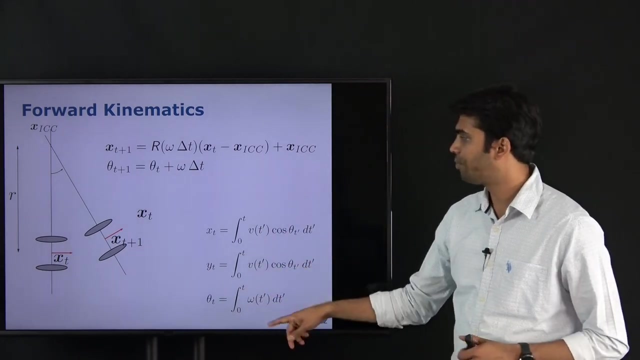 times delta t, because this is the amount that the robot has rotated in the meanwhile. So this is a way to understand how the robot would move over time, And in this case it is a discrete formulation, whereas here it is the same idea but as a continuous formulation. 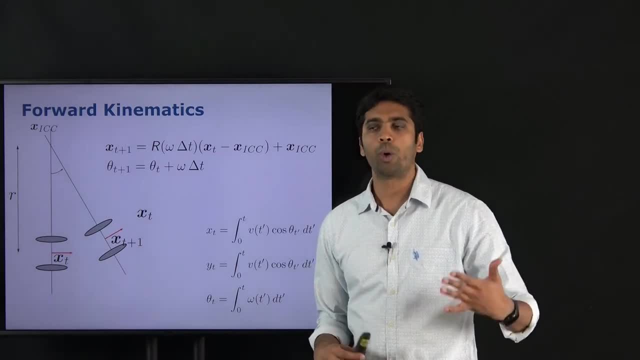 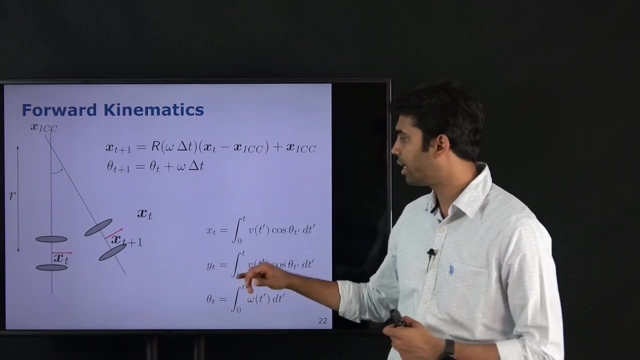 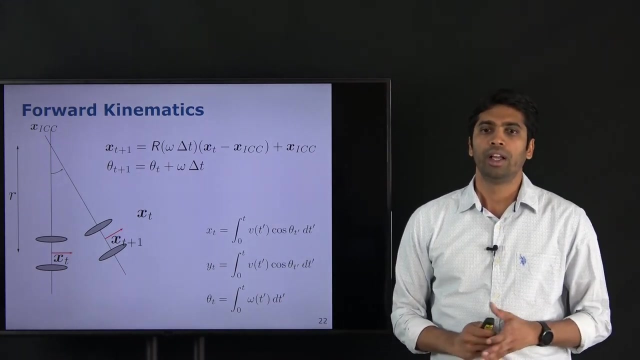 So this is what actually happens in reality. So you do not have constant velocities per se, but rather following a trajectory or a profile of velocities, and there we would end up integrating instead of just adding, like we saw here. Okay, so the next rubber that we actually see here is quite similar to: 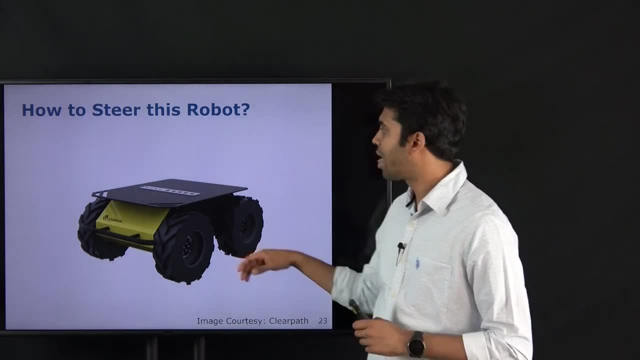 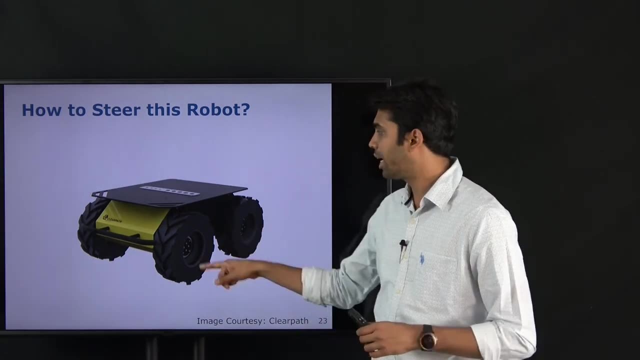 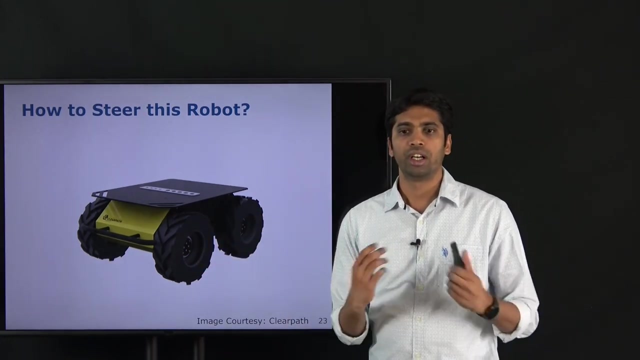 the differential rubber that we saw before, in the sense that these wheels, both in the front and the back, are attached with a fixed axle. You can control the the velocities of, let's say, the front wheels and the back wheels separately, but they are attached rigidly. So in some sense it's similar to 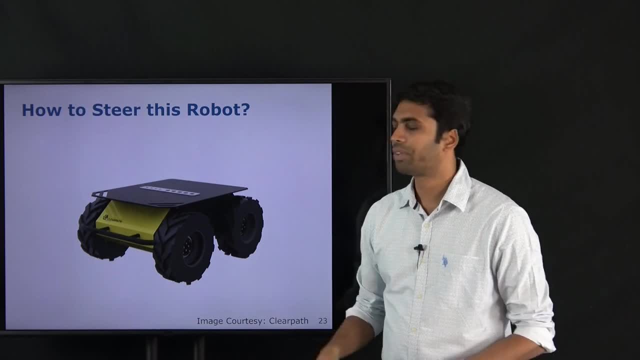 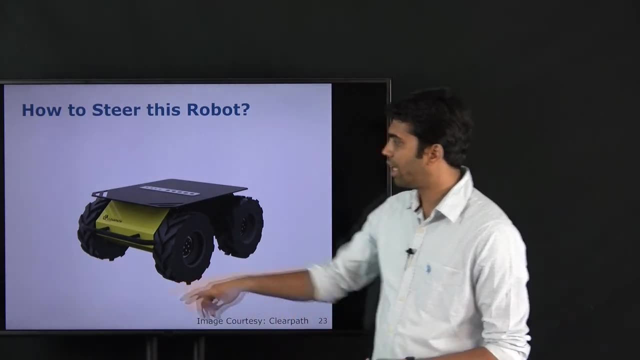 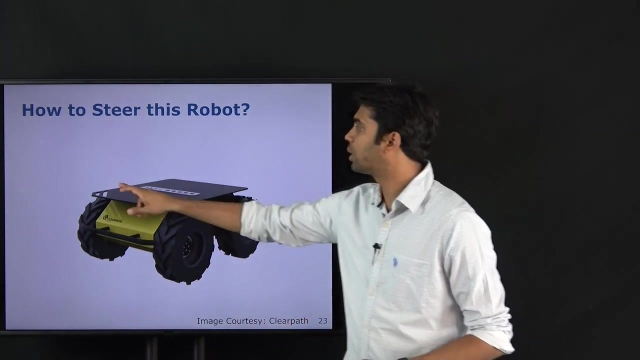 differential drive. but if we look carefully, there's a flaw, so to say, in the kinematic design of this robot itself, because if you think, there's an axis which is going through the front, a front pair of wheels, and there's also an axis which is going through the back pair of wheels, and since they're attached, 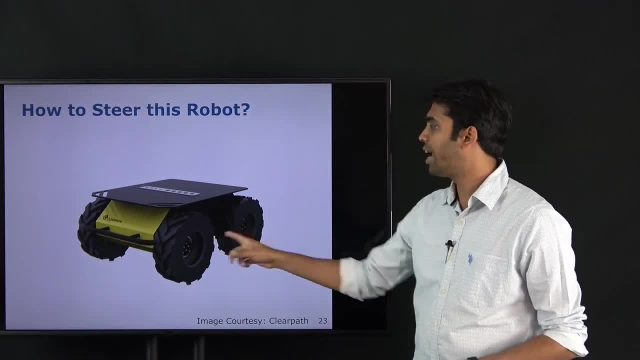 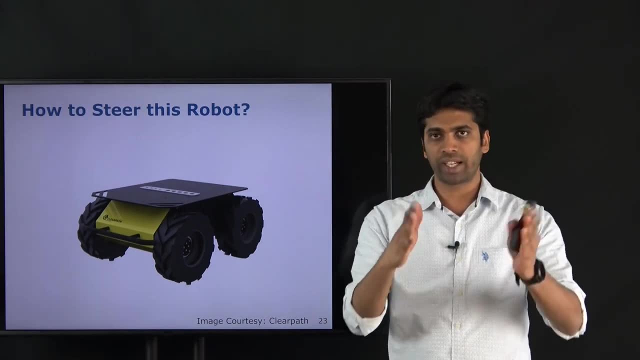 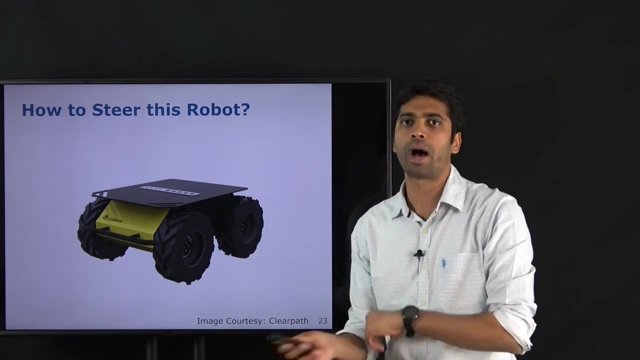 rigidly parallel to each other, there is no way that those two axes will ever meet. So, of course, if you just want to move straight, it's fine, they're parallel. you apply the same velocities to all the wheels and that, and then you go straight, either forward or backward. However, as 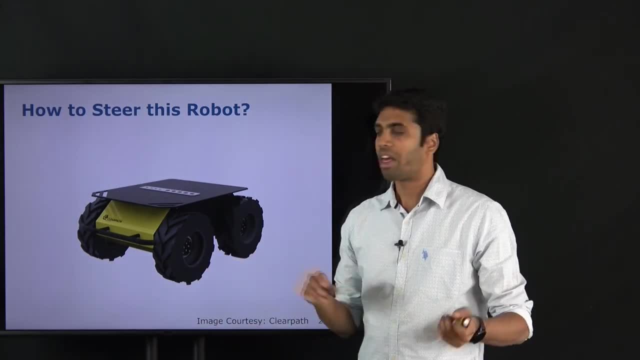 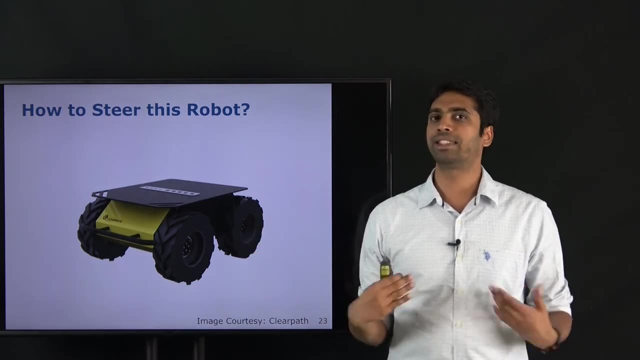 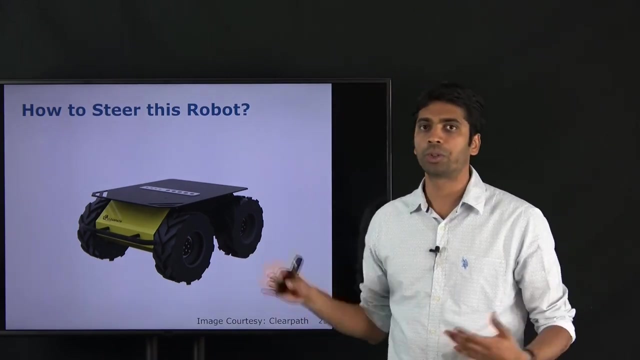 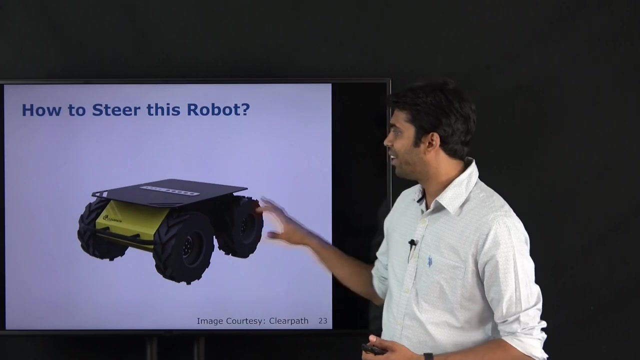 soon as we have to make any turn, then this means that since these two axes can never intersect, this kind of robot will always skid. It's never possible to roll off robots, and therefore sometimes these kind of control or to control these robots are also called as skid steer robots, So they're not very elegant in. 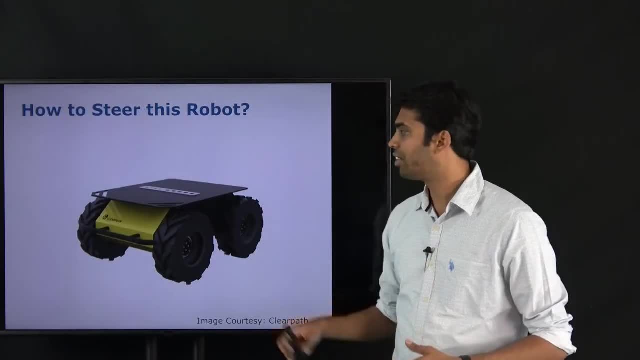 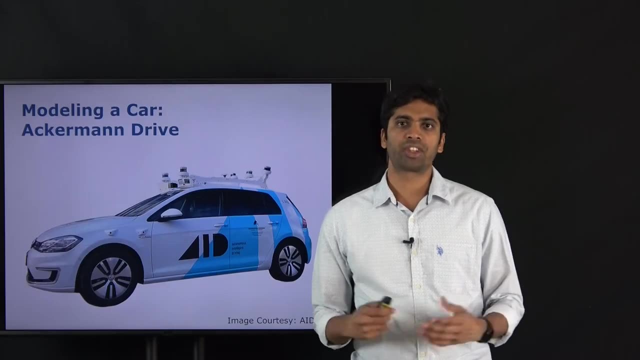 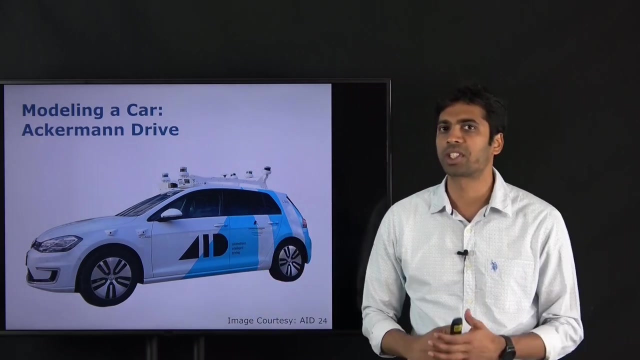 terms of kinematics, but it so happens that they're quite sturdy and they're often used in outdoor environments for navigation. The next drive that we look at is what is called as the Ackermann drive, So this is the typical car. in this case it's an autonomous car, but 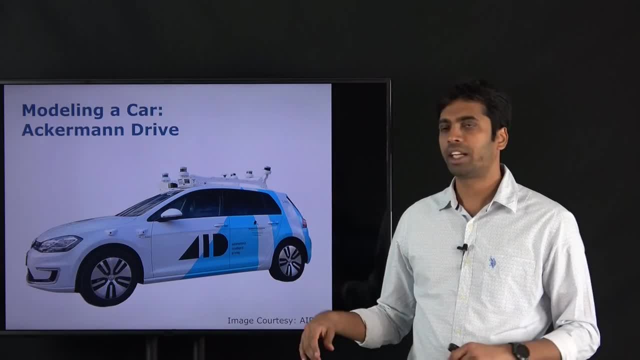 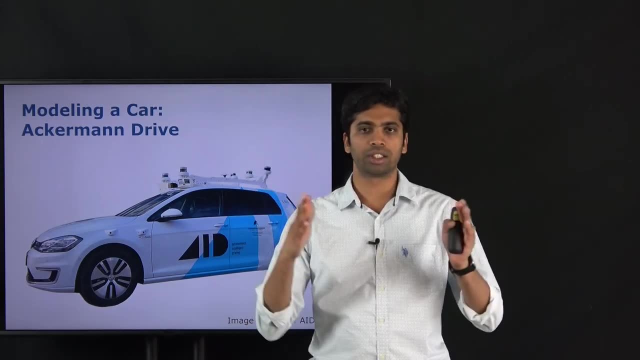 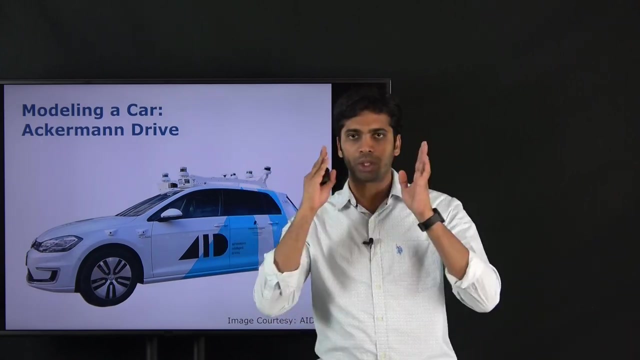 just a car, yet the same. and for these kind of cars, what you would have is that the back wheels would be usually fixed and the front wheels are steerable. So in this case, essentially what would happen is, if you want to go straight, of course, the same idea, put the same velocities on all the four wheels, and then you go. 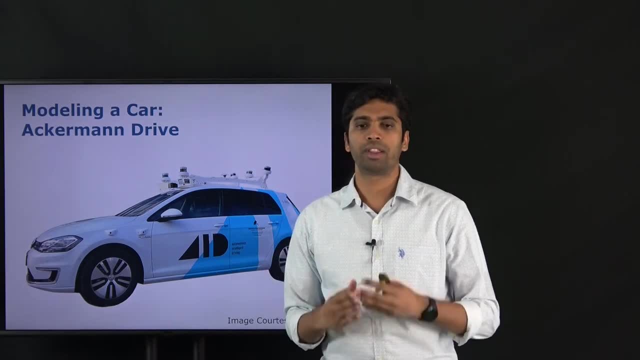 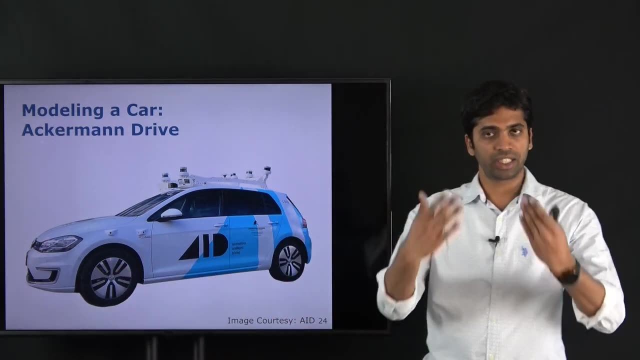 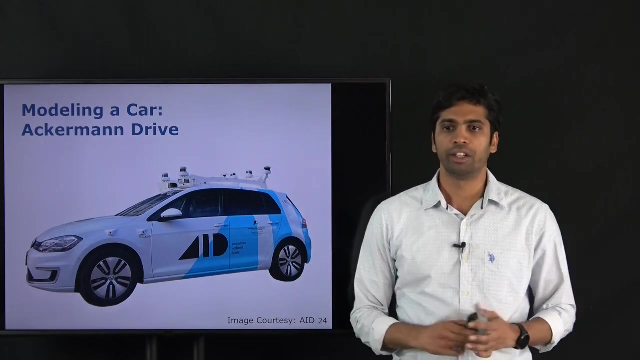 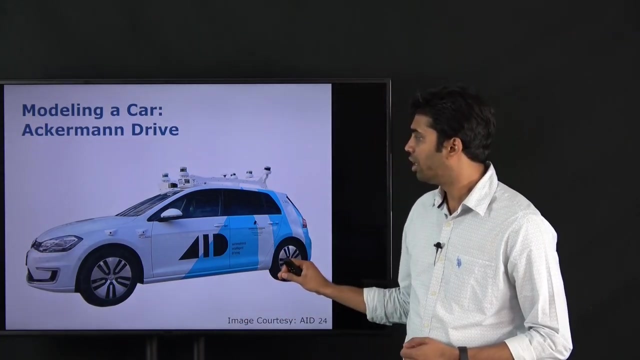 straight. But if you want to turn, the idea would be then to turn the wheels such that you obtain a instantaneous center of curvature by intersecting the back wheel axis and the front one. So, since this is an Ackermann kind of drive, the kind of 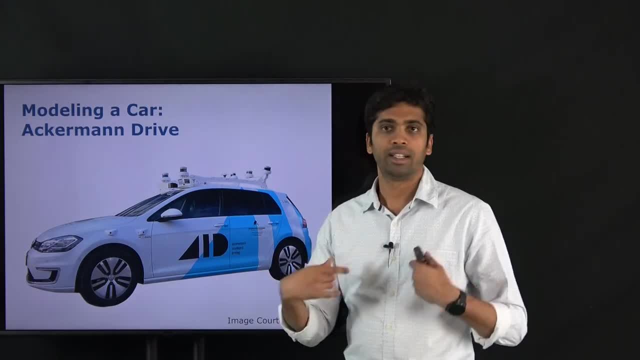 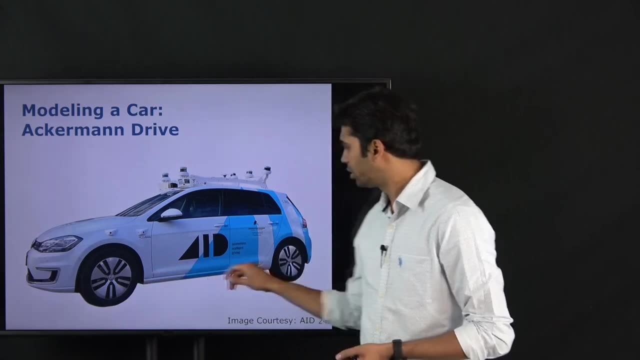 maneuvers that it can do are restricted. For example, like a differential drive, it can't really rotate on spot because at the least there is this distance or this difference between the back wheel and the front wheel. So this is the kind of example where you have a car in which the car can rotate on spot, but the back 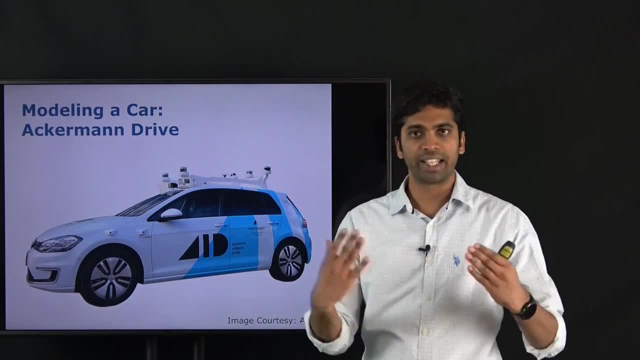 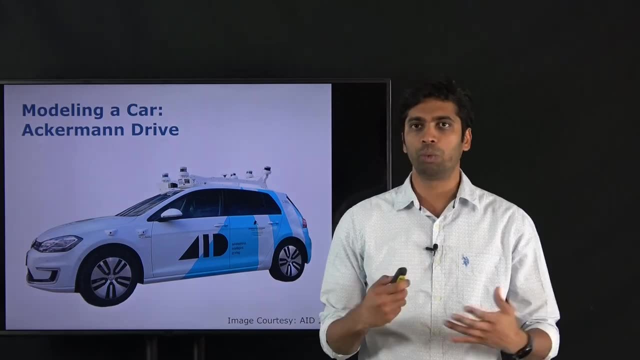 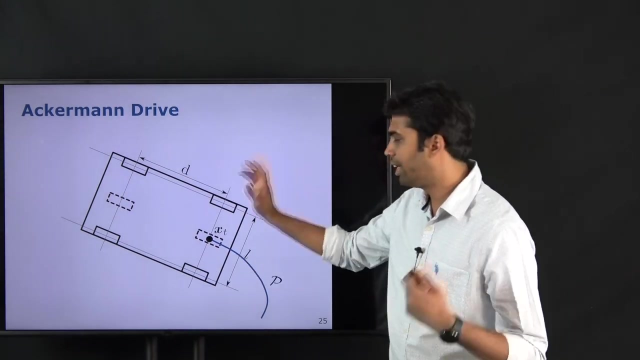 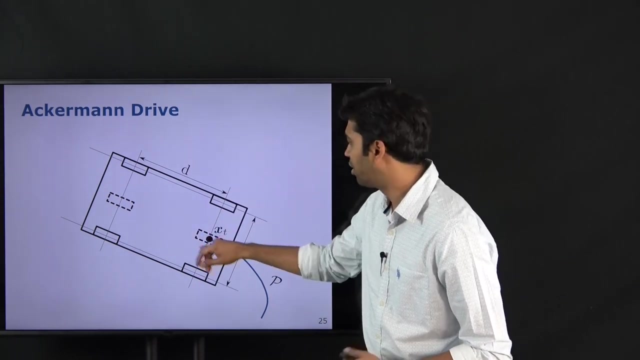 wheel and the front wheel, and therefore it can't make a non-zero radius turn, so to say. So let's look at how this Ackermann drive actually works. So to analyze this Ackermann drive, one usually approximates, or it's an assumption that one makes- instead of using the real back wheels, You take a virtual wheel, which 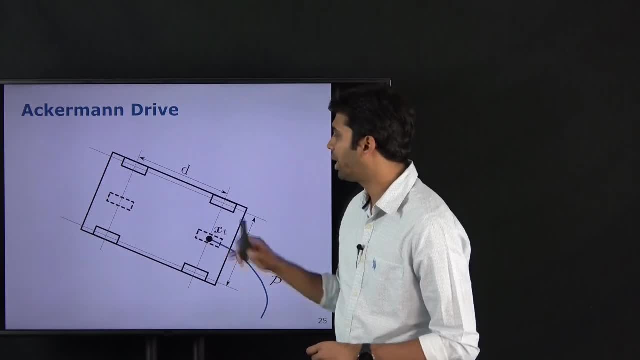 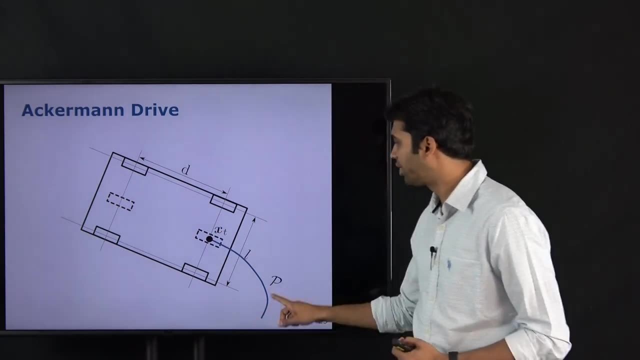 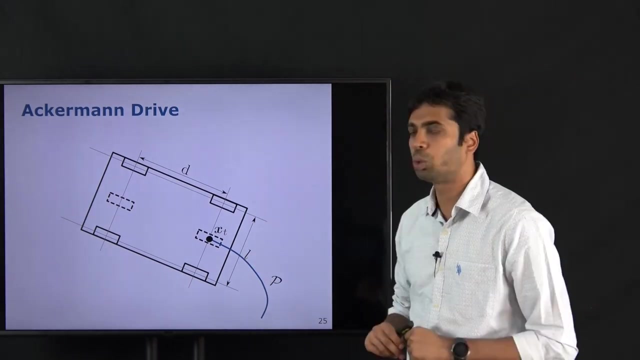 center of these axises, and this point would then be, so to say, would be the center of mass or the center of the vehicle which will follow the trajectory P. here, as shown here and again, we have these terms: L, which is the width between the two wheels, as well as this term D, which 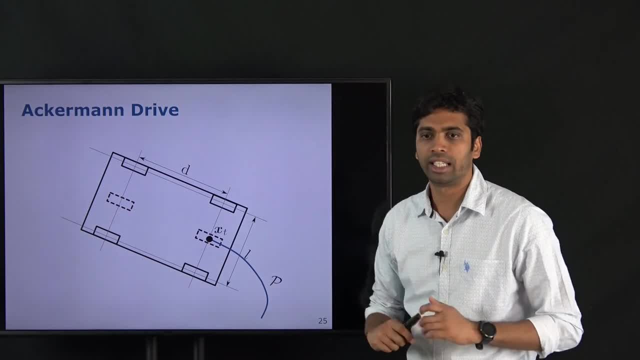 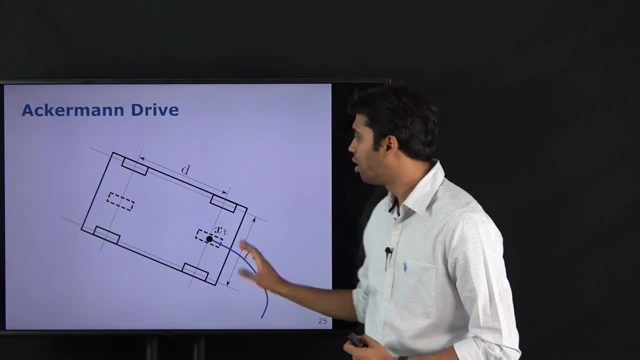 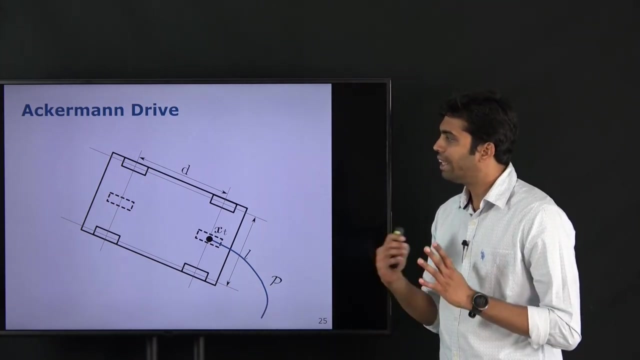 is the distance between the back wheel axis and the front wheel axis. So the goal would be to figure out how to make this particular robot follow a particular trajectory, shown here in blue here. So to make the analysis simple, one usually approximates this Ackermann drive to what? 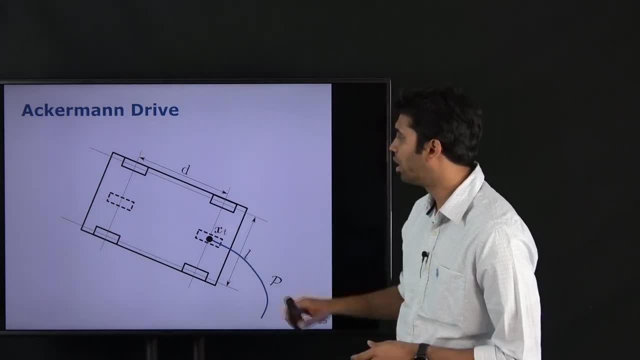 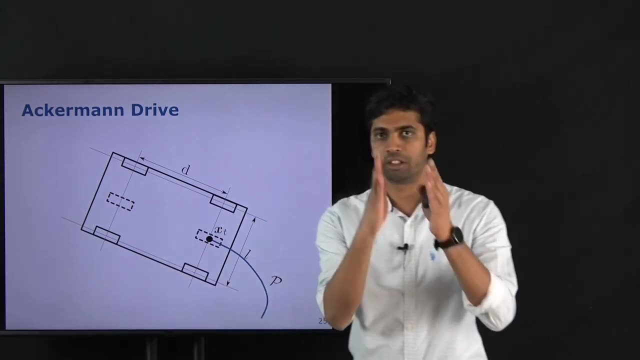 is called, or Ackermann model, to what is called as a bicycle model. So, in addition to this virtual wheel in the back, we also create, so to say, a virtual wheel in the front. Sometimes this wheel is also called as the ideal wheel. however, the difference is that 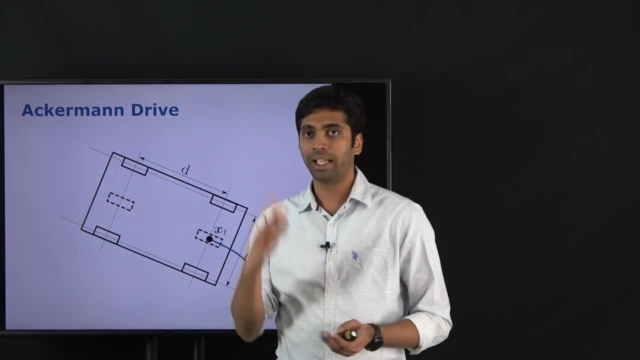 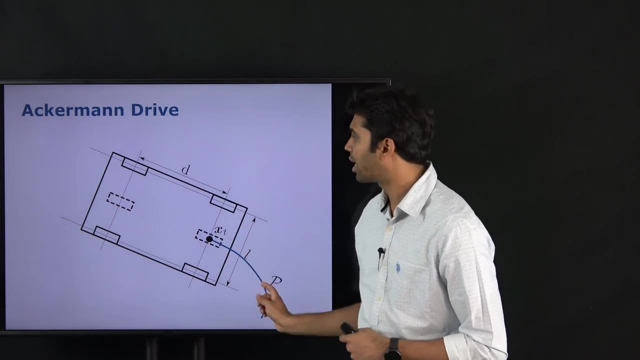 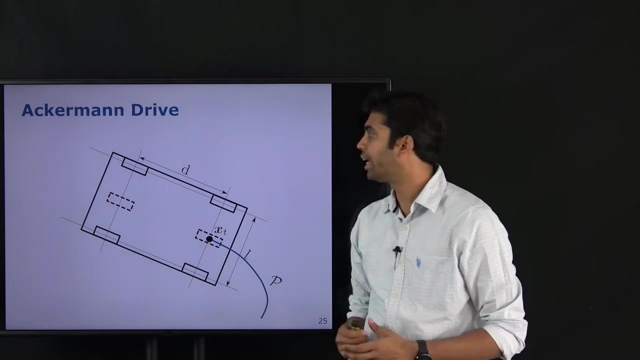 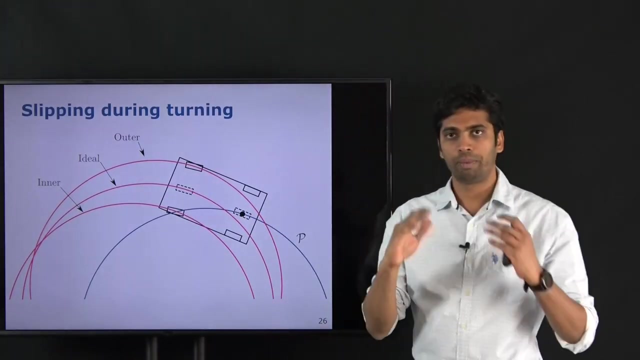 this wheel is fixed, whereas this front wheel is steerable, So you could think of this wheel moving at different steering angles in order to track a particular trajectory. So let's see how this would then result in a motion. So, for example, now let's say we want to follow a particular arc. 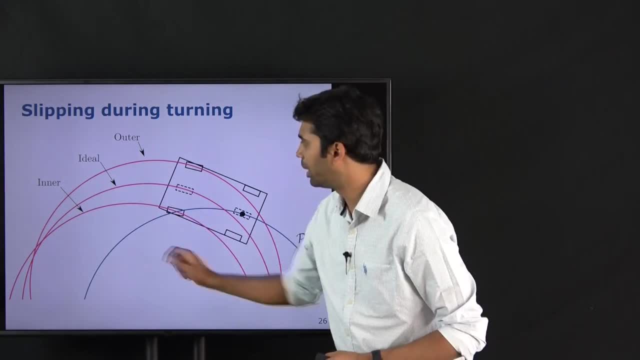 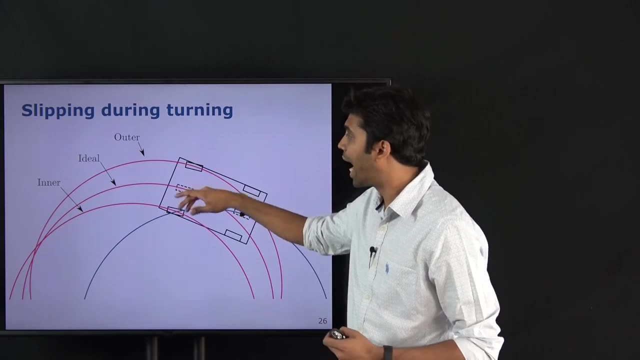 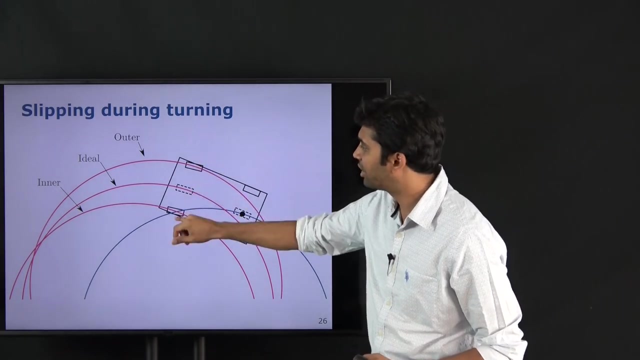 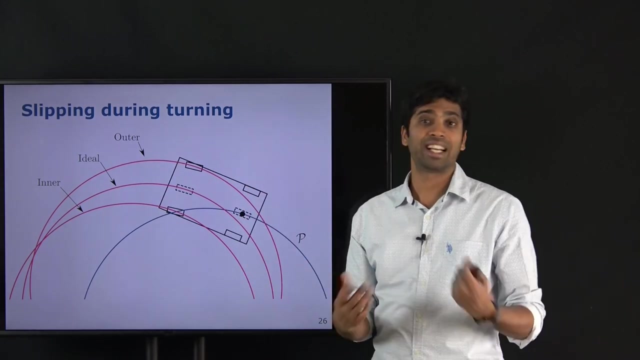 So a park which is for passing through this back wheel. However, if we put the same steering angle of our so-called ideal wheel on to the actual wheels that you see here, since there is some distance between these two front wheels, the circle along which that they are passing does not have the same radius anymore. 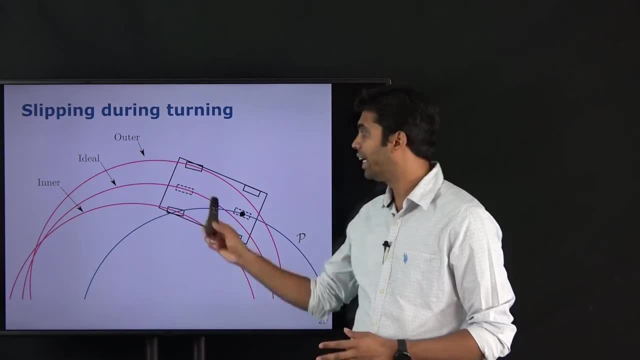 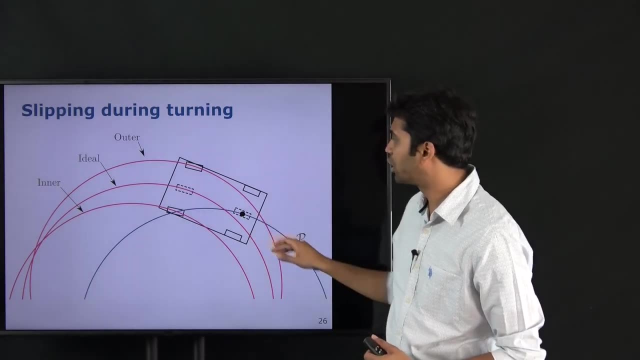 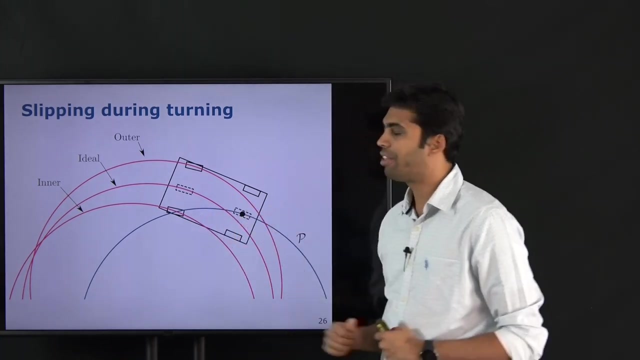 This means, then, that they are slipping, So each one of these front wheels is actually following a different curve, instead of the one that we actually follow, which we want to follow using these using this path P here. So, if you think about it, the answer to this would be, then, that the two front wheels cannot. 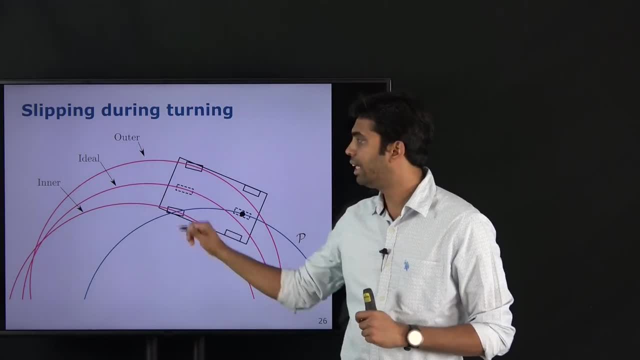 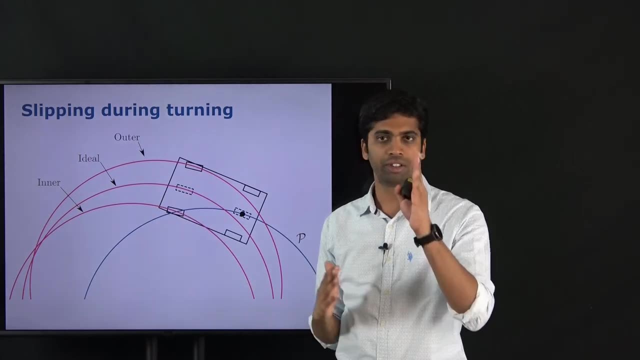 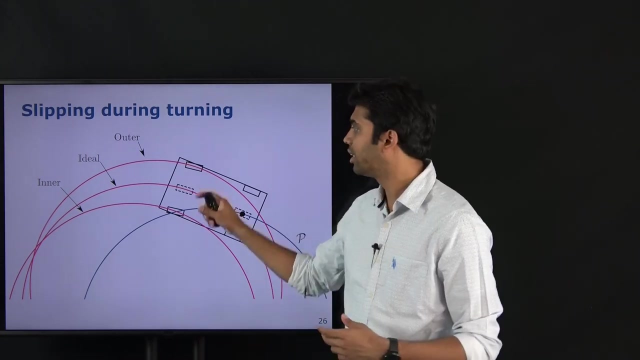 just steer at the same angle. they need to move or they need to be steered at different angles. The one which is towards the inside of the curve needs to steer less, whereas the one which is on the outside probably needs to steer more. In either case, we need to have different steering angles for the inside and the outside wheels. 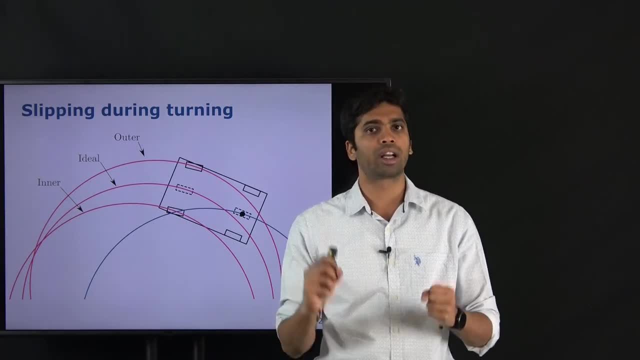 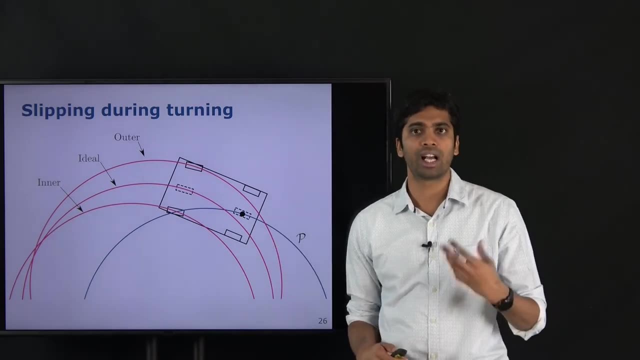 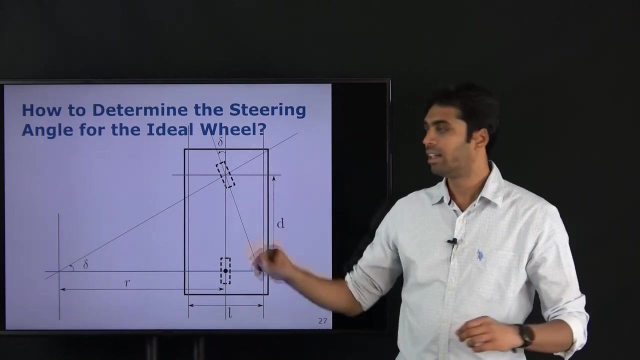 and actually this is what also happens when we actually steer our car in real life. So let's actually try to derive these equations and see how that looks like. So first let's do it for the ideal wheel itself, Although this wheel doesn't exist in reality. let's now, for assumptions sake, assume that 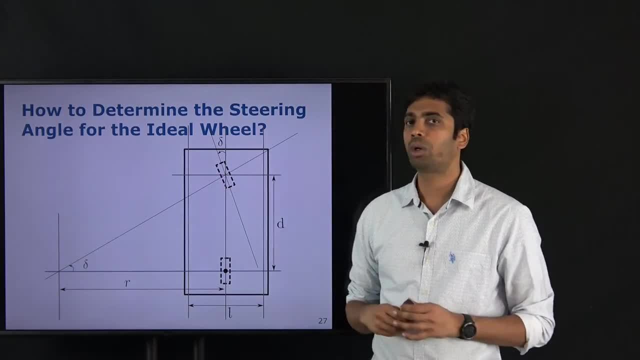 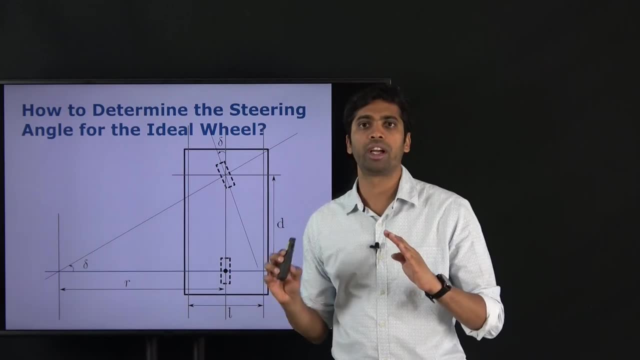 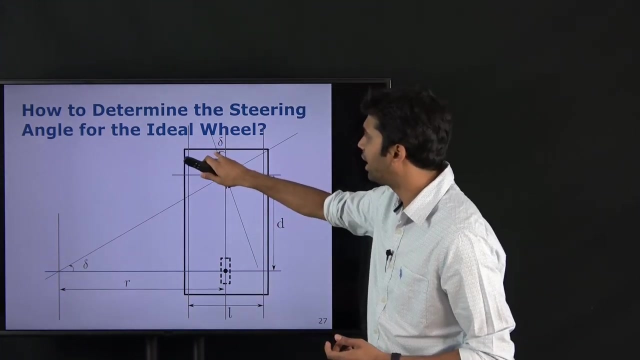 there is this ideal wheel and we want to figure out how much we should steer so that we have a instantaneous center of rotation and therefore we are rolling smoothly. So in this case, for example, we determine or we define this steering angle by delta and if we look at the right angles, 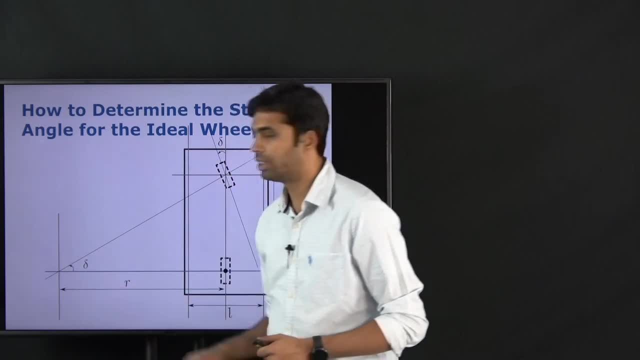 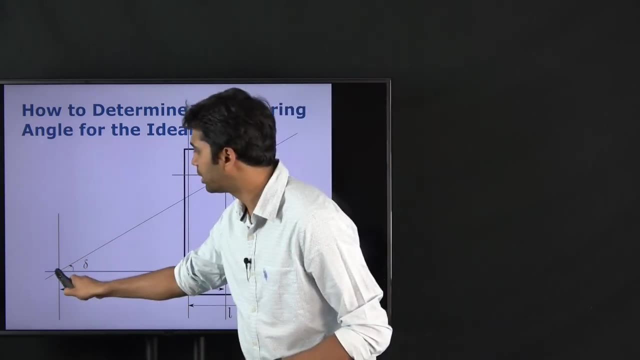 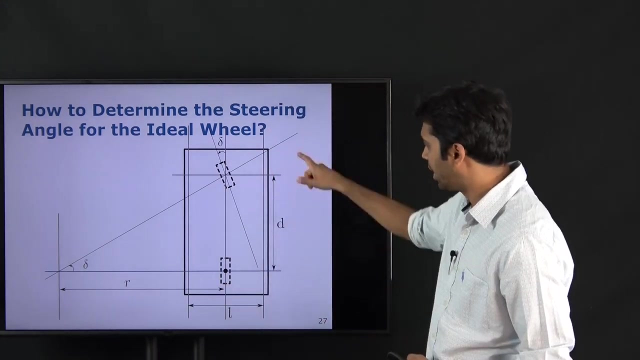 We would also come out that this angle here is delta. So what we see here is again: this is the center of the back wheel and this is the instantaneous center of curvature. So this R is basically this radius of that particular circle. We again have this D, which is the length between the two axis, and the L, which is the width. 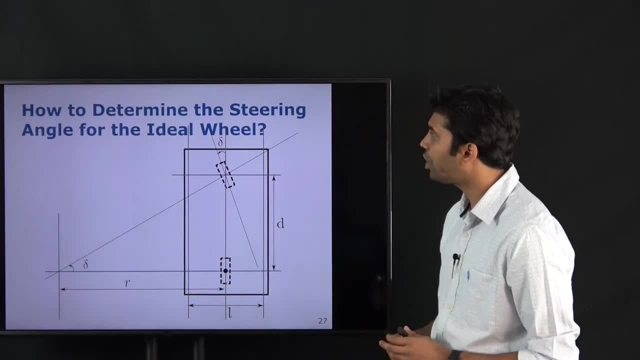 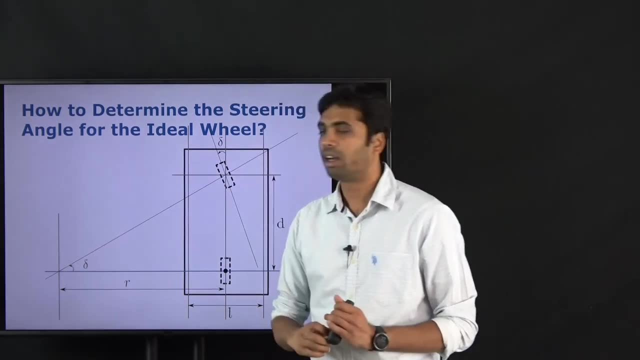 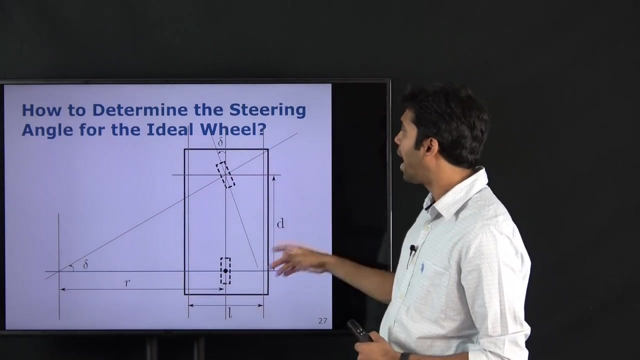 of the of the car itself. So the question that we now want to ask is: What should be this delta, such that it intersects at our instantaneous center of rotation? What is the relationship between delta and other geometric quantities that we see here, And actually this is quite straight forward- 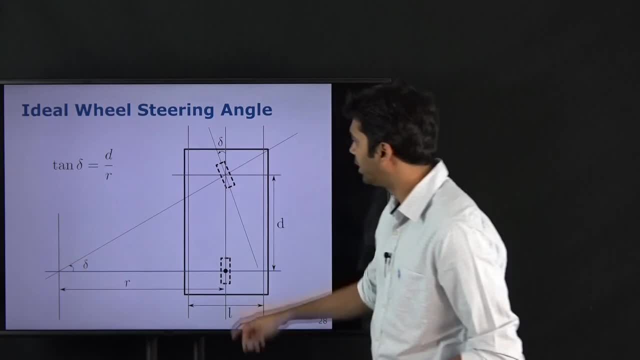 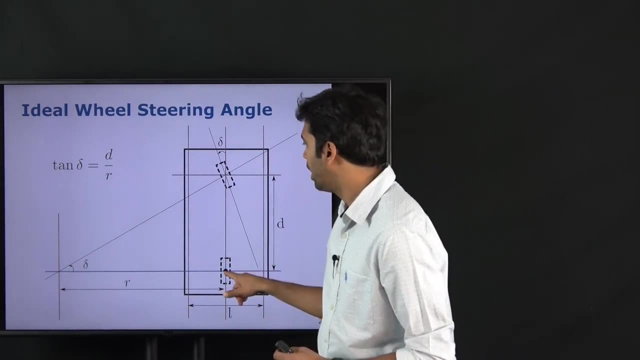 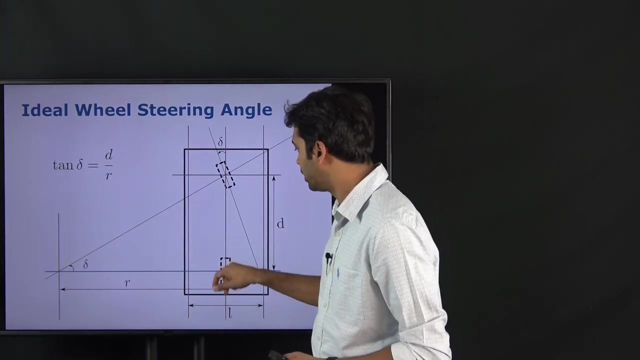 So, if you look at the tangent of this angle, delta, that is nothing but the opposite side here, which is D, which is the distance between the two axis and the, this particular distance here, Which is nothing but R. yeah, it's R because it's the distance from the center of our car. 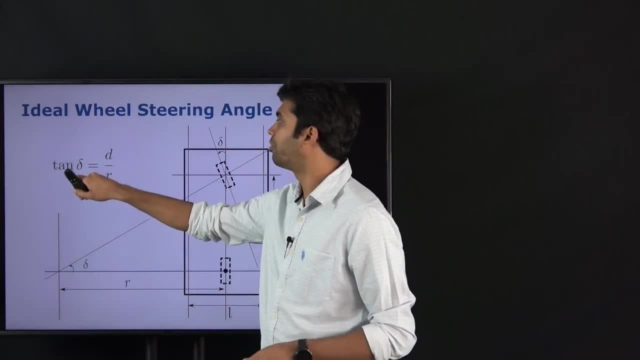 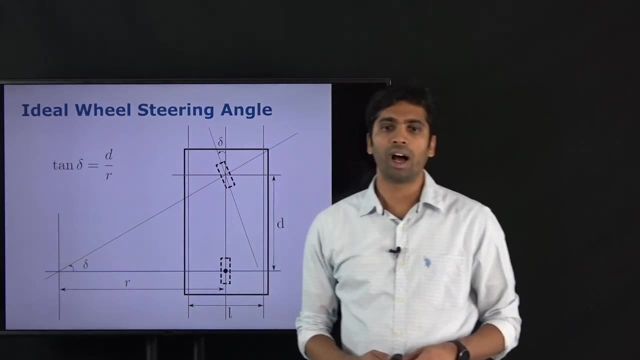 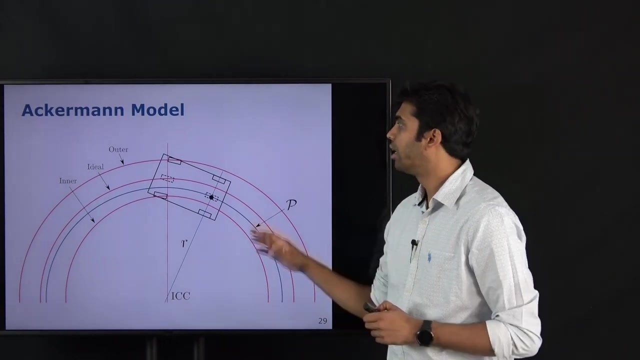 to the instantaneous center or location. So, basically, tan of delta is D over R, which means delta is nothing but arc tan of D over R. However, if we actually want a smooth motion for all the three, for the whole vehicle as a whole, Then it means that we need different circles. 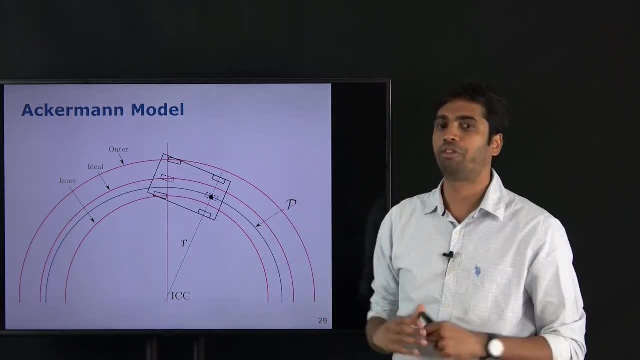 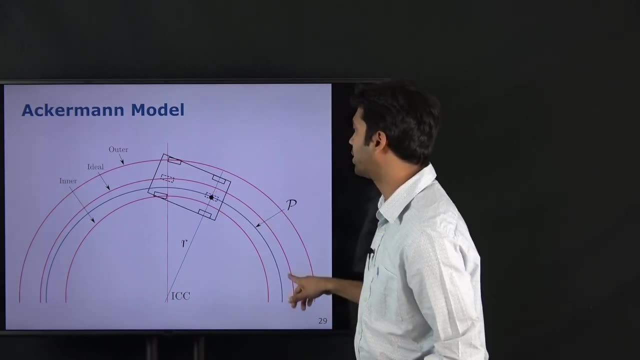 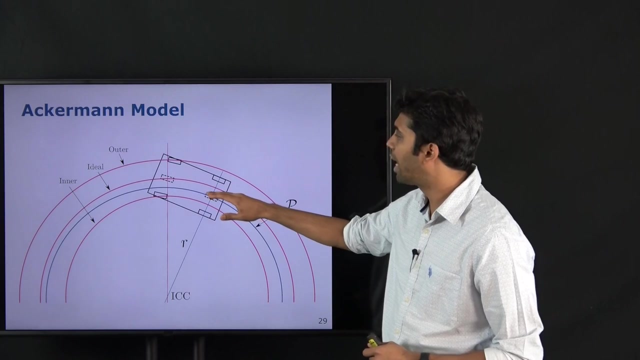 That the Inner and the outer wheel actually follow. So this is the path that we want to track, and also the path that the back wheel tracks can be slightly different from the one that the ideal wheel or the center front wheel tracks, And so by choosing the steering angles for the inner and the outer wheel such that they 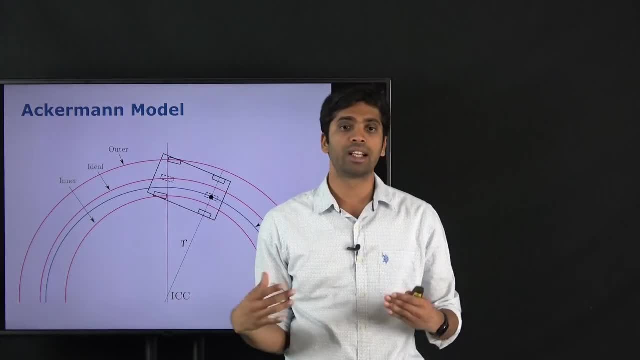 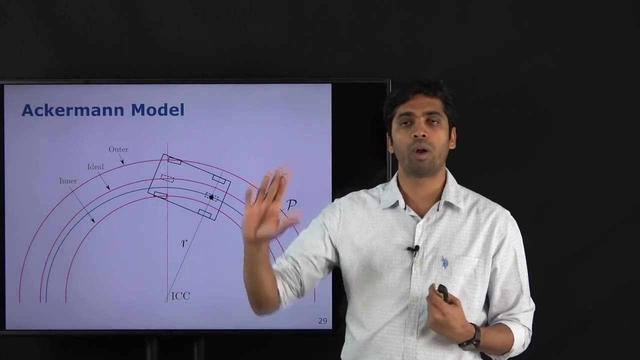 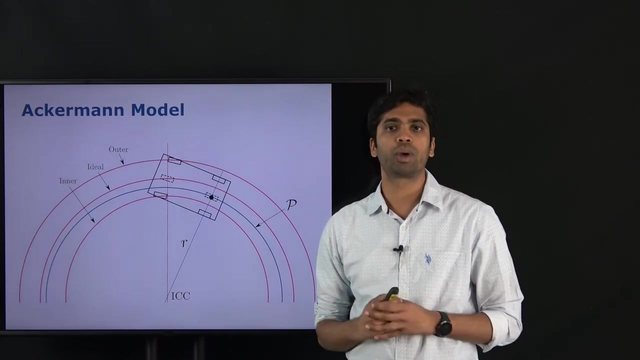 intersect at the same point as our ideal wheel does, Then we could come out with a formulation or a way In order to track our robot along the curved surfaces without any slipping. So it will be smooth, so to say. And so the question is: how do we actually figure out what these steering angles for? 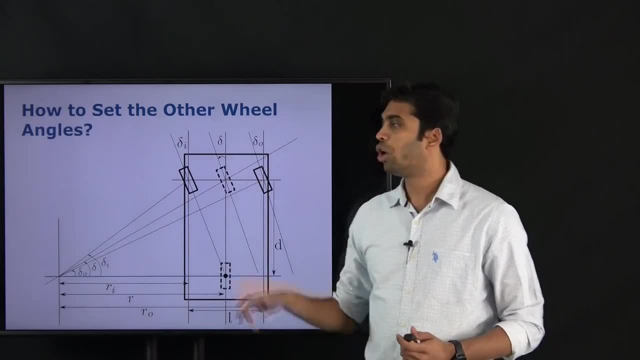 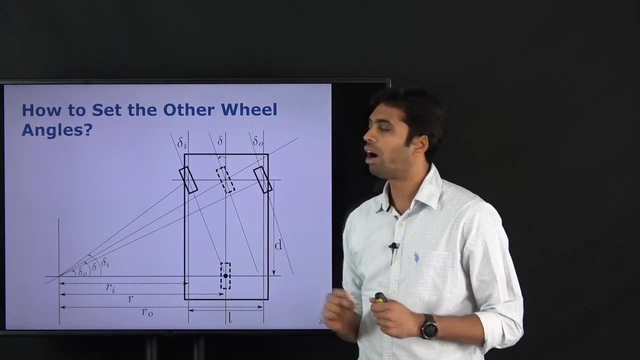 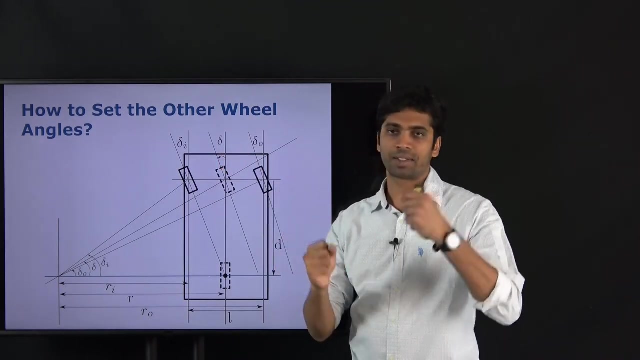 the two front wheels are. And so we go back to the similar diagram like we had before, where, if we move our steering wheel by delta, So we could think As this steering angle, as the amount of steering, for example, that we give on the steering wheel. 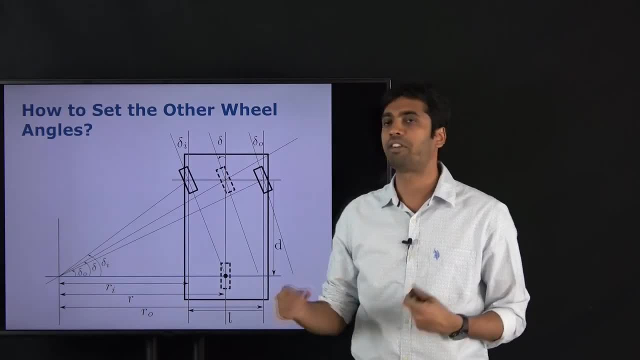 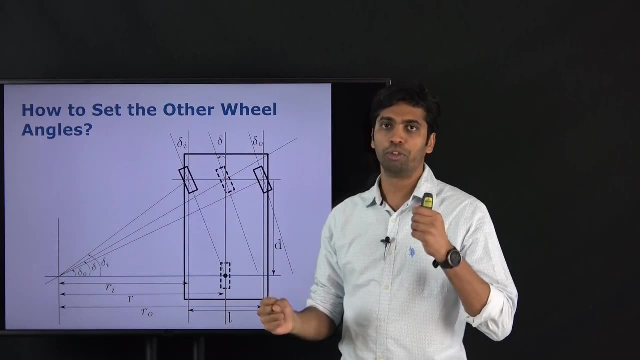 This need not be directly the case, that if you move your steering wheel five degrees, that the wheel also moves five degrees. But just for argument's sake let's assume that when you move your steering wheel by delta degrees, also the steering wheel moves by delta degrees. 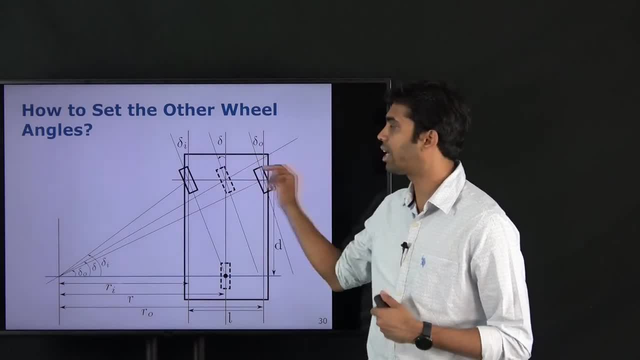 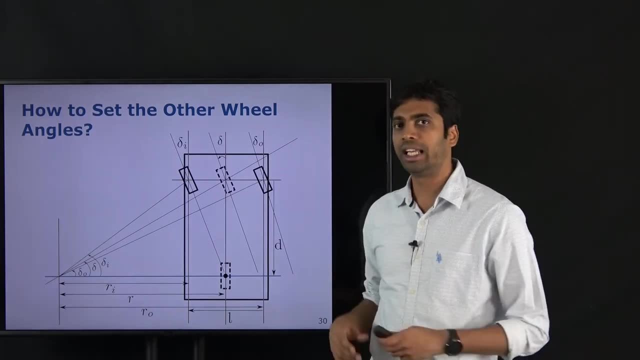 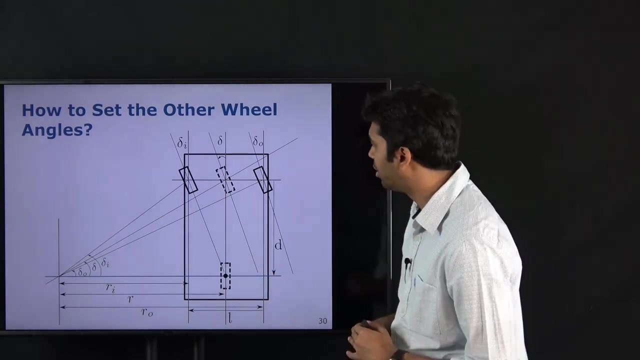 So the question that we want to answer here Is that If this ideal wheel moves by delta degrees, How much should the inner and the outer wheel move by, or how much they should rotate? And again we get the constraints from the geometry of the platform itself. 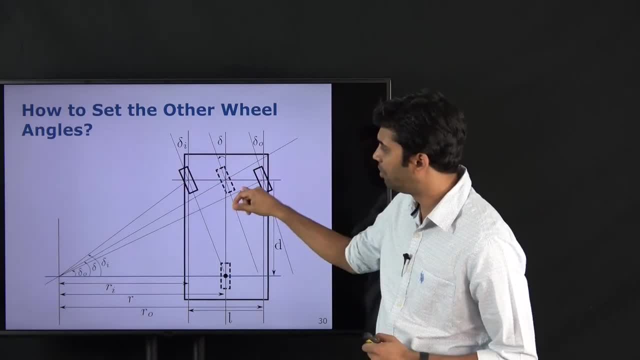 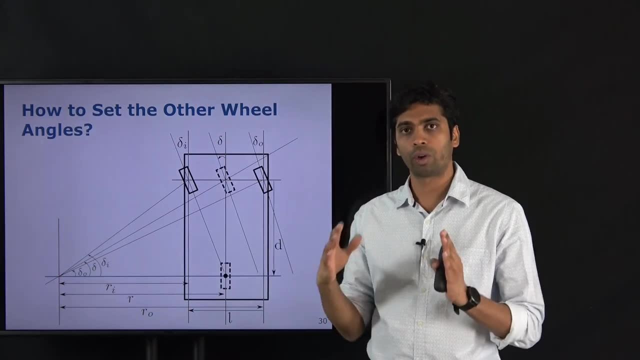 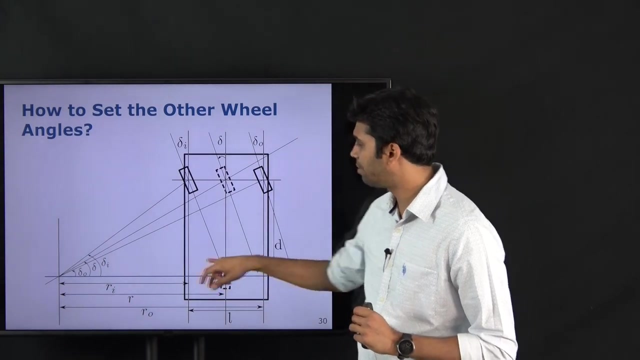 We want that the axis passing through these individual wheels all pass through the same point. This ensures them that the whole overall system would rotate around the same point. This happens automatically For the wheels which are on the back side because they are attached to the same axis. 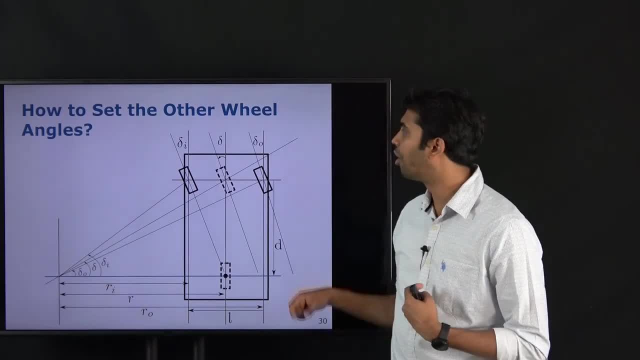 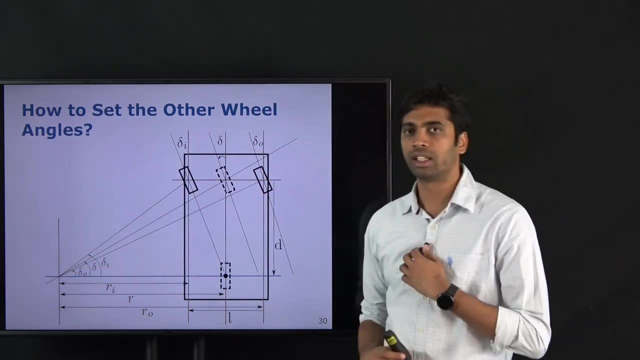 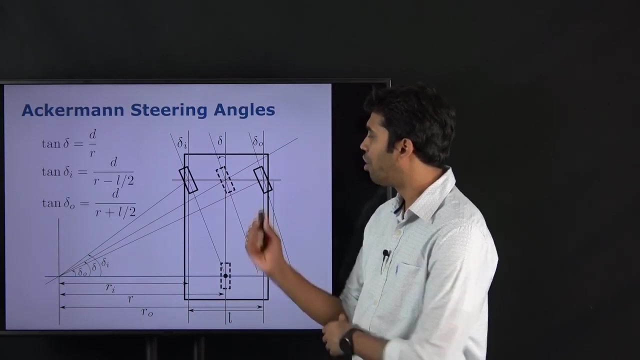 The axis through them will also pass through the instantaneous center of curvature. What's more tricky is how to ensure that the front two wheels also pass through the instantaneous center of curvature And, like before, if we write down the formulation or the relation- geometric relation- here. 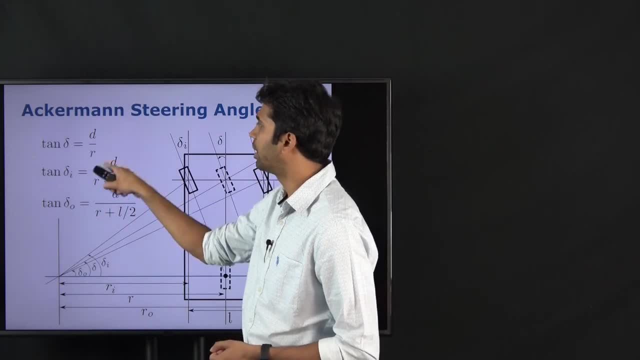 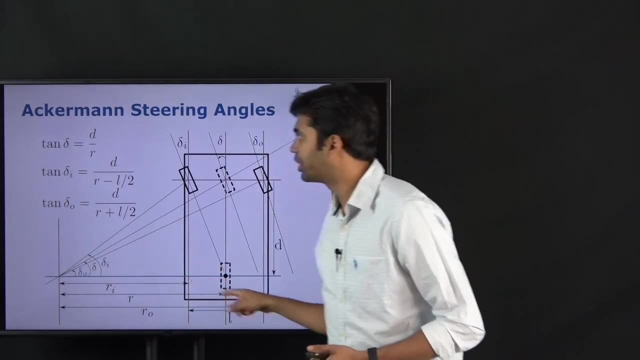 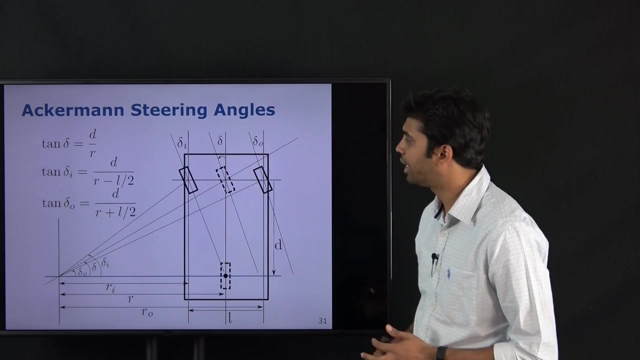 We had this from before, that the tan of delta is nothing but d over r. So this v base length, so to say here over the radius of curvature. Similarly, for the inner wheel, delta i here, or the left wheel that you see here, is nothing but the d, which is the same. 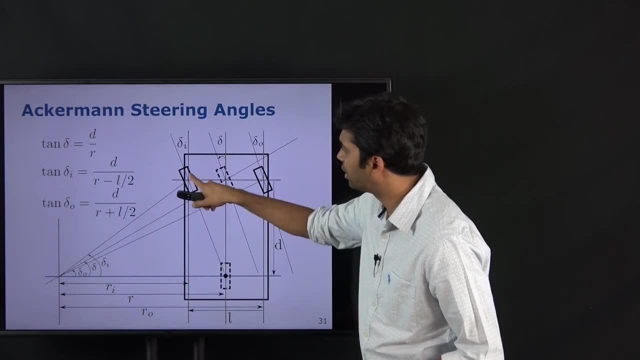 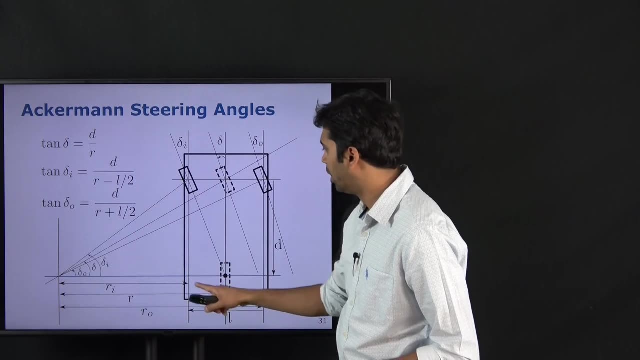 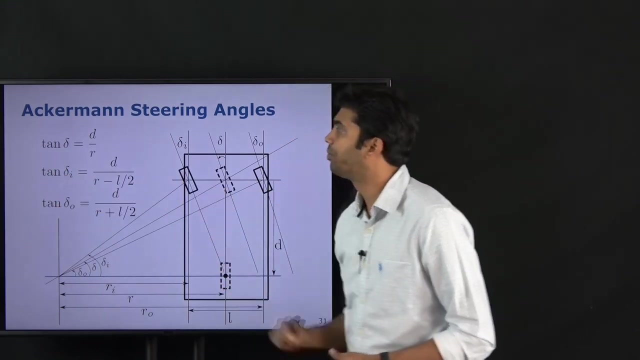 So this length is the same, whereas the radius along which it's turning is shorter. So it's r, which is the distance from the center to the RCC minus the half of the length of this width of the car, And therefore we have the relationship for the inner tire or inner wheel as tan of delta. 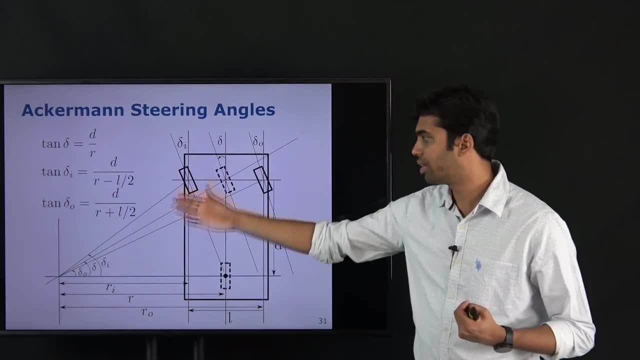 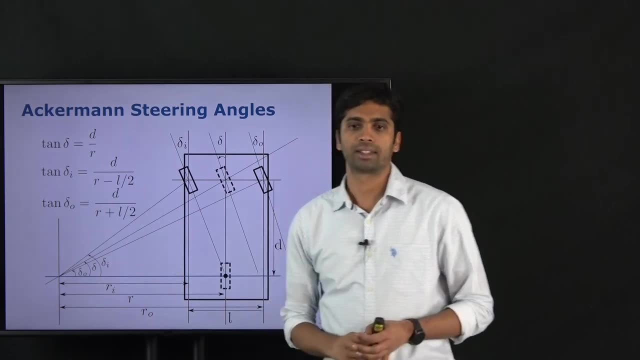 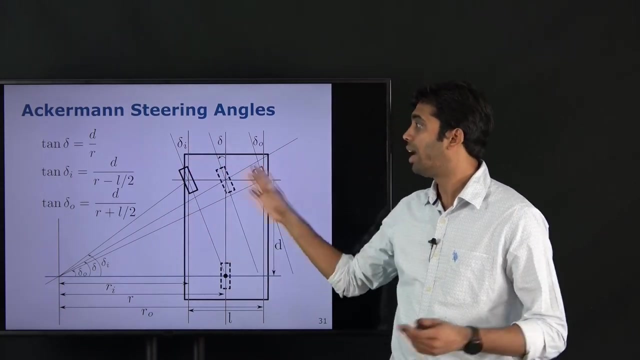 di is d over r minus L by 2.. And similarly we can argue for the outer wheel. this being tan of delta 0 is d over r plus L by 2.. So now, if we set these angles, delta i and delta o, as given by these equations, 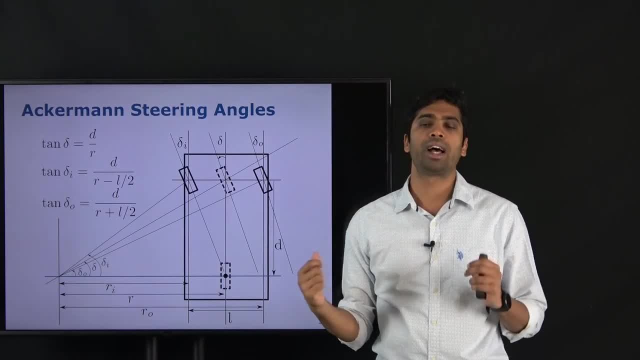 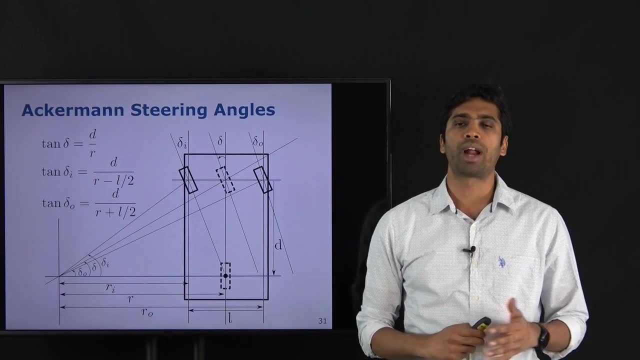 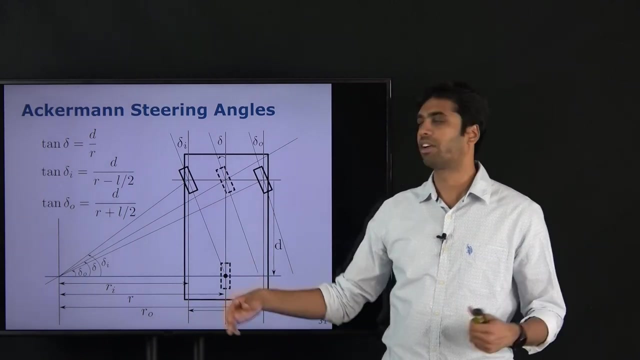 We would ensure That the entire platform has one instantaneous center of curvature and therefore would move smoothly along the curve that we want to track. And so, in principle, if you have a car for which we can make some digital calculations, we could think: okay, we could take the arc tan of these numbers and then figure out based 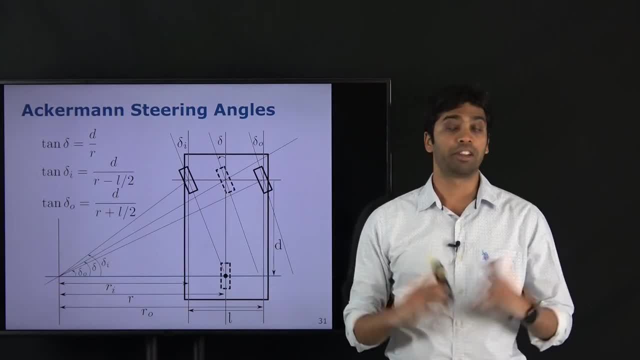 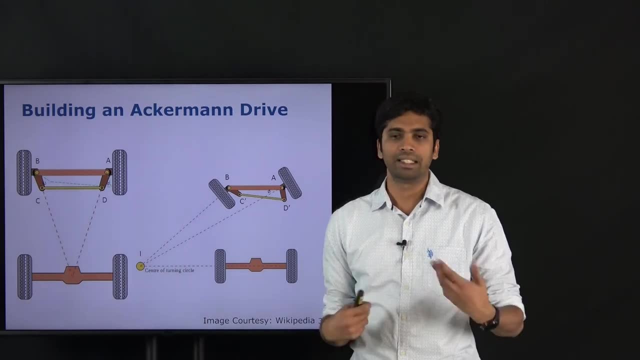 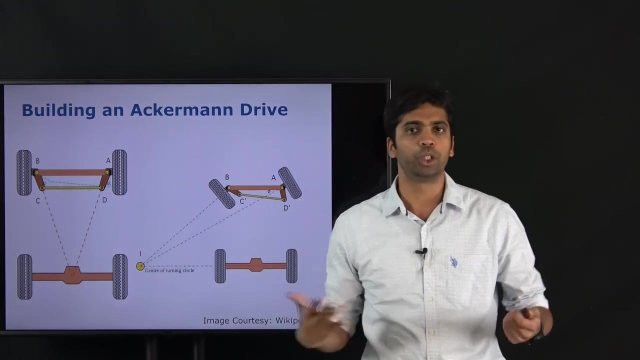 on the curvature that we want to track, how much we should steer if it's an autonomous car. However, this problem is not something that's new And this has been done for quite a long time. for example, here, what we see, the solution was also used, is used in cars, but also was used originally for horse carriages. 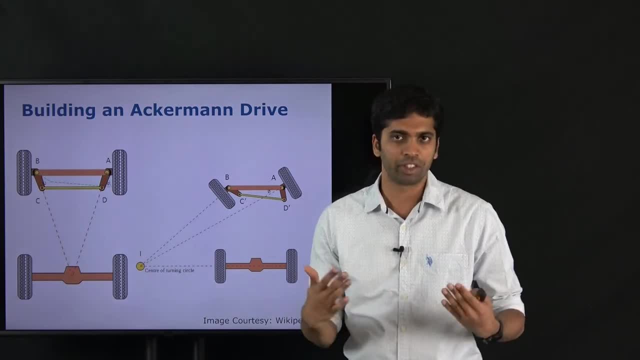 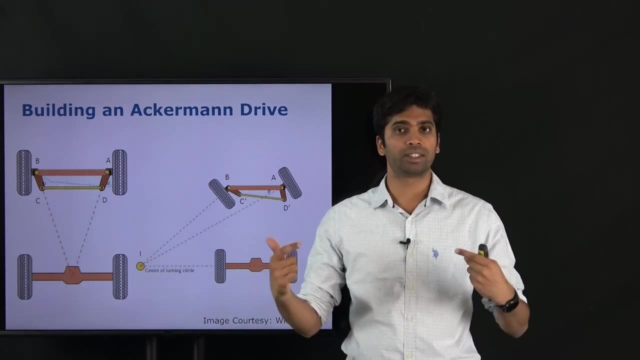 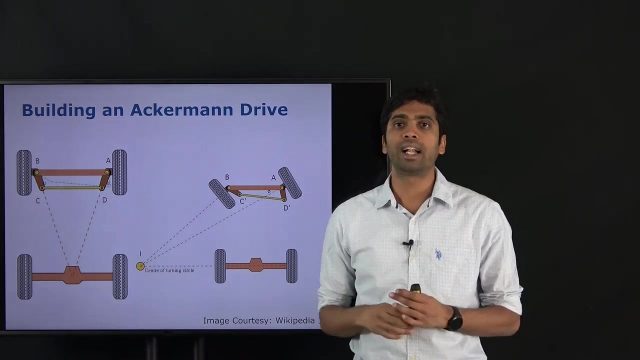 So what was happening was that previously, all the front wheels were steered in the same manner, which we now know is not good because this results in skidding, which results in large forces on these wheels, And this was what was happening, And this resulted in the fact that the carriages- the horse carriages- were breaking down a lot. 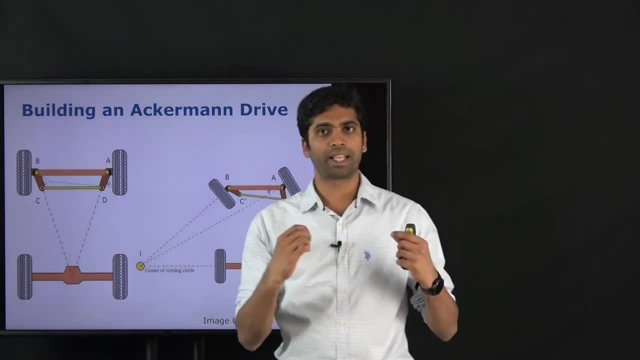 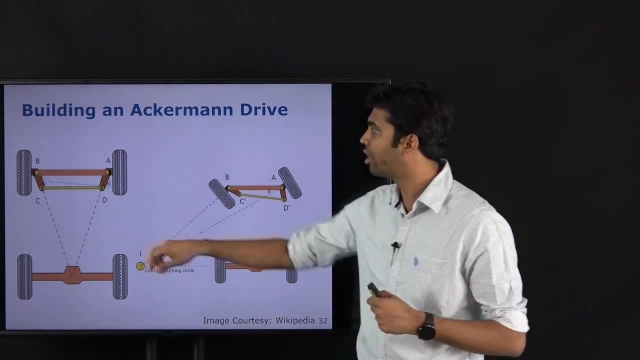 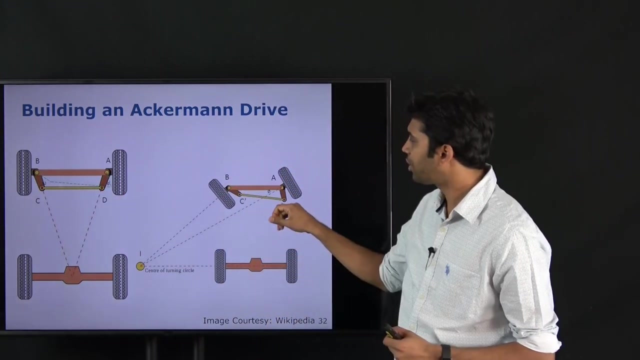 And there was a smart solution which was found in terms of a mechanical fix. So by attaching this extra rod they have to be calculated to be of a certain length. Also, these linkages here have to be of a certain length, Such that now when you pull or when you steer, you can move this mechanism here, such that 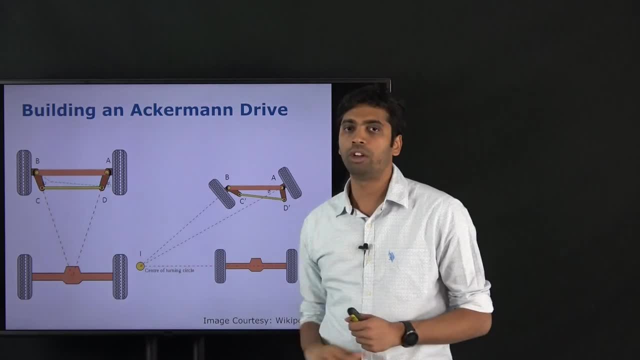 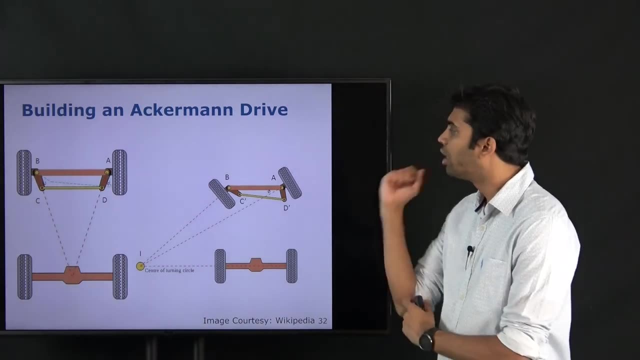 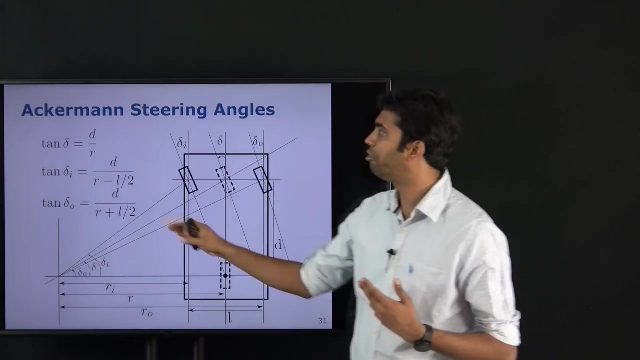 the axis Which passes through the two front wheels will always rotate. This is also roughly how the mechanism in our cars, or at least the older cars, work like. So this is a constraint that is made mechanically similar to, so to say, to enforce these specific 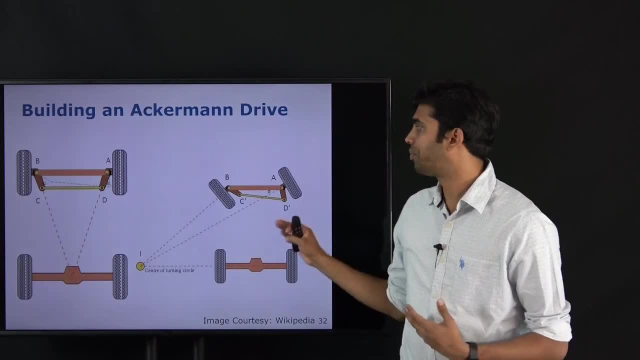 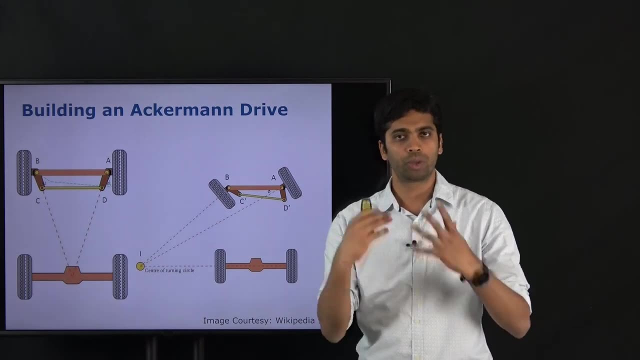 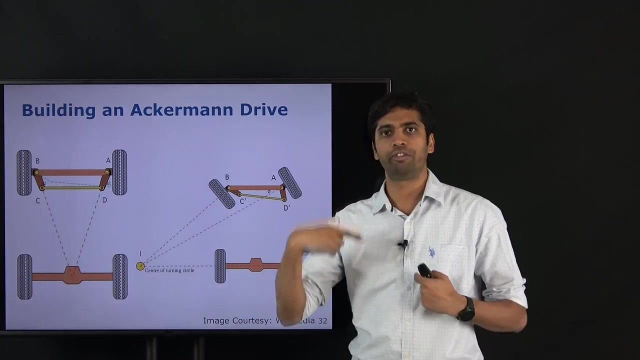 steering angles, but to do it rather in an elegant and a mechanical manner. And so now we know how essentially to control All, Or to drive a common type of car, by ensuring that the all the wheels, all the four wheels, so to say, of the platform are rolling smoothly. 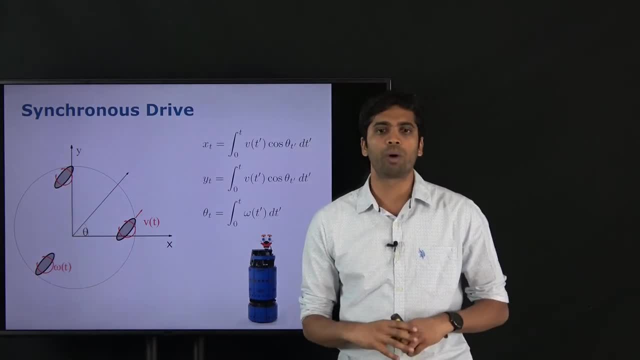 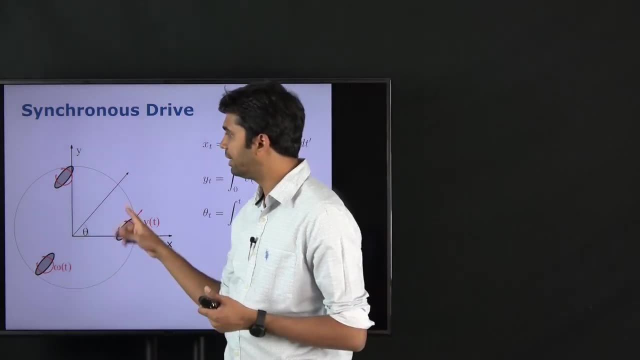 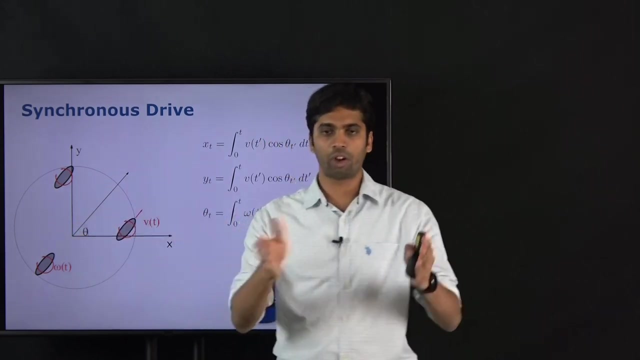 With this we move on to the next drive, which is an interesting drive, also called as synchronous drive. So essentially what happens is that we, in the synchronous drive, you put wheels parallel to each other on the platform And then they all move at the same linear velocity. 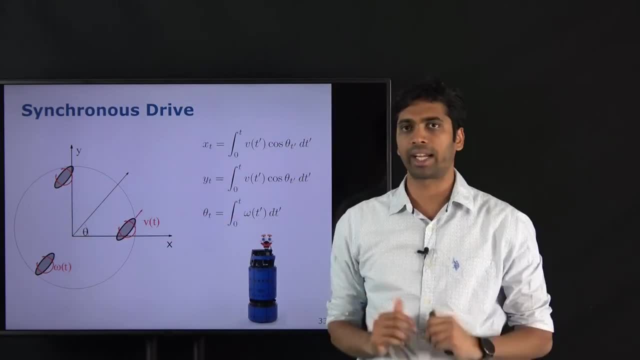 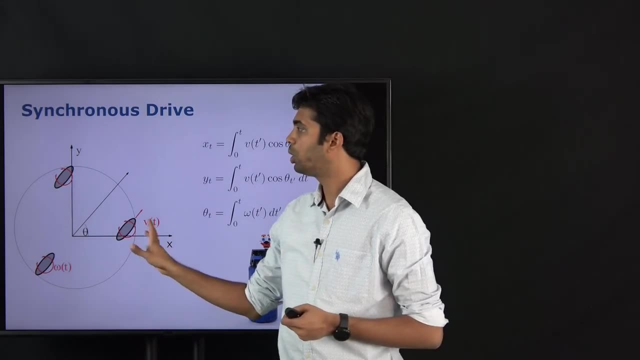 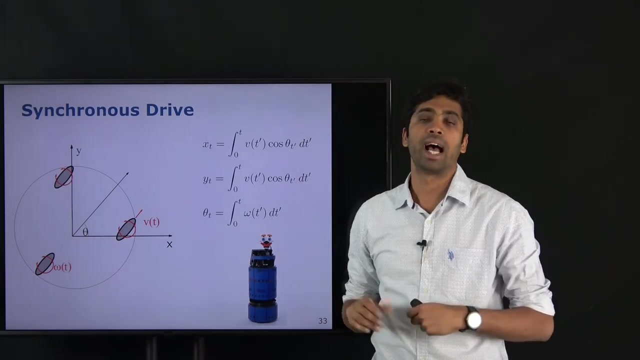 So if you give the same velocity to all those wheels, they would move straight, and similarly, by giving negative of that velocity, they move backwards. And what's interesting is that it's also possible to rotate all these wheels exactly the same. There's one, let's say one motor which rotates certain, at some angular velocity, and that 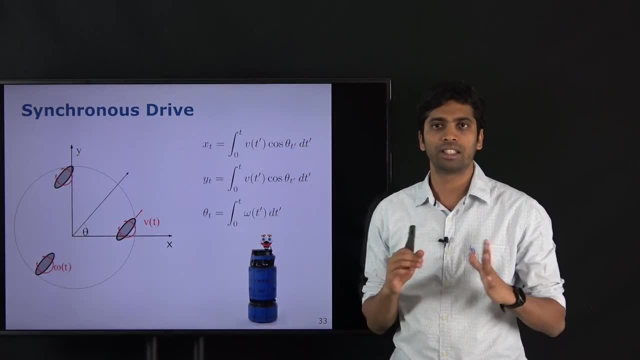 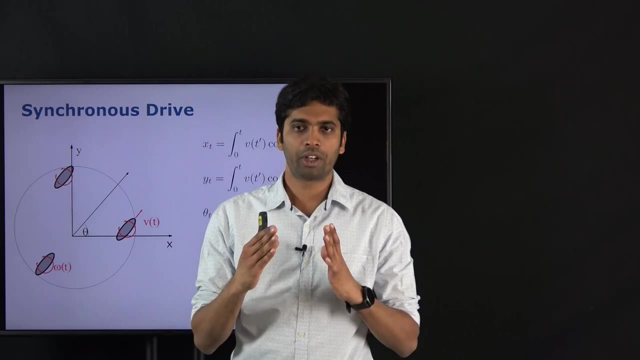 is transferred to each of these wheels. What this then results in is in a very kind of nice motion, where you can move straight and back, But also at a particular angle, Because all these wheels are attached at all. these wheels are rotated in the same way. 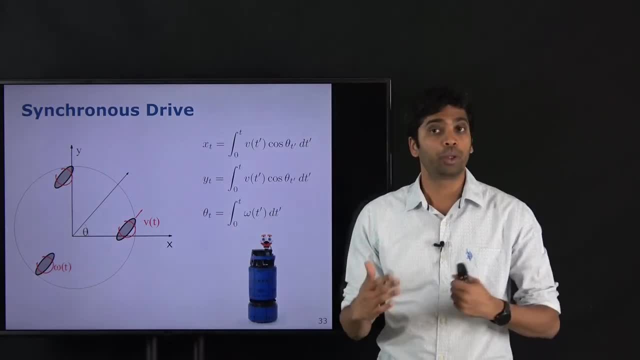 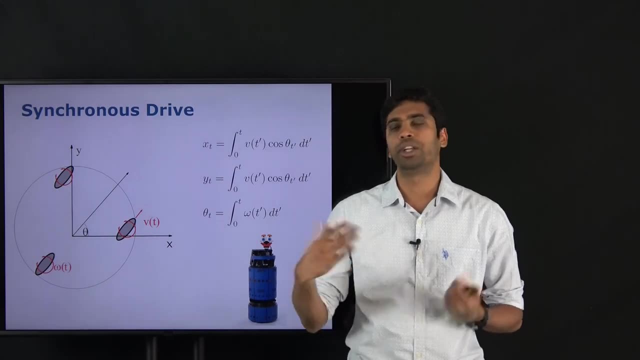 So you could come out with really smooth motions and you could reach portion, you could reach parts of the environment in a confined space, as opposed to using, for example, an Ackermann model, where you would need to do more maneuvering in order to reach to the same positions in. 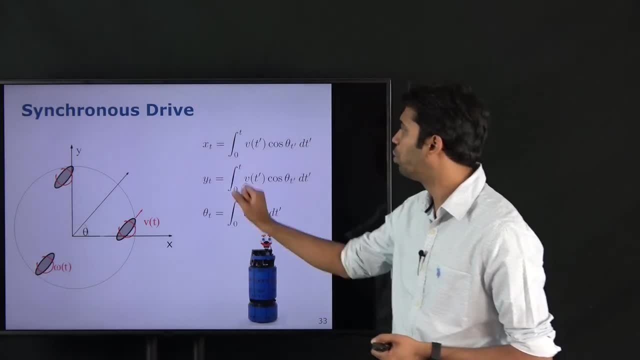 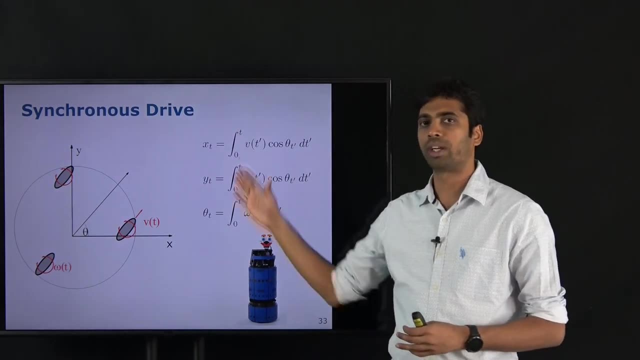 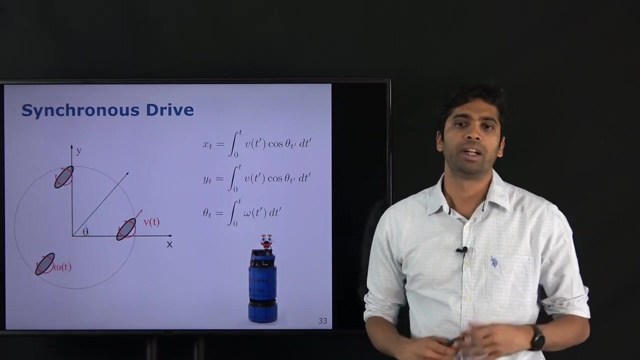 the in the environment, And again similar to what we saw before. in order to understand what our new positions would be, we need to integrate our velocities over time and this will give us the. this will help us infer where the robot is at time t plus one. 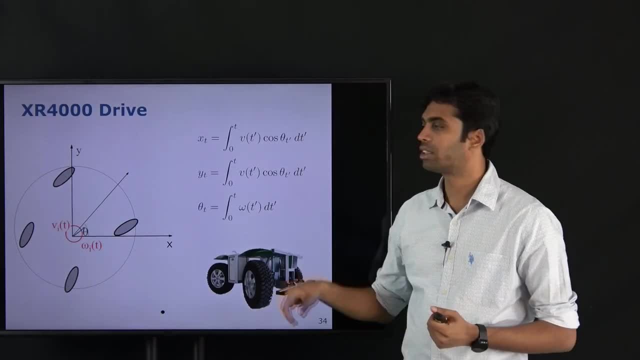 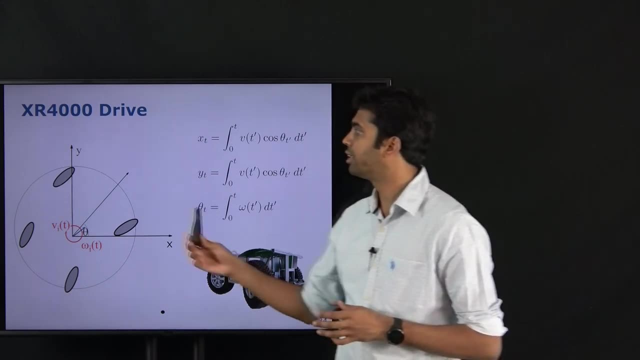 Another interesting robot is, or drive is, this XR4000, what was initially done in XR4000.. It's almost like an Ackermann drive in the sense that there are two wheels on the front which can be steered, But also the wheels on the back 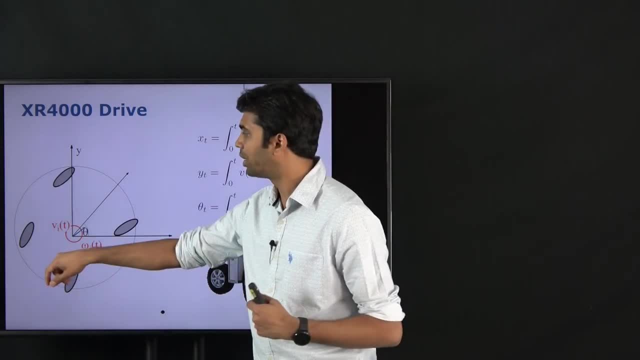 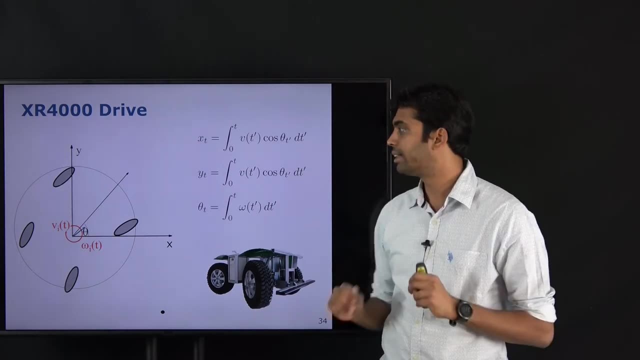 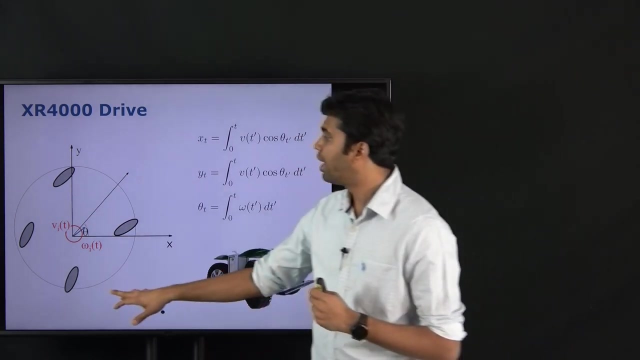 Can be steered. So, in this sense, what one does is to have the axis of these front and back wheels intersect at a particular ICC. Then we can ensure that the that the whole system rotates around the ICC by moving both the front and the back wheels. 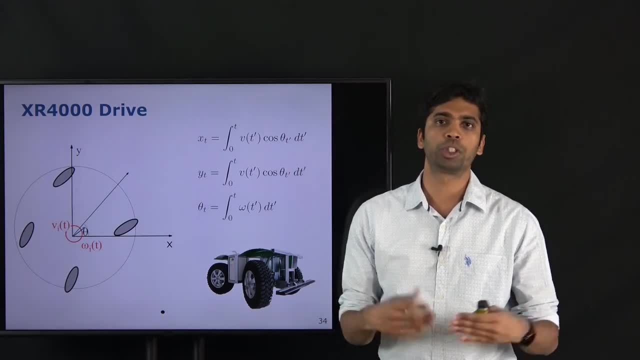 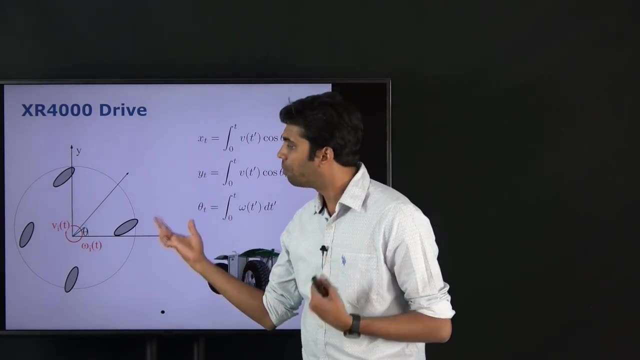 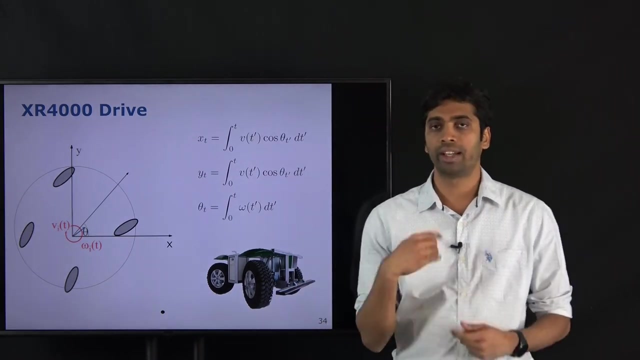 This allows to move in tighter circles than is what is possible with Ackermann drive. So this is really interesting. This is an interesting kind of drive which is mainly used in the outdoor environments, and this is an example of such a robot. Again, the for the inference of the next time instance. so whether the pose of the robot 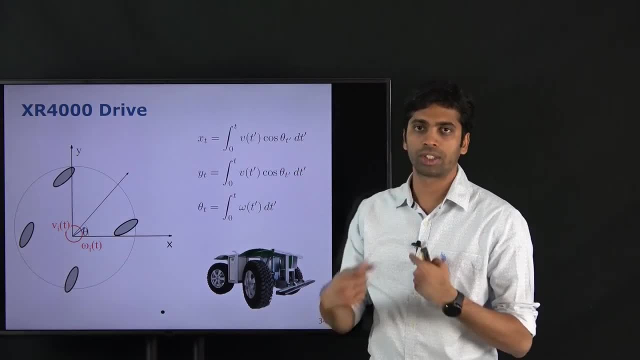 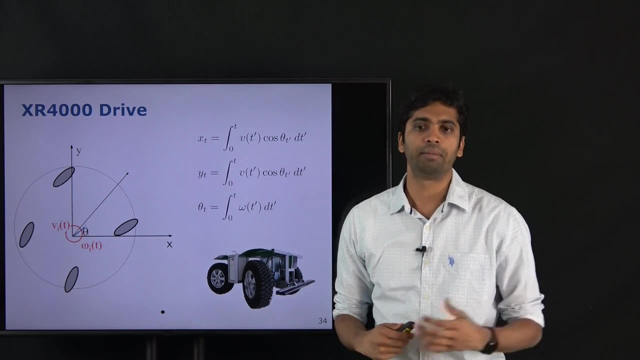 at the next time instance we do the same. So we have to integrate the velocities over delta t's, which would give us the idea of where this robot would end up in at time. t plus one, Right. So, like I said, So we want to ensure that. 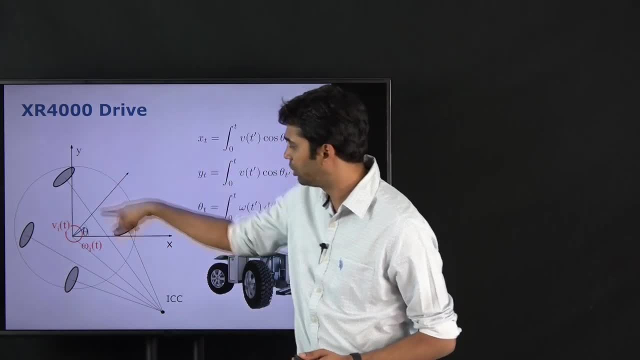 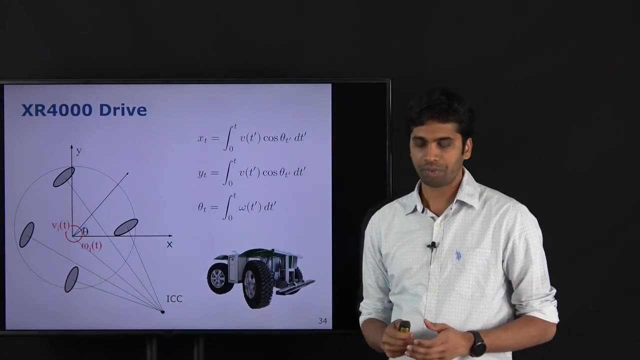 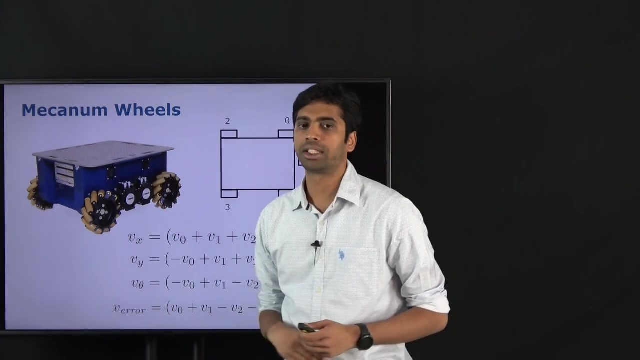 That, the, That the ICC. so the axis passing through these four wheels end up through or pass through this ICC, which would ensure a smooth motion. So this last mechanism that we see here is really one of the coolest ones. So this is obtained using what are called as mecanum wheels. 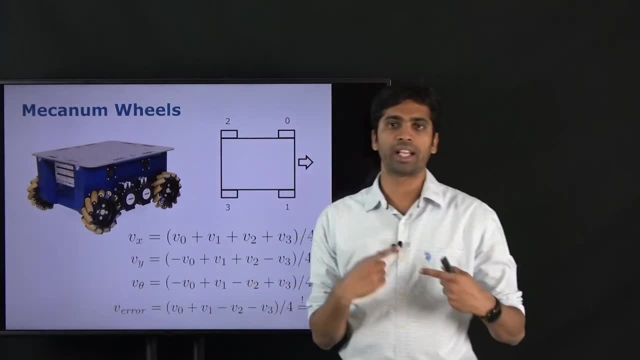 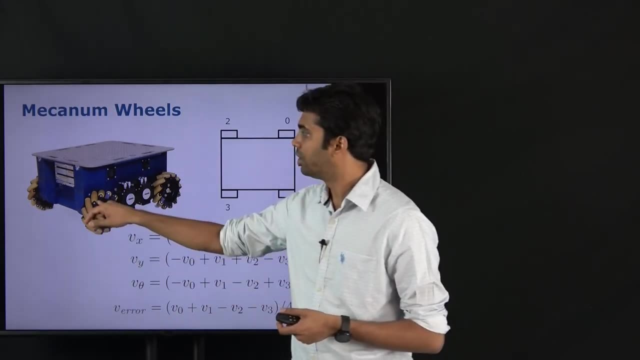 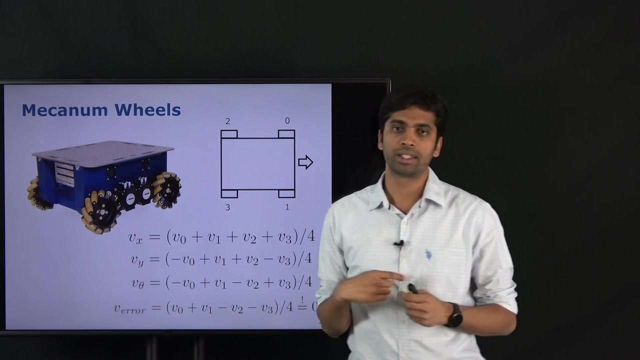 So essentially these are four motorized wheels with some passive rollers on top of it. So there are wheels on top of wheels. So these, These rollers are normally put at an angle of forty five degrees on top of these actuated robots, actuated wheels, and by rotating these actuated wheels, these rollers, then passively 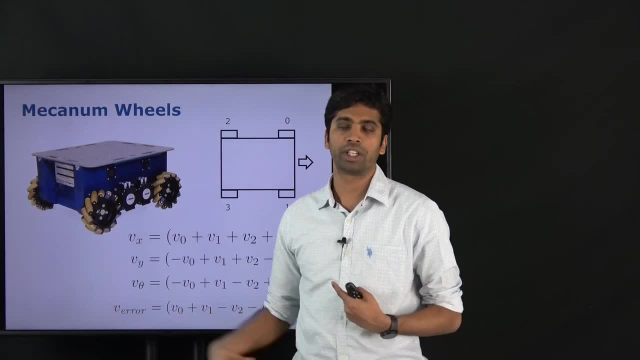 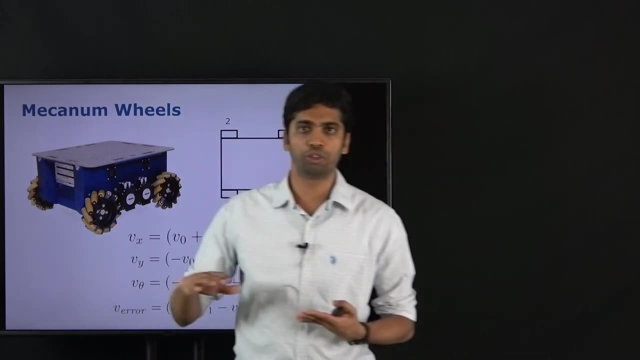 so to say, rotate due to the normal forces in the friction from the ground, And what this allows is to do is to is to make movements, for example, a sideward movement, which would be not possible with a Ackermann drive, or even with a differential drive. 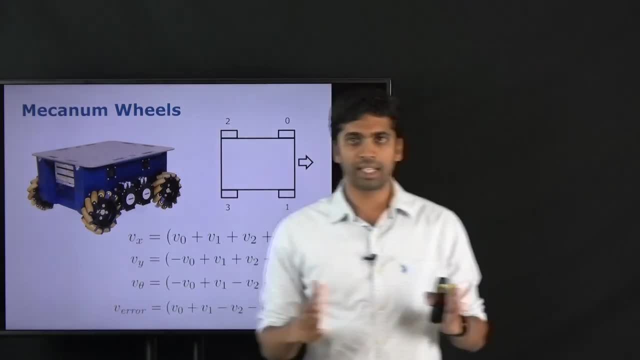 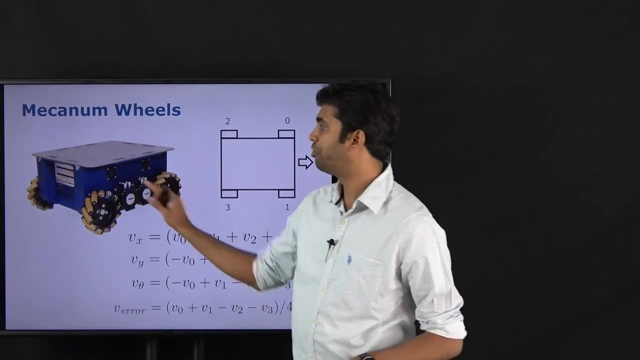 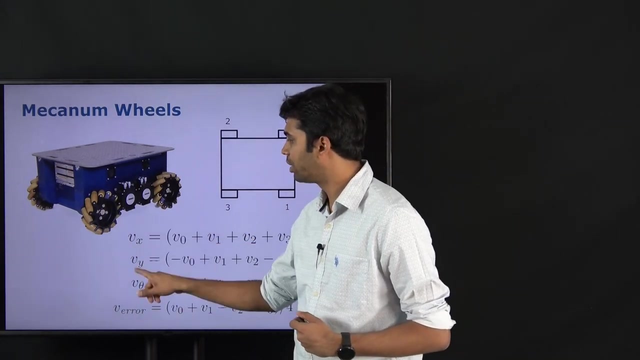 So with these kind of robots, Right, They can move, for example, side and so on. So, for example, if you look at the equations here, we have basically four motors, so there are four degrees of freedom and we can set the individual velocities on the X, on the. 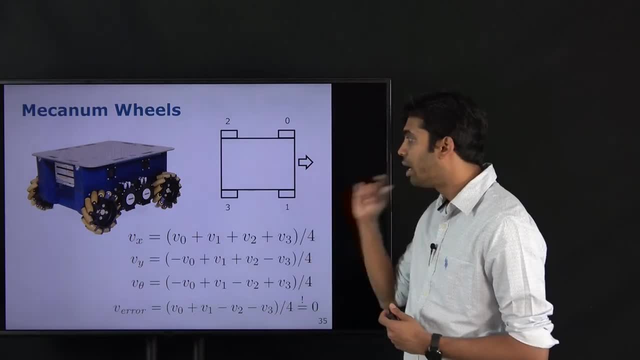 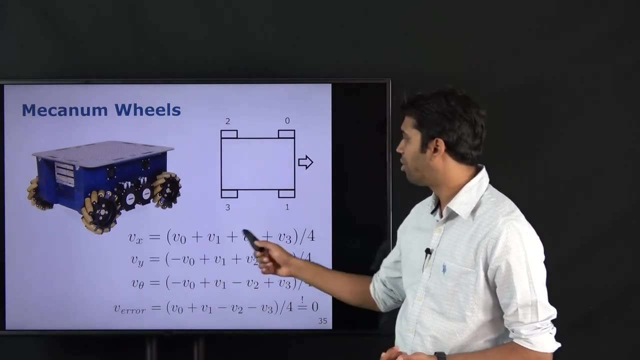 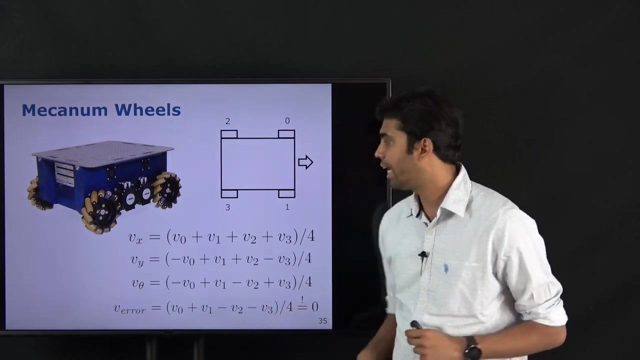 Y and on the, the rotational velocity, by setting these different velocities on the four wheels, So by setting certain velocities for V0, V1, V2, V3.. So the V0, 1, 2 and 3.. Right, We can obtain a particular velocity in the X direction, similarly in the Y direction, and 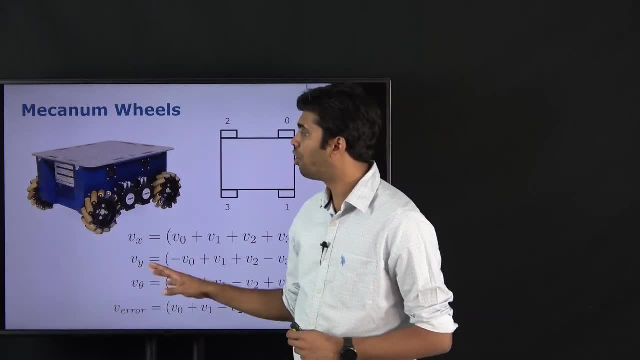 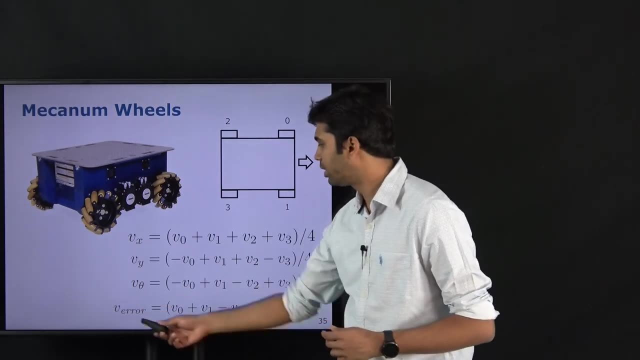 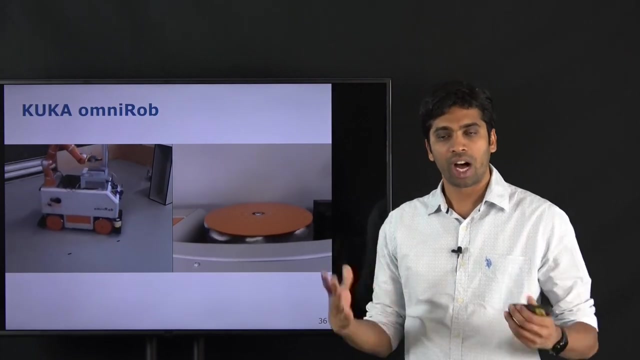 an angular velocity. Since we have four motors and only three degrees of freedom, we also have to ensure that this error vector, or this error velocity, goes to zero. So let's look at how this motion or how this mechanism looks in practice. So this is a robot, for example, which has this mechanism: wheels. 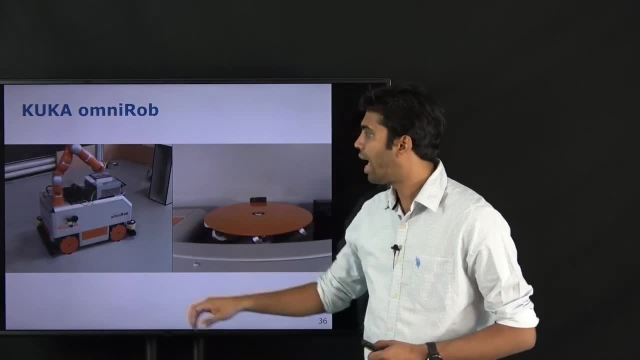 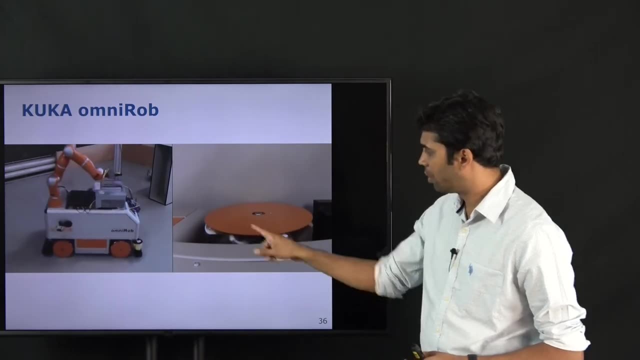 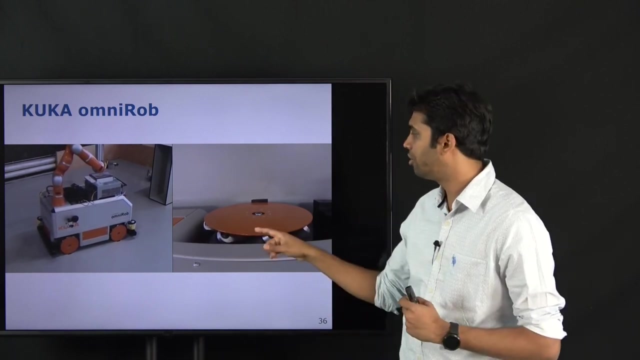 And, as you could see, it slides along the floor and reaches. this particular is done for some other application, But as you see here, the- the active wheel rotates, but also the passive wheels on on its collision or on interaction with the surface also rotates, allowing it to move on sidewards, for example. 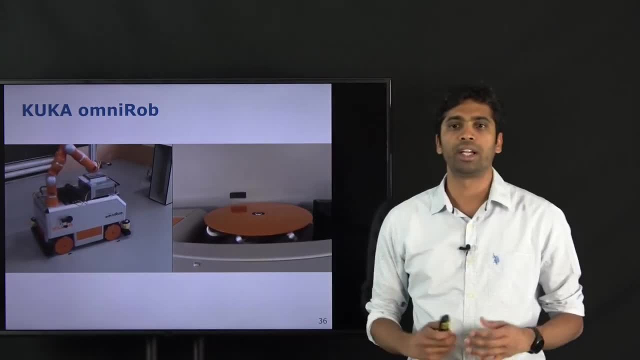 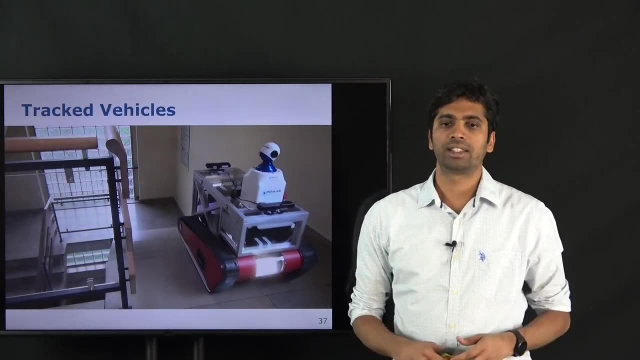 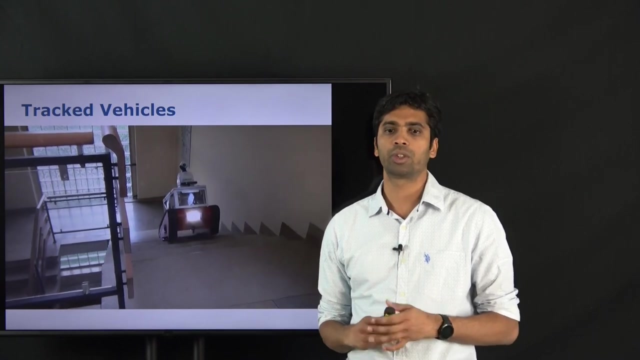 and creating motions, which would not be possible with other kind of drives, Right? So the next kind of vehicles that we see are what are called as tracked vehicles. In this case, these are almost similar to the skid steer vehicle that we saw, but there's 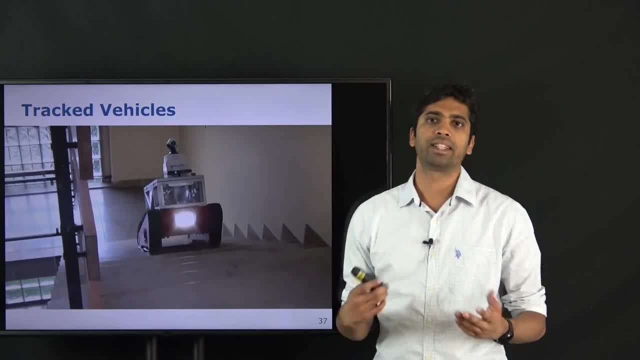 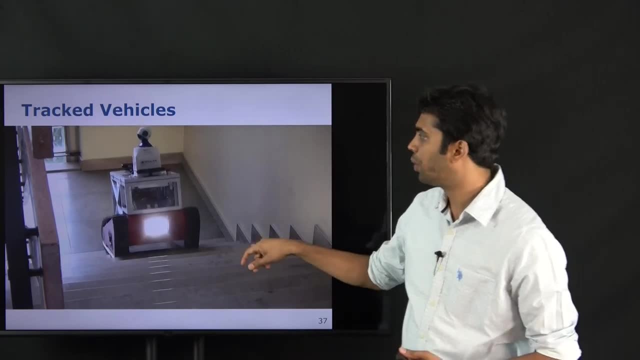 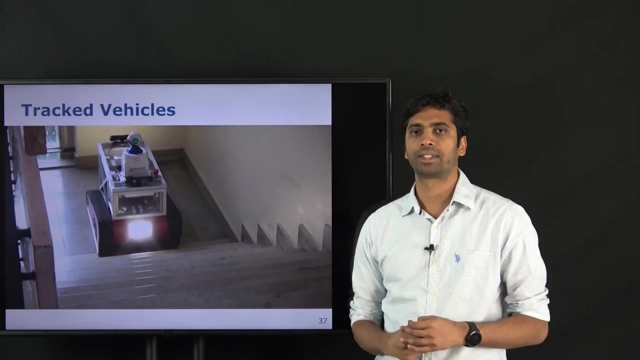 a track around the platform, and these are really interesting for for environments which in which wheels won't do So. you really need to have these kind of tracks in order, for example, to go up and down rugged surfaces or stairs in this. As you can imagine, this is quite a rough kind of drive. 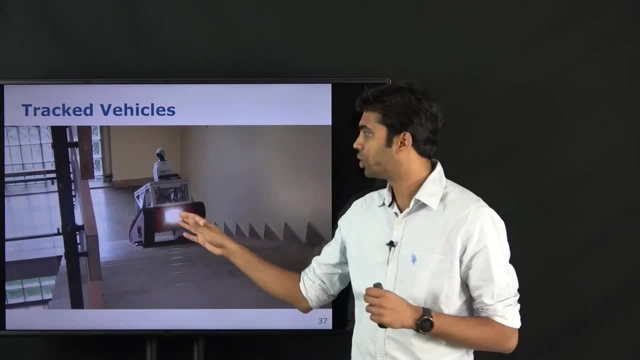 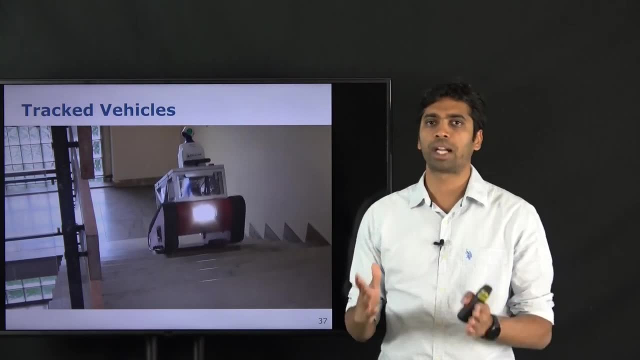 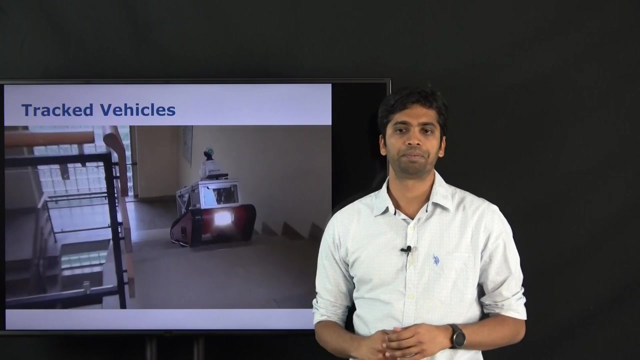 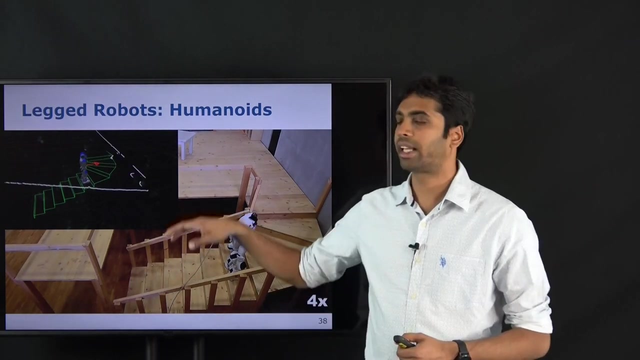 So there is no mechanism per se to to steer these tracks so that you can have a smooth motion Whenever you turn. they're not the nicest experience, but basically essentially use skid in order to turn, similar to the skid steer mechanism. So what we see here is another kind of robots or a kind of motion, in this case a humanoid. 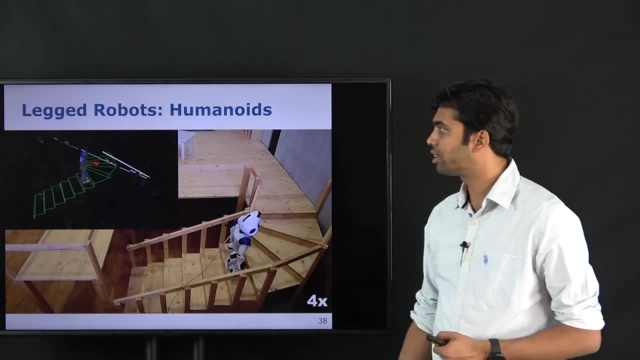 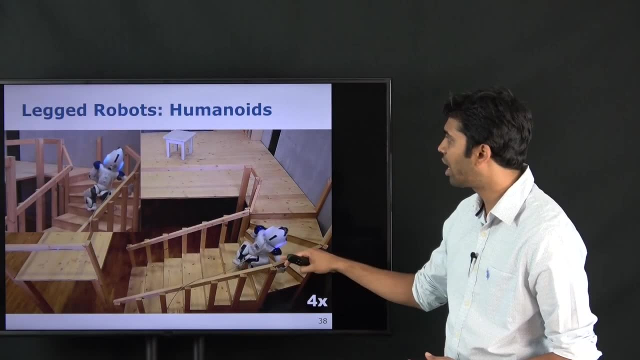 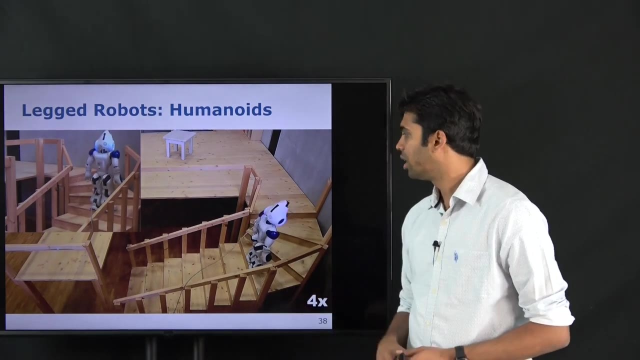 motion. So we have legged systems. So the movement or the locomotion for a humanoid system is much more complicated, as it first has to figure out, in this case, where those steps are and then make the movement. So in this case the robot does what is called as a static, statically stable movement. 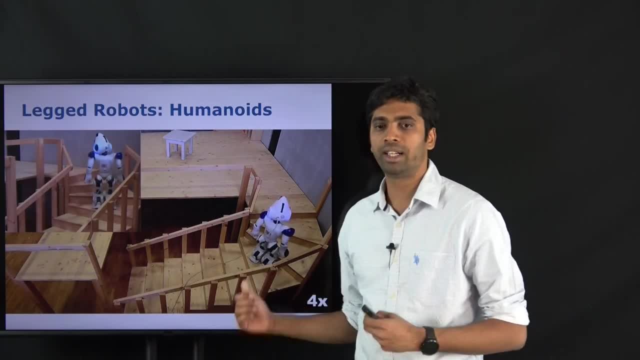 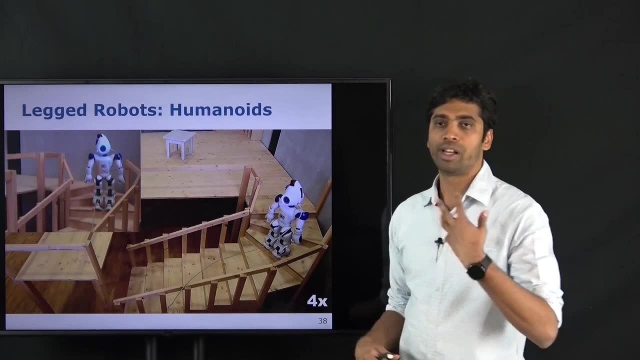 So it moves such that at every point in its movement it's stable. So we as humans Typically don't walk like this. We walk in a dynamic way such that we may always be falling, so we're not stable at each point of time. 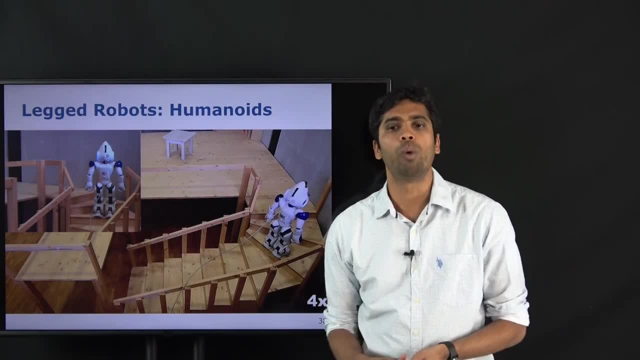 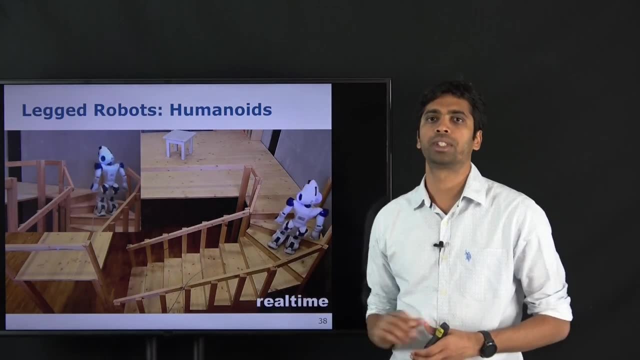 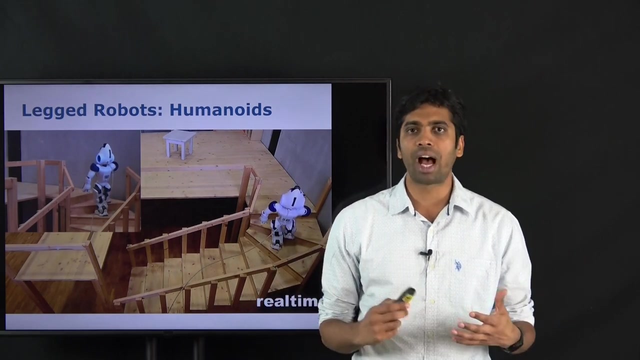 But while tracking or while movement, we are stable overall. So this is another kind of movement which is not a wheel based movements, but using legged systems. So the main advantage of such systems is that if we want a robot to operate in environments which are already, so to say, made for humans, 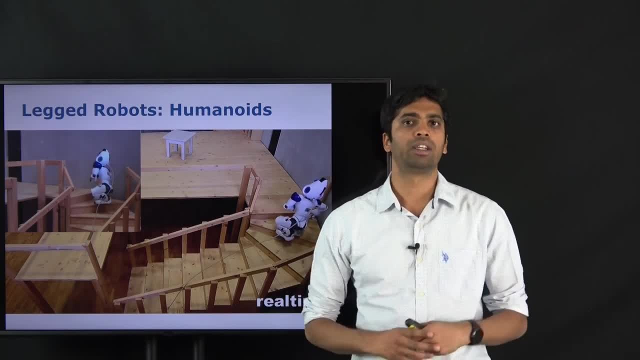 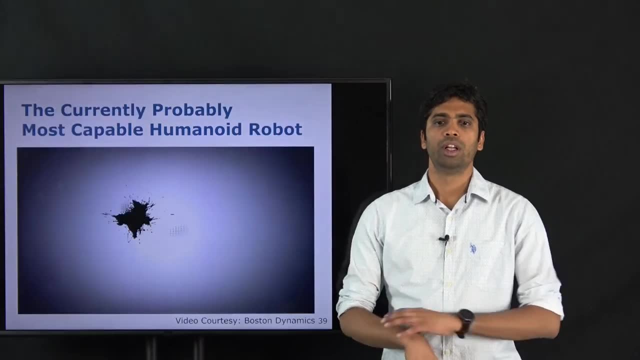 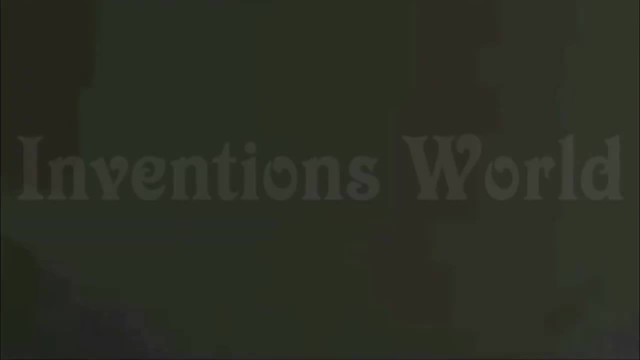 You don't want to redesign them for wheeled vehicles. This is the kind of systems that one needs to develop. So something that's more cool, so to say, to look at is this robot, called as the Atlas system, that's developed by Boston Dynamics. 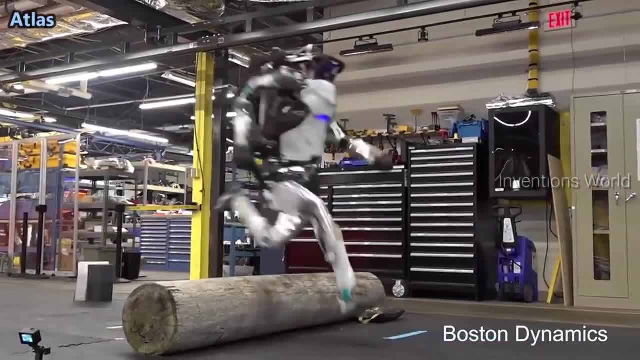 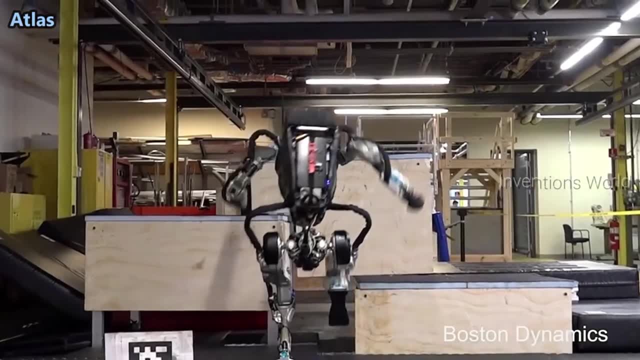 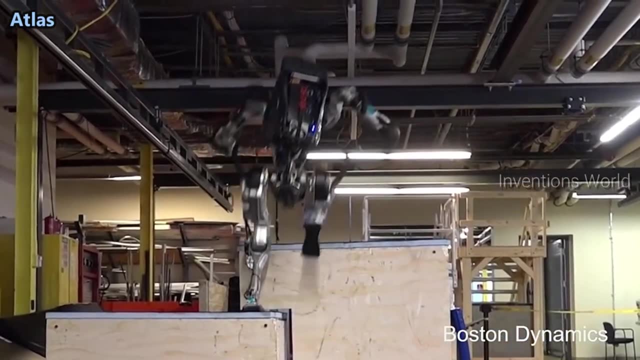 So in this case, what you see here is a dynamic kind of stability, So it's not stable at any one point in time, but overall, while making the movements, it's stable. So this is a very complex system with several controllers ensuring that these different motions are being followed. 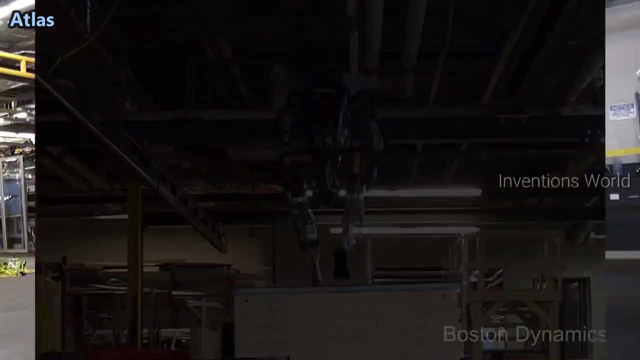 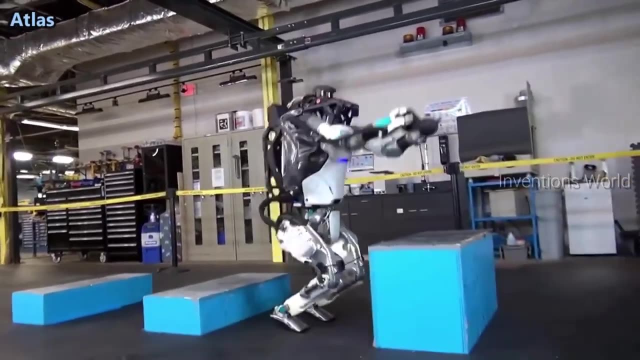 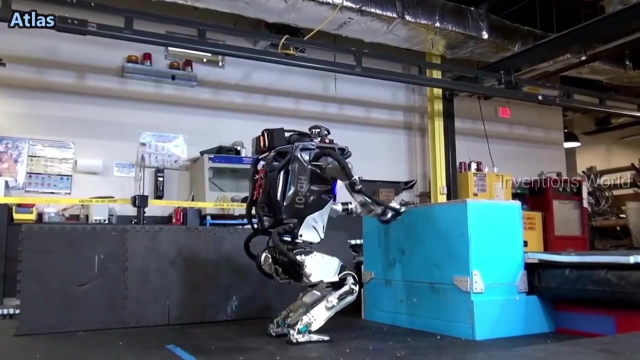 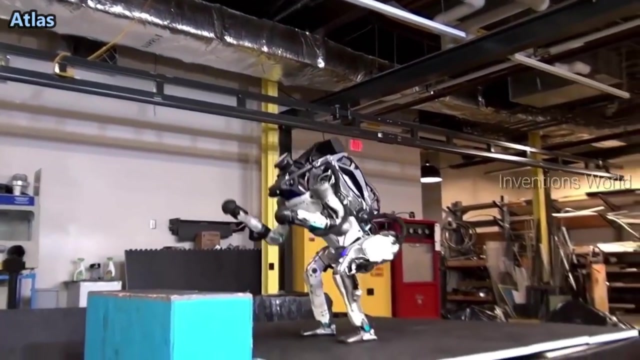 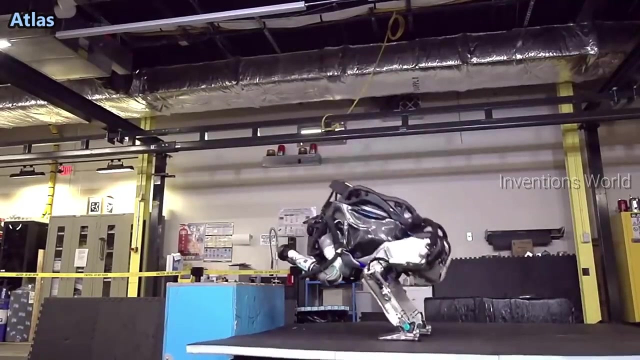 It's one of the very few robots which have these capabilities to do it, So they're able to do These really complex movements. This is, of course, helped by the specific hardware that they have, But also understanding the dynamics or understanding the movement in order to do such complicated. 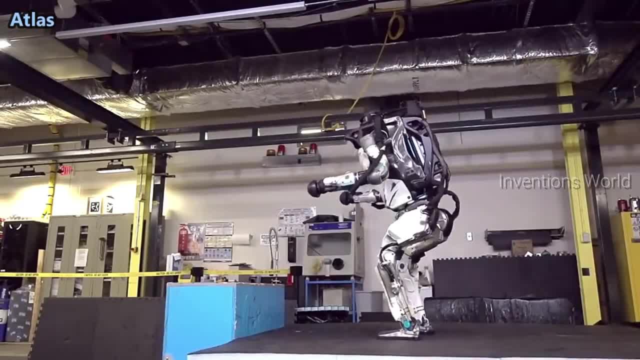 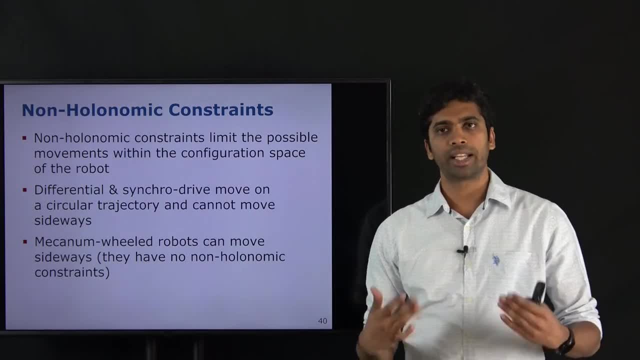 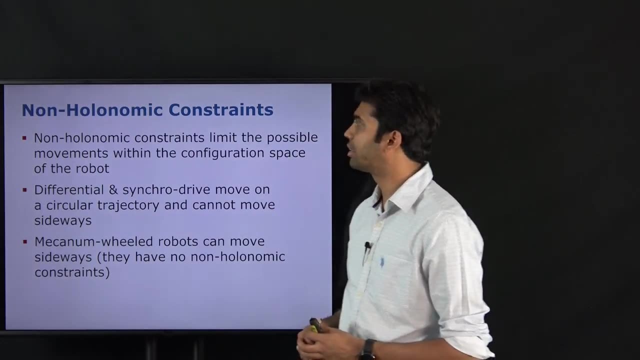 tasks in the environment, so to say. With that, we move to a couple of terms that we often come across when we are studying or reading papers about motion of different platforms, And one of these terms is the motion of motion. Okay, And one of these terms is what is called as the non-holonomic constraints. 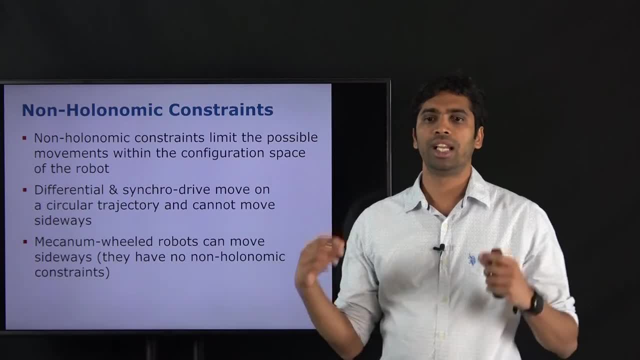 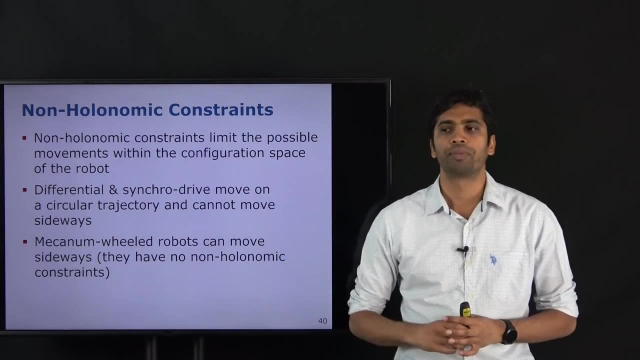 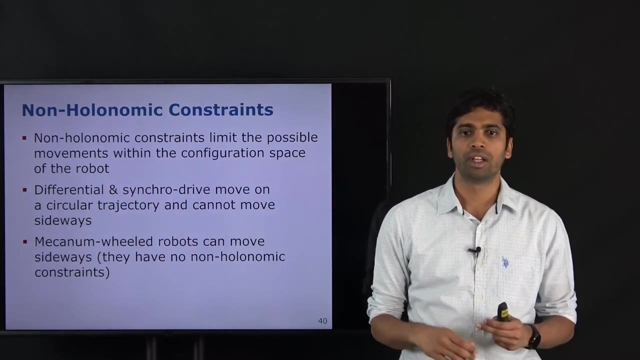 So essentially non-holonomic constraints are those which limit the possibilities for a particular platform: how it moves in the configuration space, or how it moves or to where it can move. For example, if you think of a differential or a synchronous drive, they can move on a. 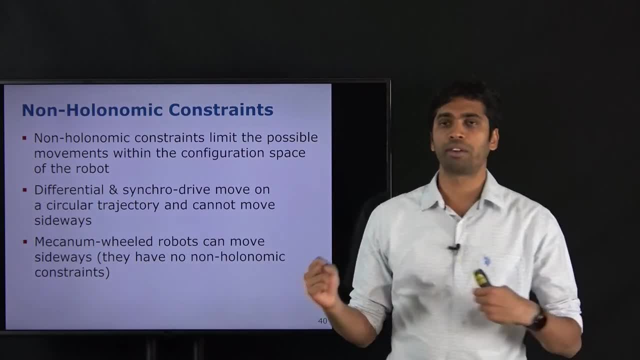 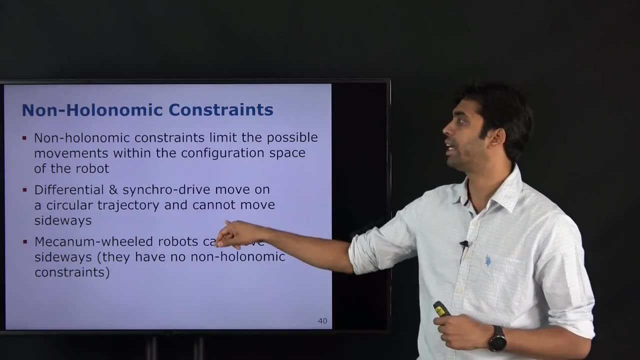 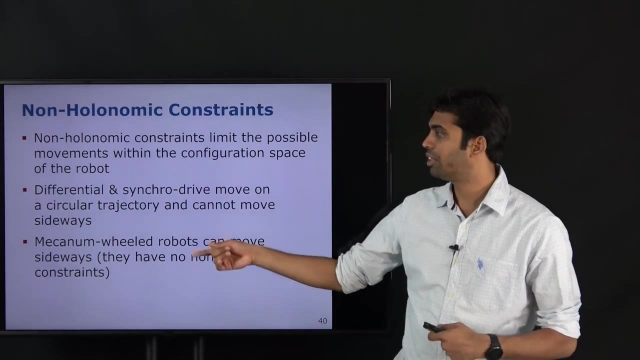 circular trajectory. so they can move on any circular trajectory, including one with a radius of zero, but they cannot move sideways. So this is a kind of a holonomic constraint that exists for our differential robot. However, if you think of the same case when we have a robot which is equipped with mecanum, 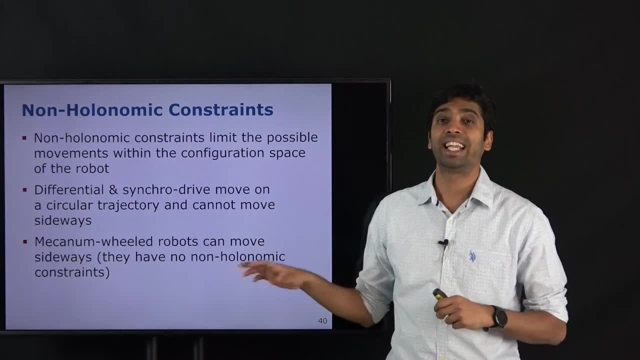 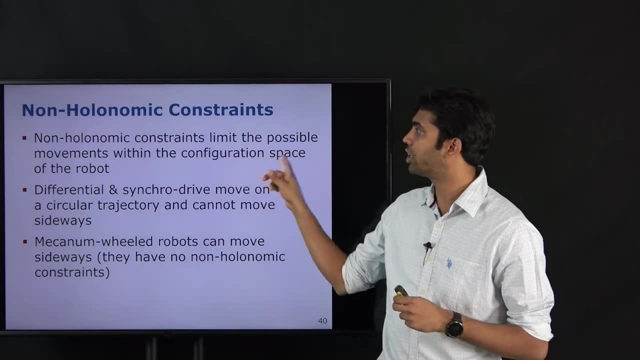 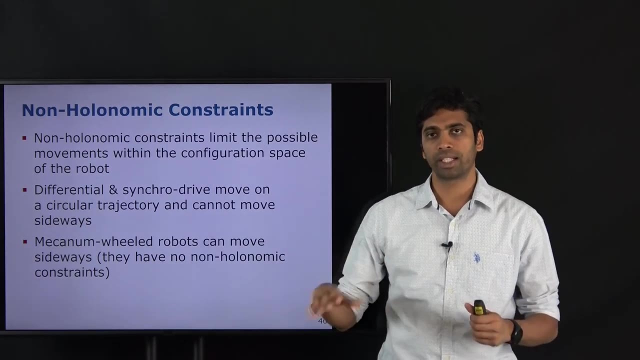 wheels, so the wheels, which lets us move sideways as well. it has no holonomic constraints. So there is no place or there is no post, so to say, in the configuration space where we cannot reach. Okay, We cannot always reach any particular post in the configuration space, starting from wherever. 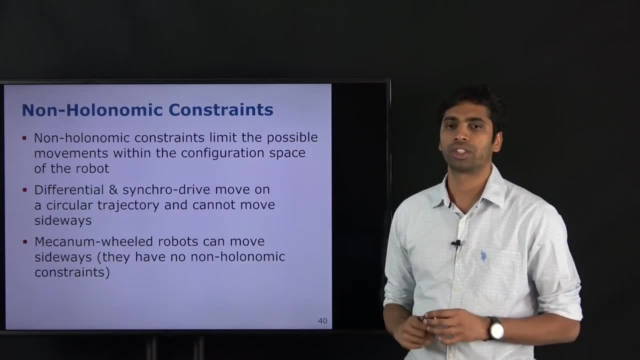 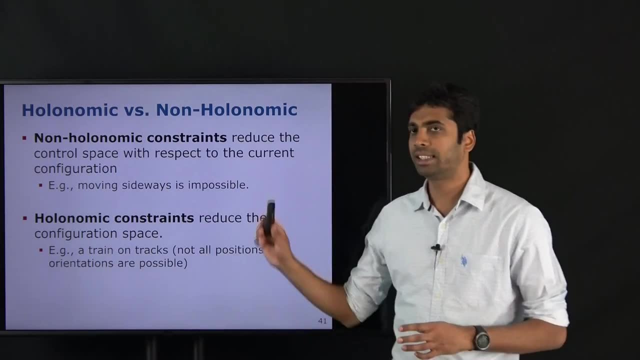 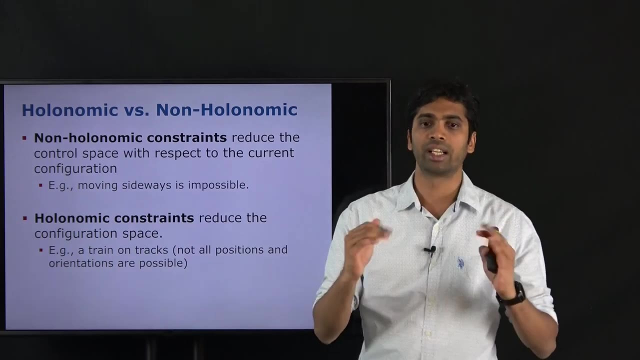 we are if we have no non-holonomic constraints. The other term that exists there is what are called as holonomic constraints. These differ from the non-holonomic constraints in the sense that holonomic constraints are those constraints which actually restrict the configuration space or the valid configuration. 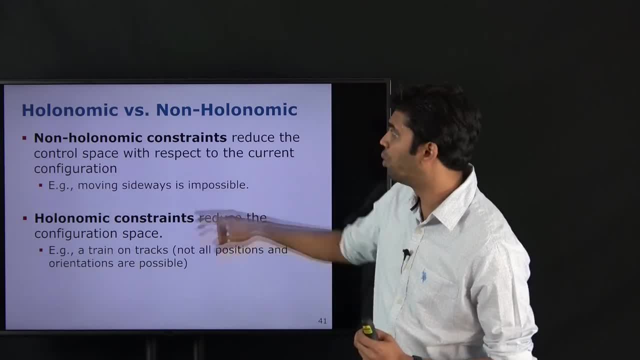 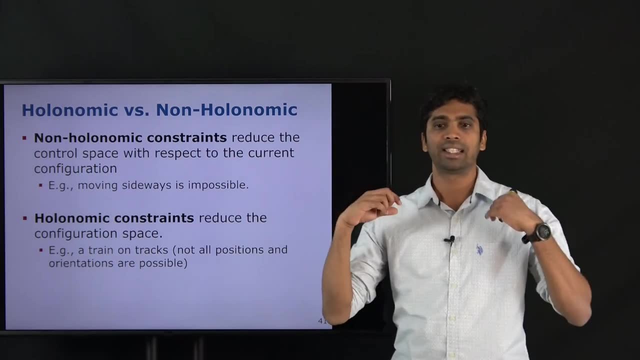 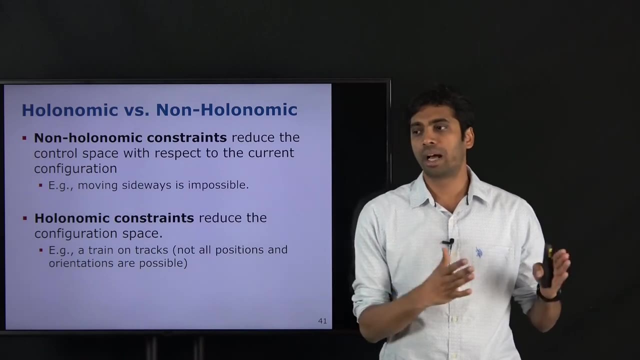 space that the platform can assume in the first case. So they sound similar. Okay, They sound similar, but it's slightly different, the two constraints. So in the non-holonomic constraints, it's that the control space with respect to the current configuration itself is reduced in the sense that, for example, for a differential robot, 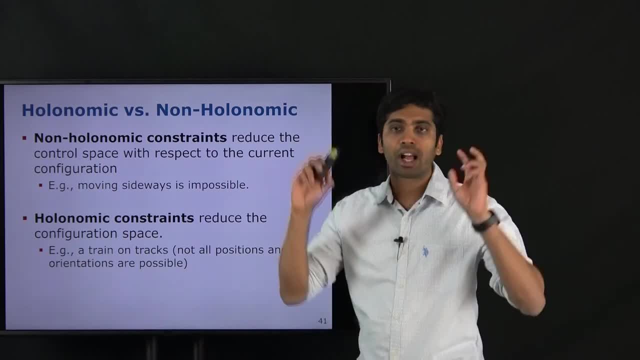 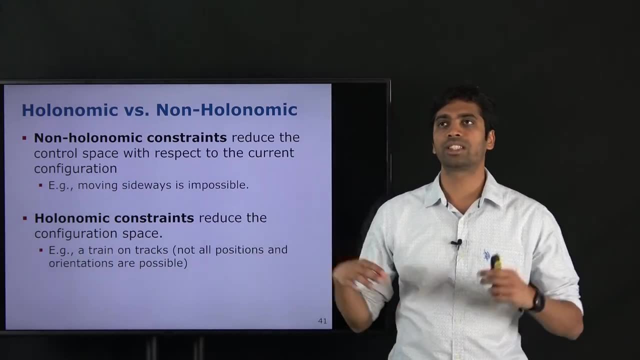 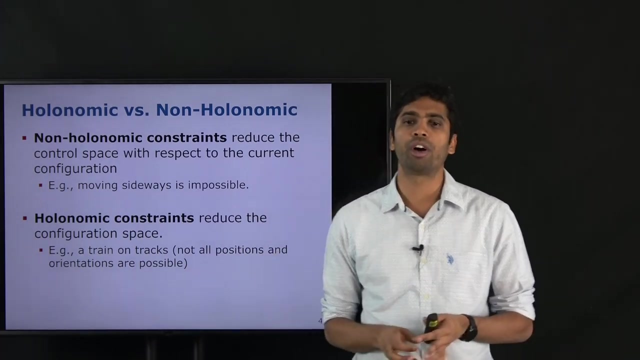 moving sideways is not possible due to the lack of, so to say, the controls on that particular platform. But whereas holonomic constraints mean those constraints or those parts of the configuration space that are not reduced, That are not reachable at all, irrespective of our controls itself, 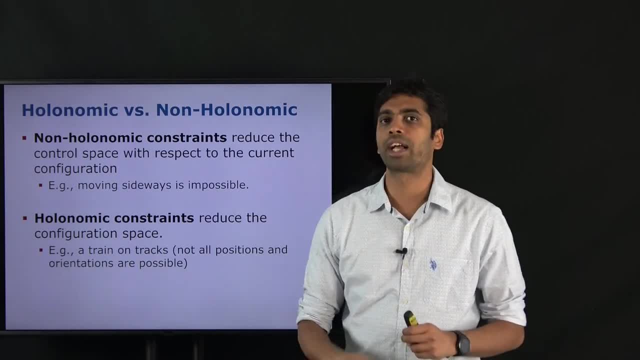 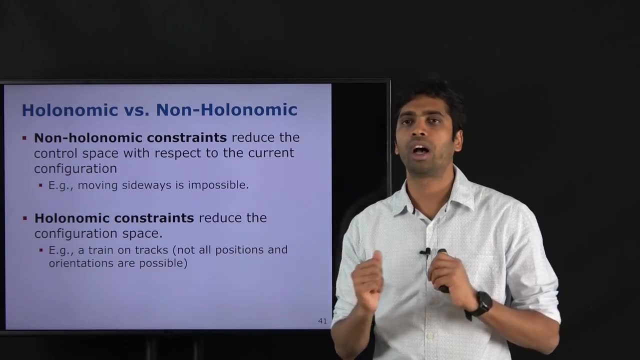 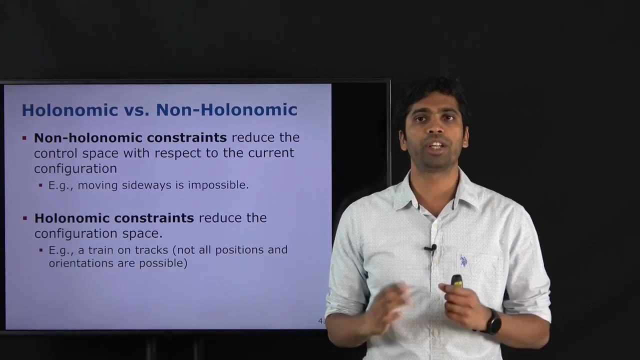 So, for example, if you think of a system which moves on a track, so train on a track, or certain trailer systems where you can attach, say, to your car a particular trailer in the back, and since it's attached with, say, a link, there are certain poses or certain configuration. 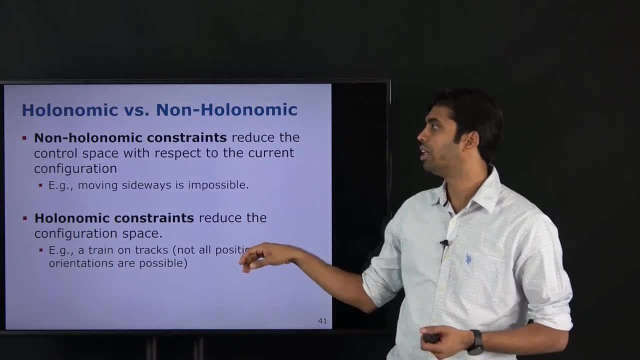 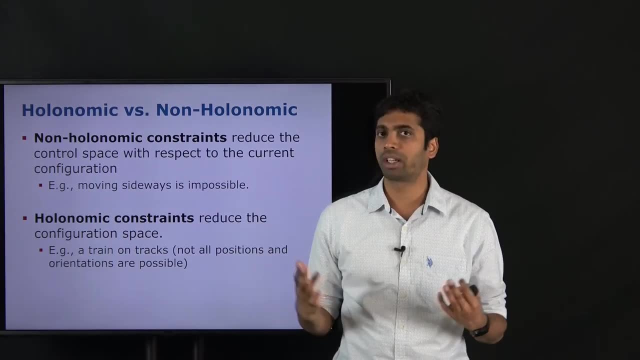 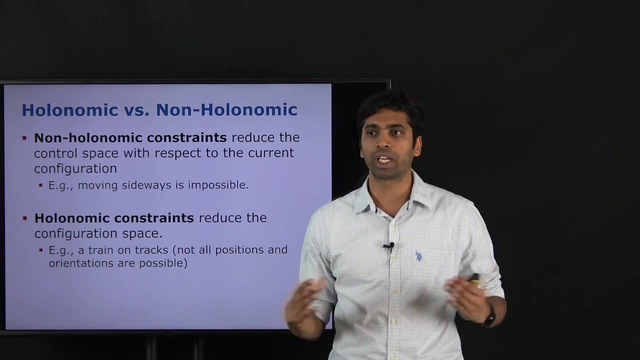 spaces which cannot be reached at all, and such constraints are called as holonomic constraints. Okay, So we have to know, because if we have certain holonomic constraints or non-holonomic constraints, this information is useful, for example, during planning. So if you want to move around in a room with, let's say, several obstacles, if there are certain, 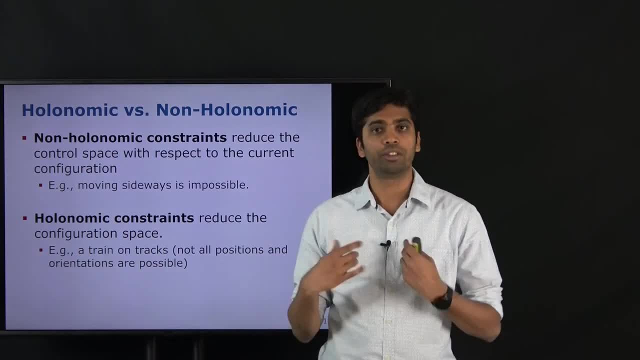 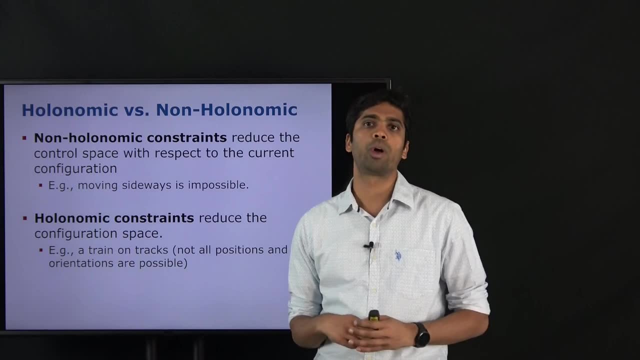 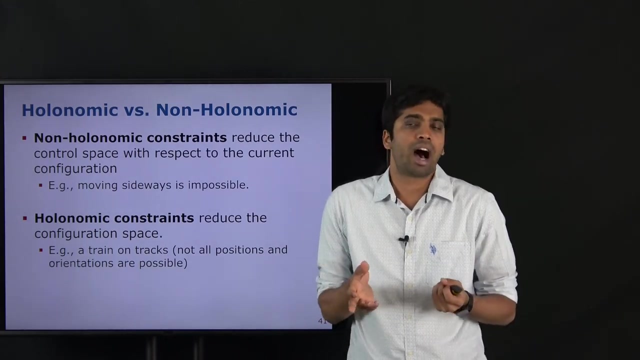 things our platform cannot do, then such knowledge would be useful to have before planning. Of course, if we have a platform which has no holonomic constraints or no non-holonomic constraints, that's the best case. This means that the planning problem itself Becomes much easier, as our platform can essentially do anything that our planning algorithm requires. 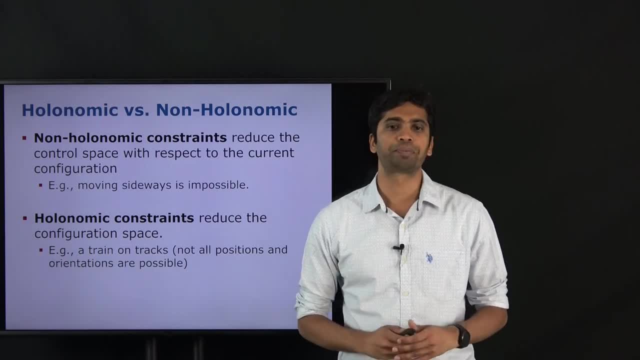 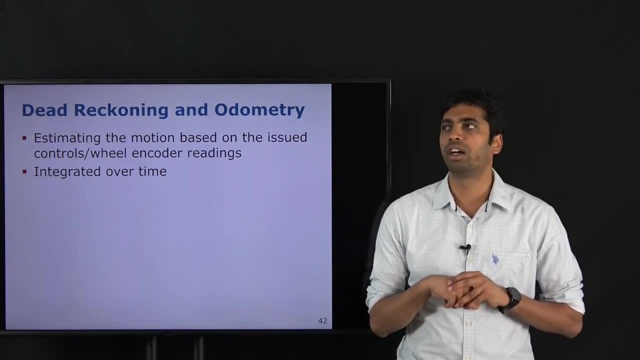 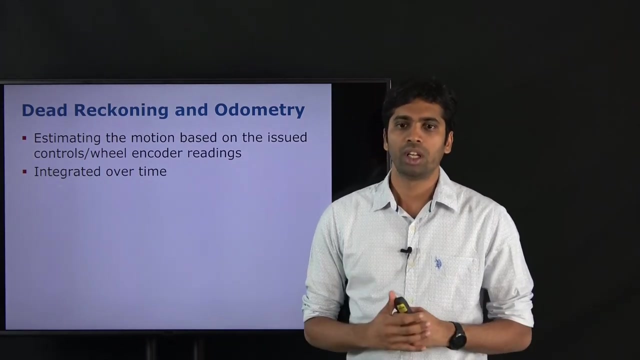 us to do, given that it's a free space. With that, we move to the next topic, which is what is called as dead reckoning and odometry. So dead reckoning essentially means we want to estimate the motion based on the inputs that have been given to the platform. 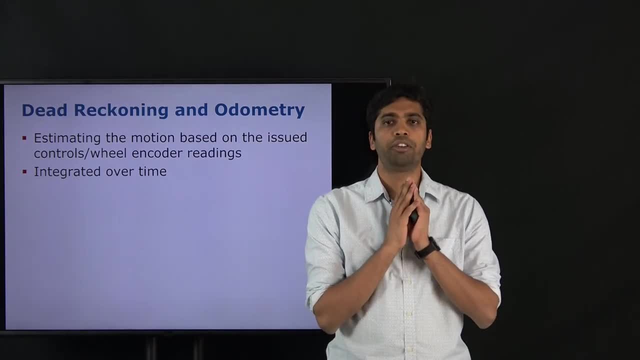 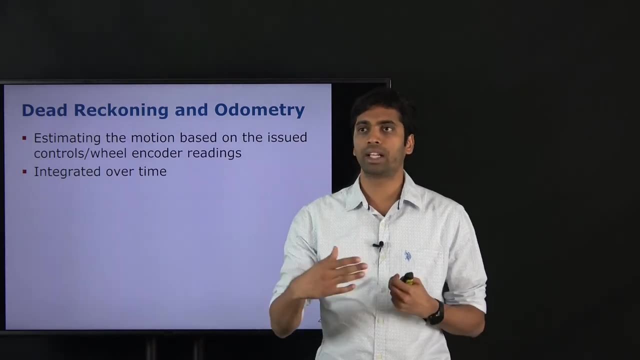 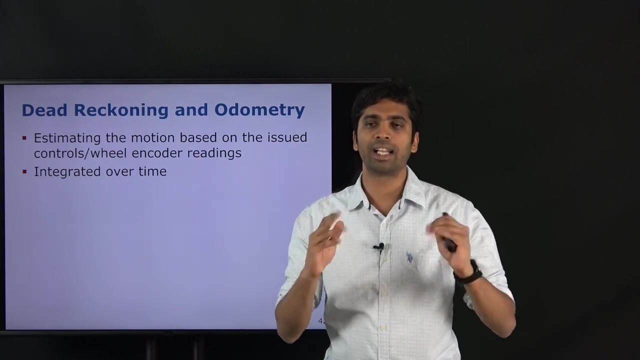 So, for example, if we have a differential robot and we give a certain velocity to the left and the right wheel and we want to estimate how far this particular robot has moved, Of course, in the ideal case, if the robot does exactly what we asked it to do, then this dead. 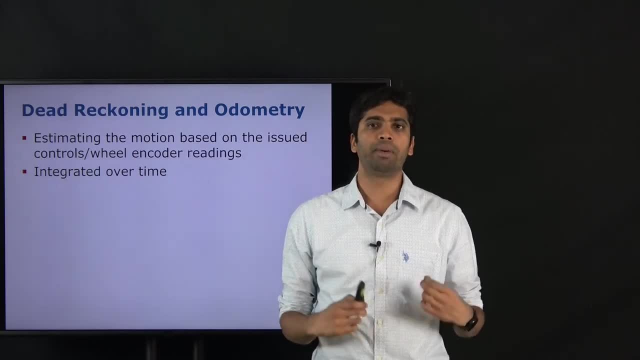 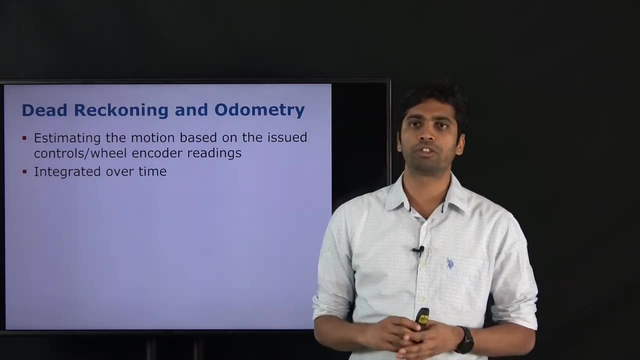 reckoning would be the perfect position of where the robot is, But typically this is not the case. There could be some limits in control, The surface might not be smooth. There's all kinds of conditions which result in the fact that if you just estimate where, 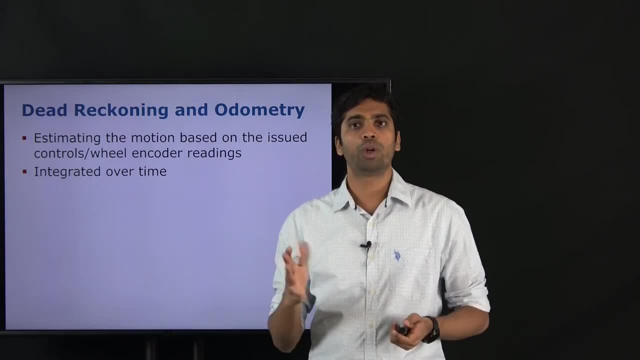 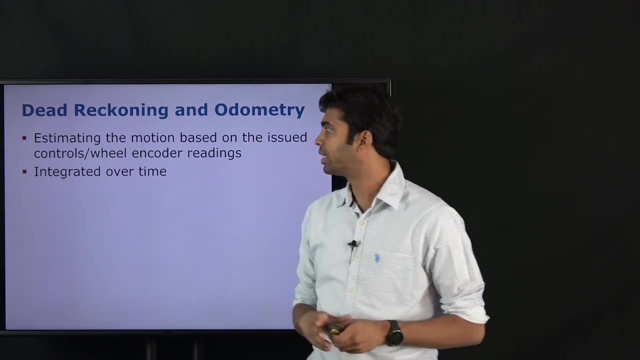 you will be based on the commands that you would give, you would not have the most accurate estimate. So to compute the estimates just using the controls or the inputs is what is called as dead reckoning. So you integrate these commands over time to figure out where you move. 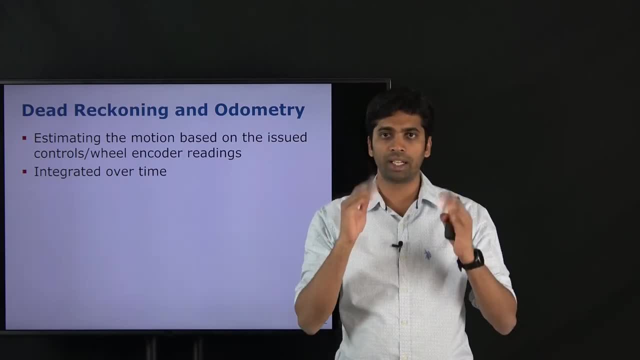 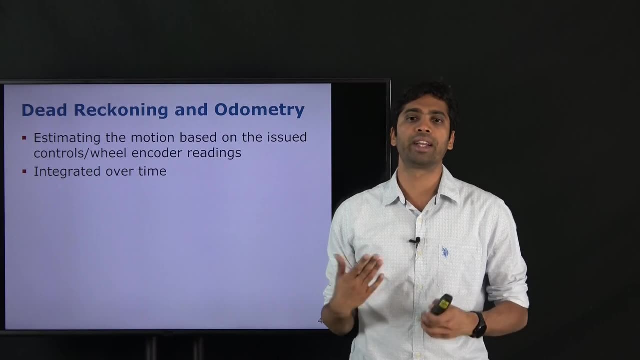 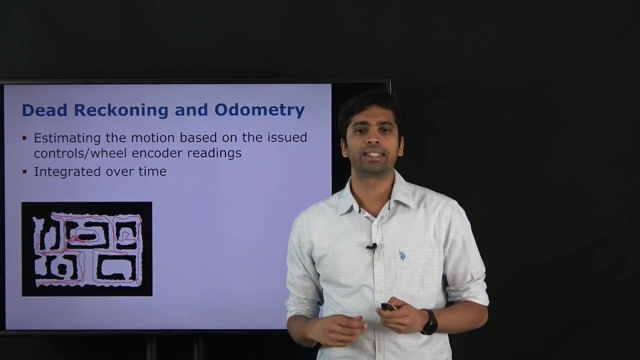 So, for example, if I say I move with a velocity of 1 meter per second for 3 seconds, I would move a distance of 3. And this would be a dead reckoning solution for where you are, Whereas odometry is basically a little bit more, which means that you actually have some. 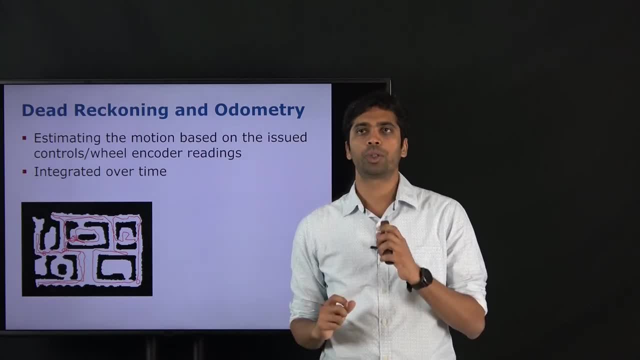 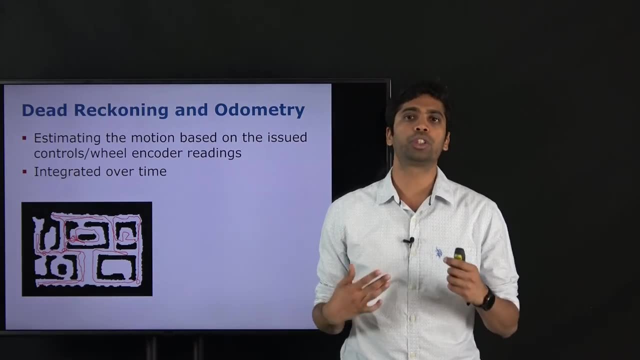 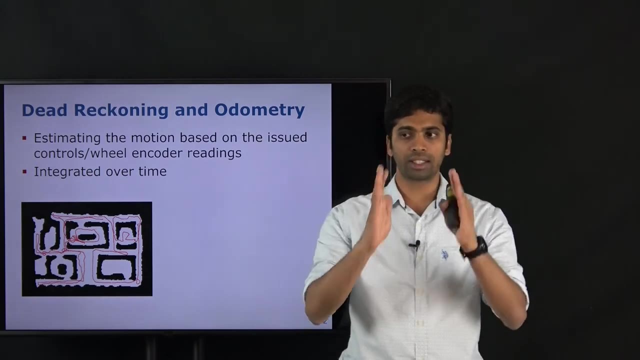 kind of encoders on your wheel, So these count, for example, the number of revolutions that your wheels make, and you use these revolutions to figure out how much you move. So since this is kind of a feedback on the movement that you make, So say you ask this question. 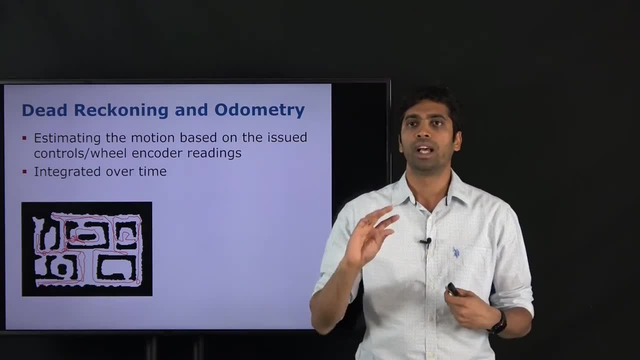 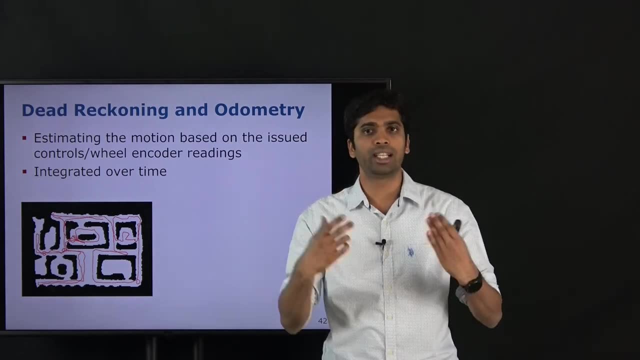 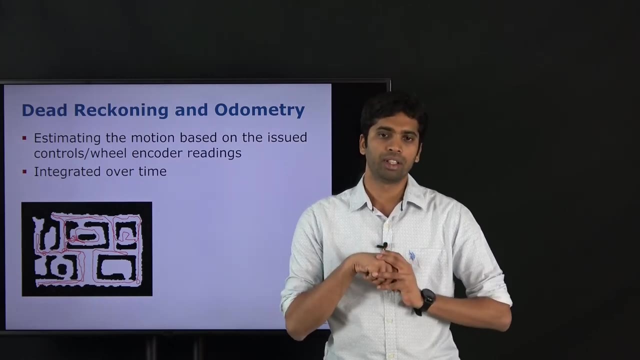 Ask the wheels to rotate at a certain velocity. Maybe the wheels didn't rotate at that certain velocity. However, since you recorded how many revolutions the wheels actually did, typically odometry measures end up being more accurate than a dead reckoning kind of estimate. So here's a simple example to see how this odometry looks like. 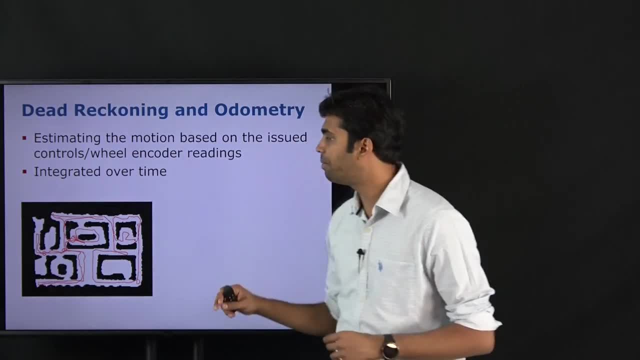 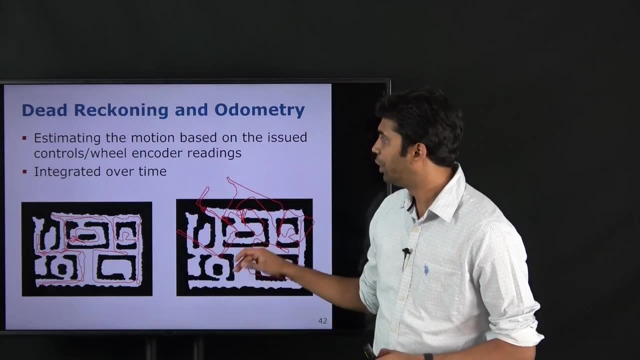 So in this case, what we see here is kind of a maze environment in which a robot is moving. So this is how the robot actually moved. However, due to some errors in the odometry, so there's some kind of a systematic error, it seems, here towards the right. 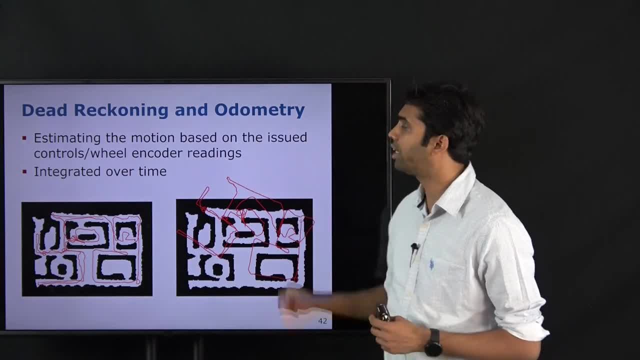 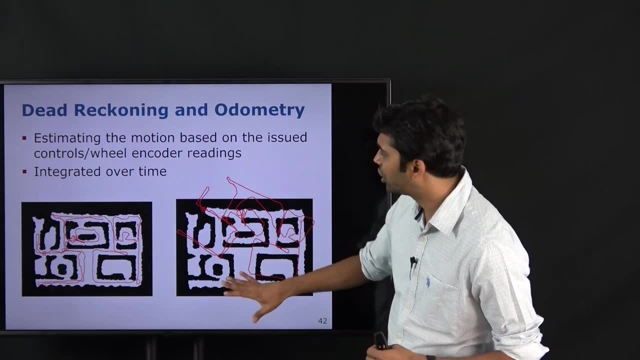 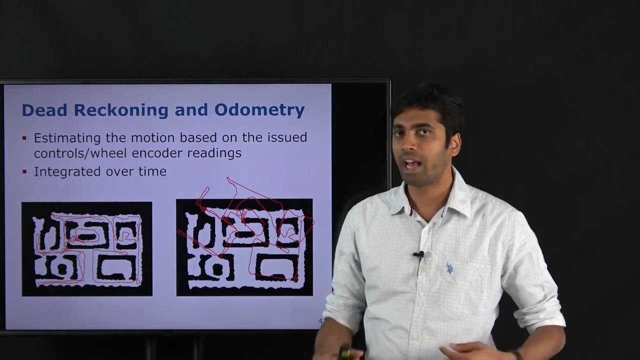 This is what we expect, or this is what we estimate our robot to have done. In this case, there is a systematic error to the right and therefore, at each term, we have this drift that accumulates over time. However, given the odometry sensors that we have, this is what we got. 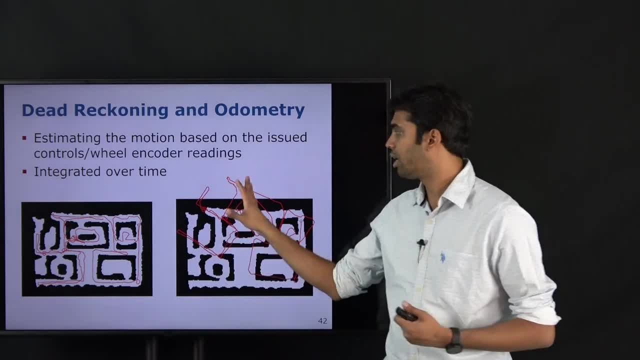 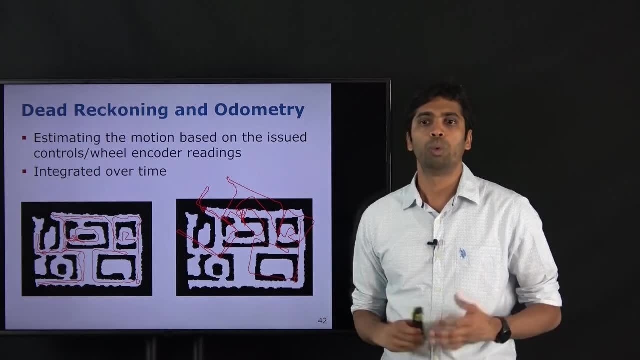 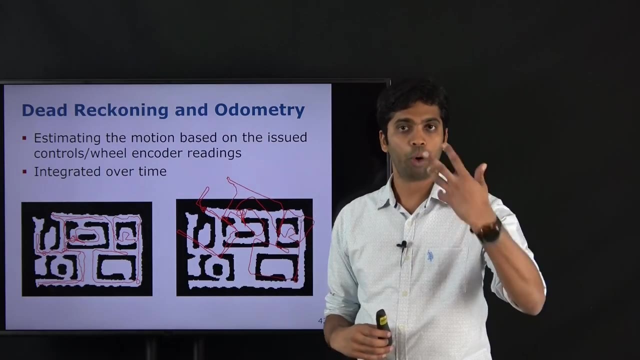 So this is probably a quite noisy sensor. Therefore there's a large error because, depending on the quality of the odometry sensor or the of the encoders, we might have better or worse estimates. Either way, dead reckoning and odometry are a way to estimate the motion.